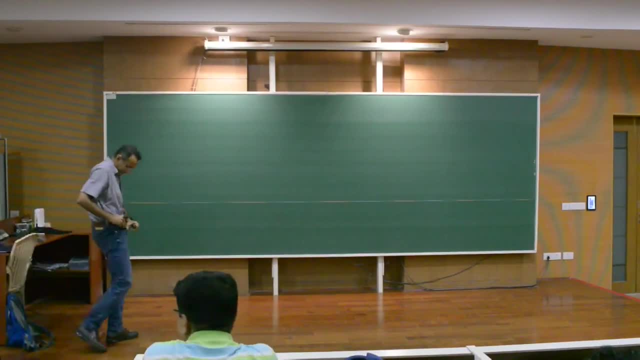 Professor A Raghuram, Thank you for this introduction. It's a very good idea that you're starting this series. So somehow the job is to give you an idea of what is research about. I don't know if I'm really so qualified. I mean, I don't suffer from false modesty So I am a researcher. 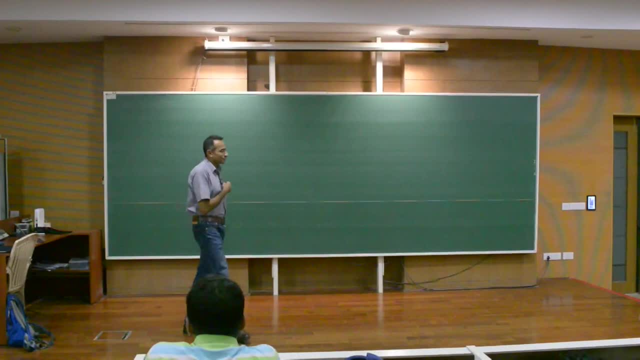 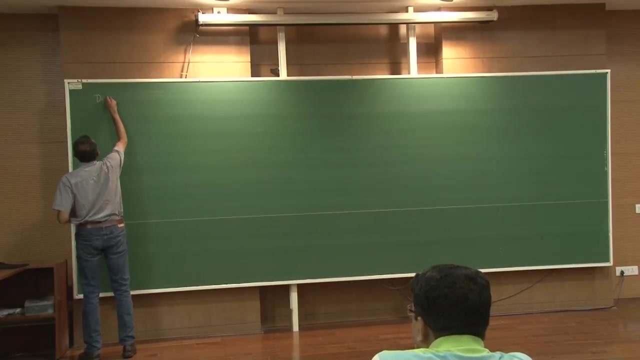 and then you go to an important center for mathematics like the Institute for Advanced Study and then you see people like Delene And then you wonder: you know what am I doing? kind of thing. But nevertheless I have something for all you guys. Let me just write it out. 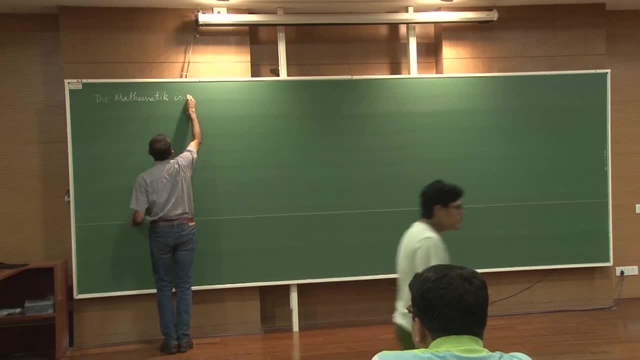 And then I'm going to tell you what I've been doing for a long time. But you know what? I've been working on this in my own office. I don't think there are any words in the papers. A Raghuram. 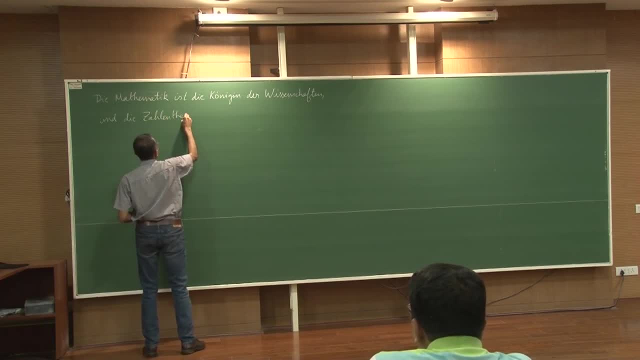 I love this, Professor. A Raghuram Adelman, You're going to go to a lab today. A Raghuram, You're going to be a foreman. A Raghuram, I like that. 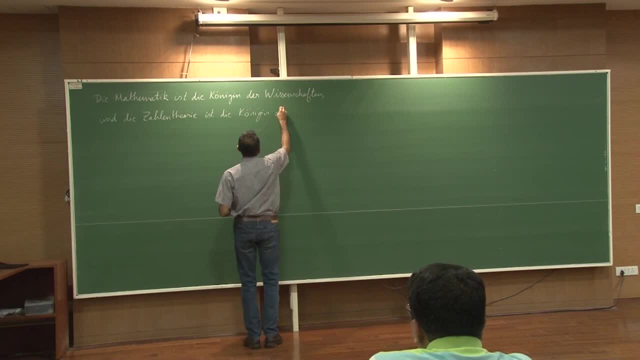 Professor A Raghuram A Raghuram, Professor A Raghuram. Die Mathematik is die Königin der Wissenschaften, und die Zahlentheorie is die Königin der Mathematik. 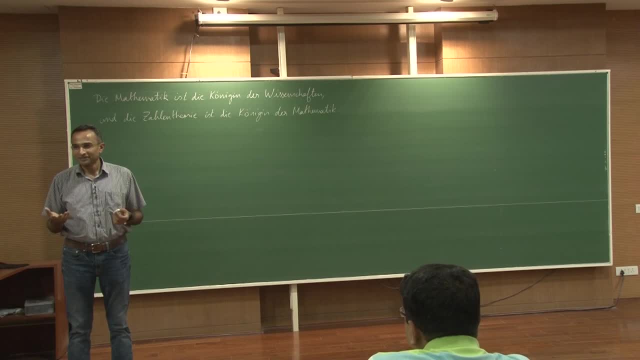 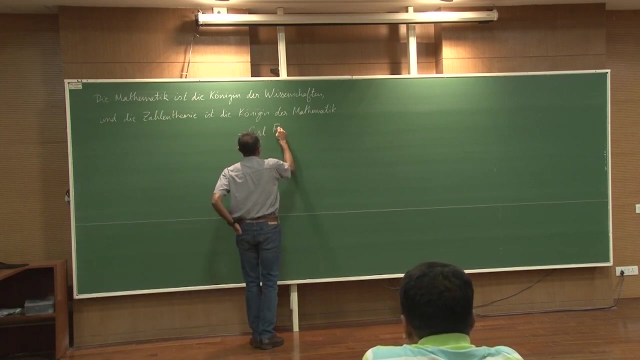 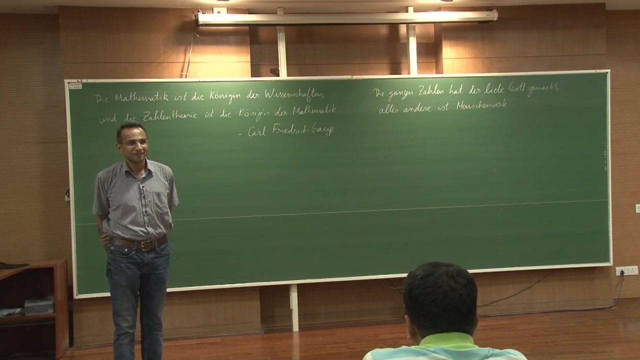 You can guess what this might mean. anyone. Mathematics is the queen of the sciences and number theory is the queen of mathematics. Who said this? Carl Friedrich Gauss, or just Carl Gauss? I have one more, The. Can you guess what the sentence means? 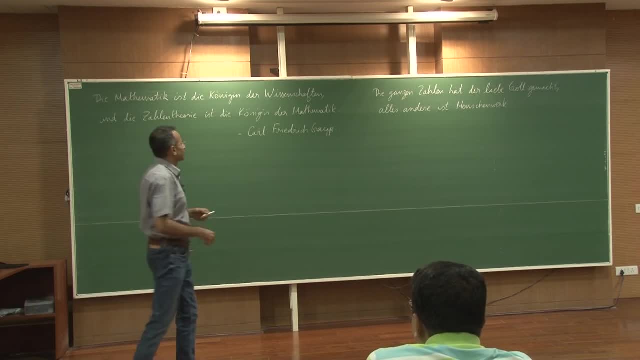 One of you, just The is a set of all numbers. literally, I mean integers is the work of the dear God and everything else is man's work. Who is this quote usually attributed to? You can't hear me. I can hear myself very clearly. 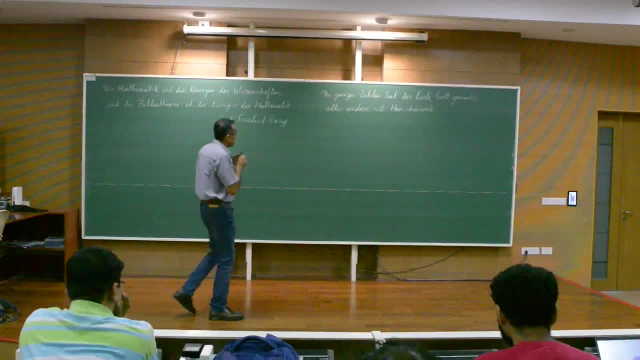 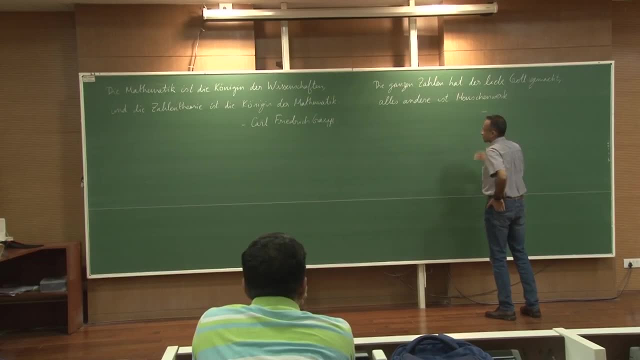 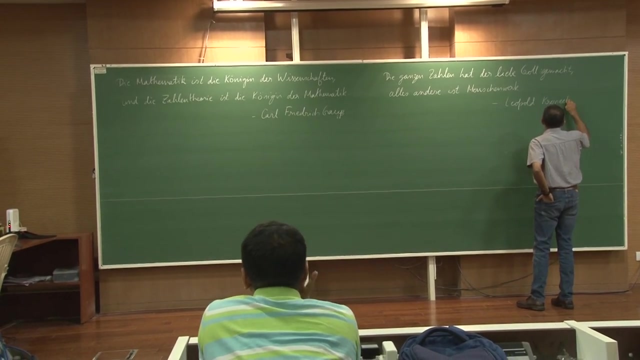 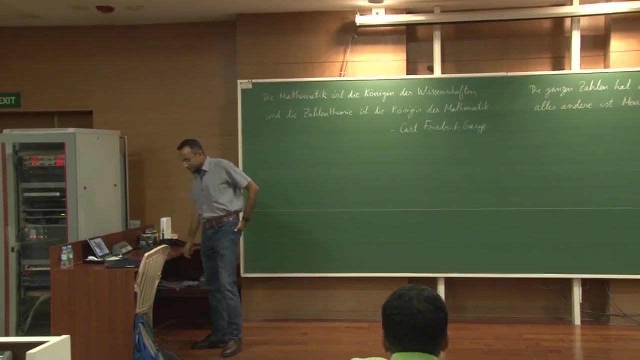 Okay, we start again. the mathematic is the no. no, So the God is okay. so this is whose quote is Kronika? what was his first name? Anyway, this is just to To kind of for me to warm up and for you to warm up. 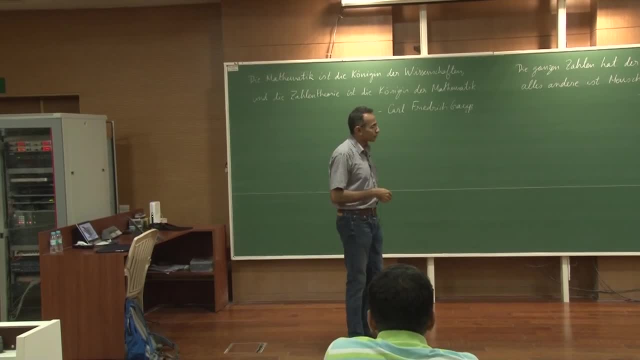 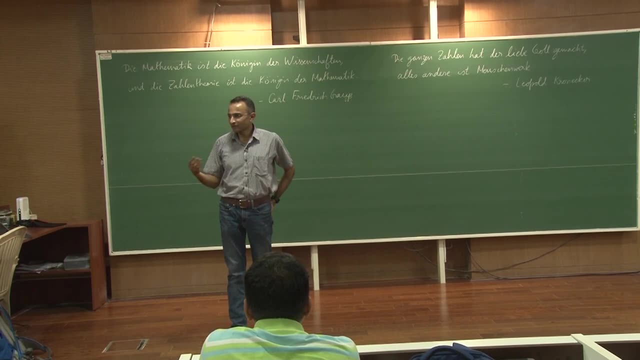 So I have given a title. I was going to say a pompous title, but the pomposity, or being pompous is forced upon me by the series itself. What is something? what is number theory? You see, any such thing is very vast. 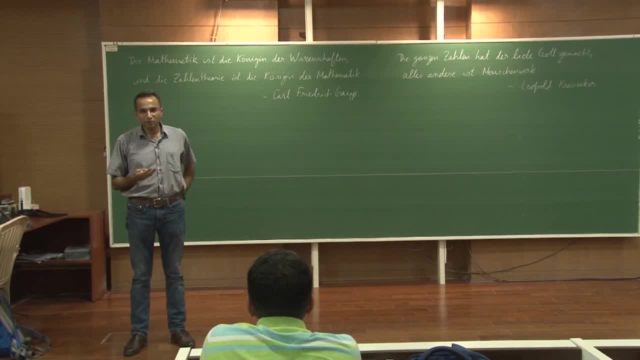 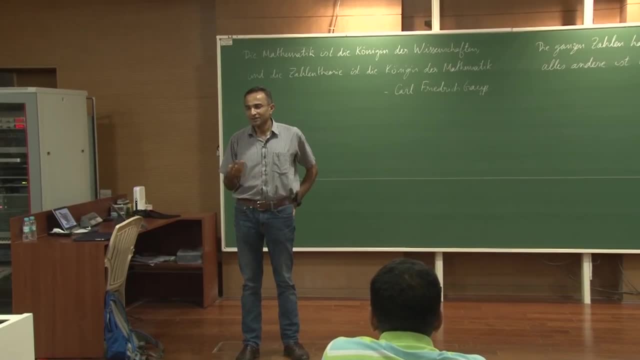 You have to understand, I can be at a conference on number theory and a fellow number theorist. so I fancy myself a number theorist now And a fellow number theorist. A fellow number theorist might be there and we might have nothing to talk to each other. 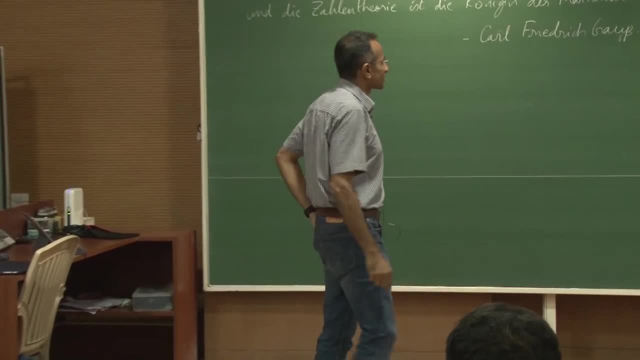 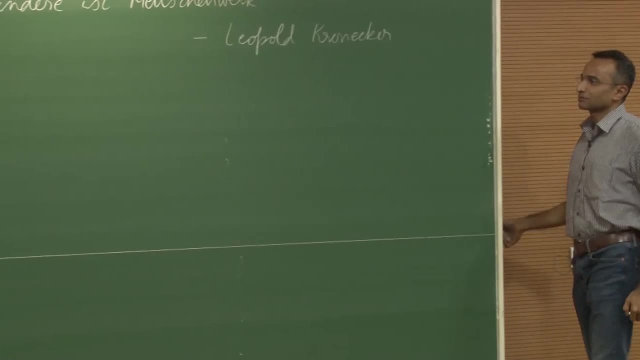 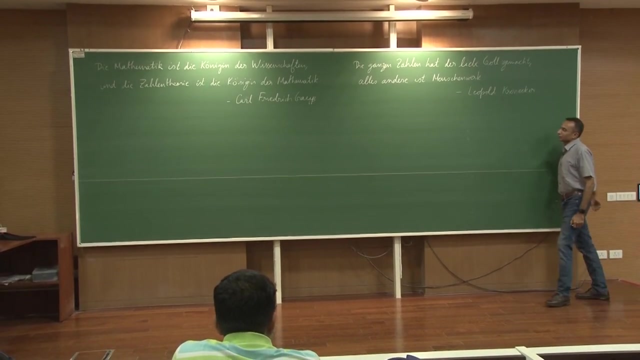 other than you know, the beer was good, or this is good, or whatever. you know, It's a very vast. I suppose any one particular, any subject is. it's in the nature of human knowledge, I suppose the vastness. 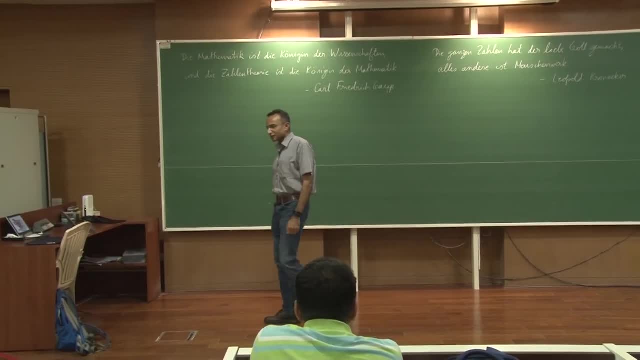 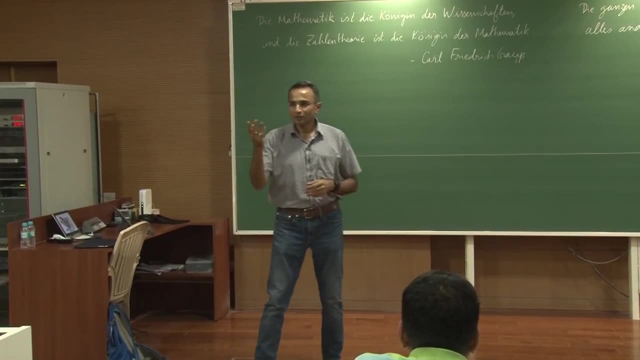 Anyway. so I will weave some storyline about number theory and hopefully you get something out of it, The okay. I'm going to stop here, Okay, So I wanted to have some idea. I see some PhD students who I'm familiar with. 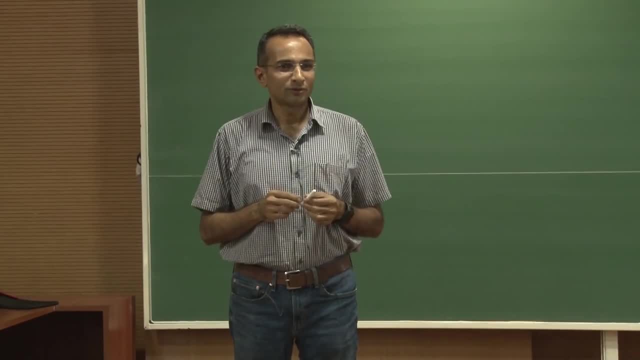 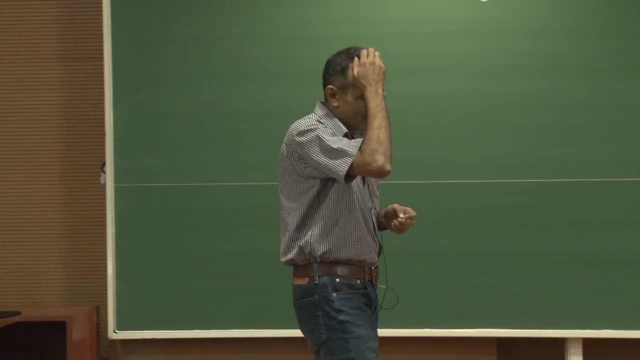 Do we have first year BSMS students here? Yes, Oh, Very good, Let's move on Second year, All right. So so you see this also. this is very good that you guys are here and hopefully at least 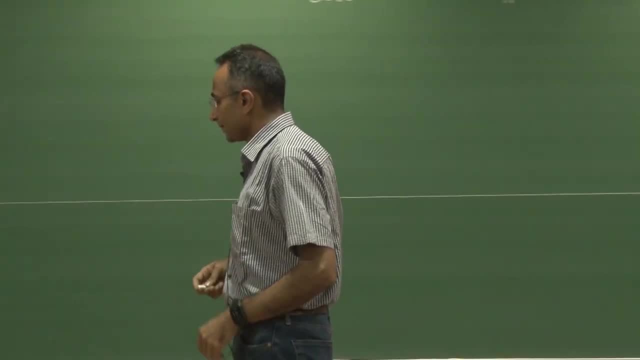 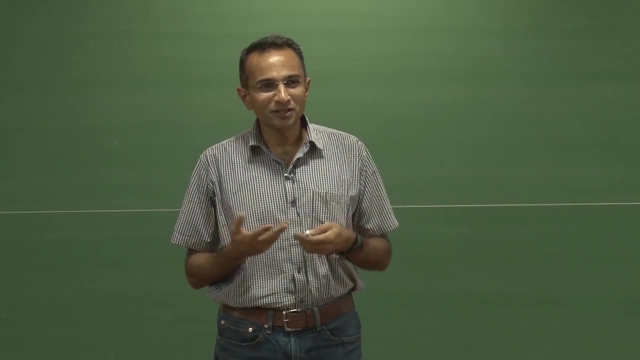 one of you will go back home feeling a little inspired, Anyway. so yeah. so what I was going to say was: I'm- I start with an apology that one is constrained by This language of mathematics. you see, you just come out of school. you're kind of in. 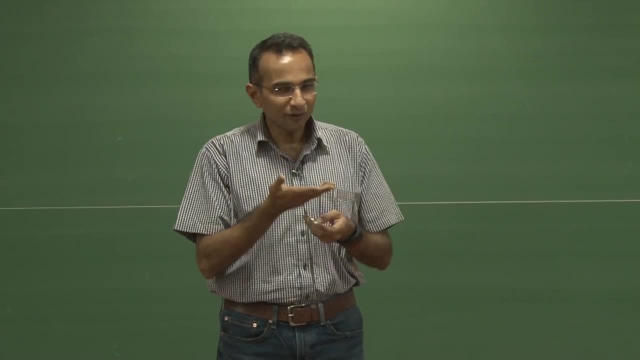 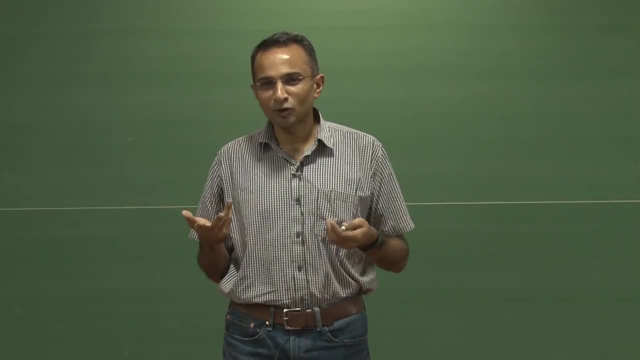 some seemingly fancy place and it takes a while to. if I start talking about, you know, take a hospital automorphic representation, it means nothing at all to most, and probably not much to me either. So there's a certain this whole business. there's a lot of language. 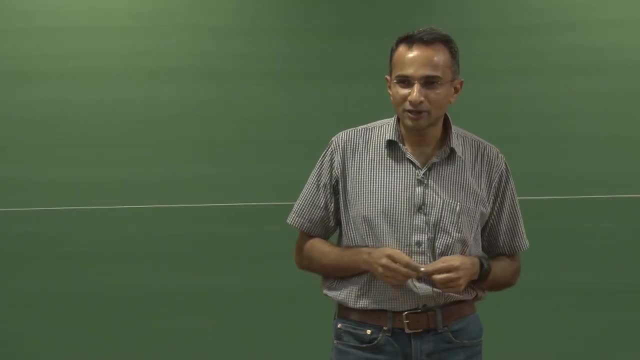 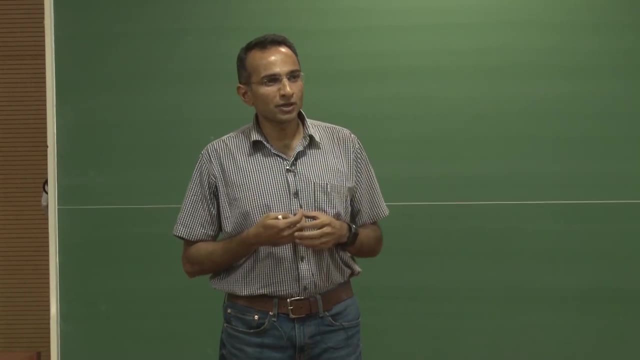 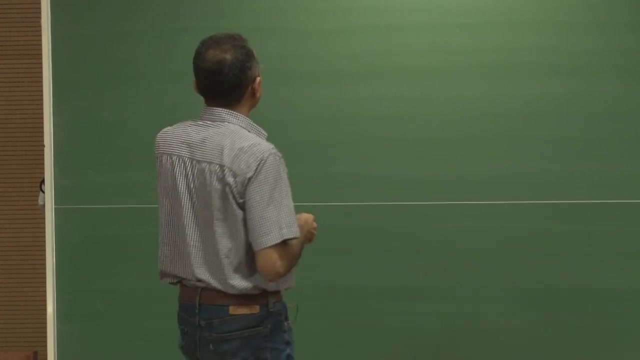 It's. you know, mathematics is the language of the sciences, as Galileo had once famously said. So I'm constrained. It's the fact that, you know, many of us in this room are unfamiliar with the language of higher mathematics. So, at the level of basics, I still want to, you know, trigger some thoughts anyway with 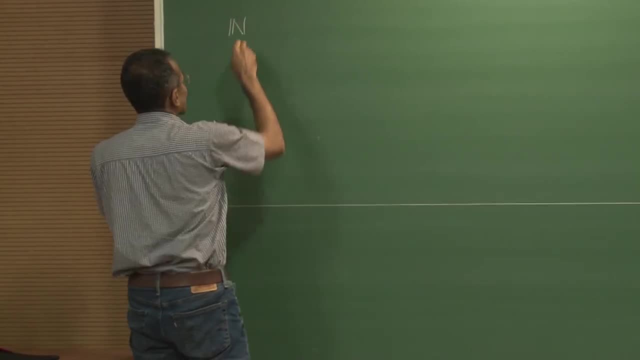 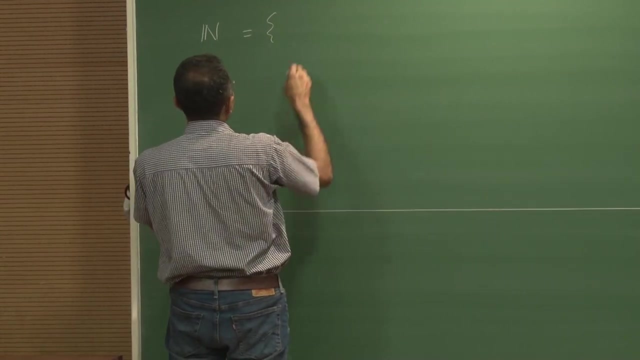 that apology. So let me just get started. Of course, as Kronecker said, all God made the numbers and everything else is the work of man. We start with natural numbers n, which is a set of all these positive integers and. 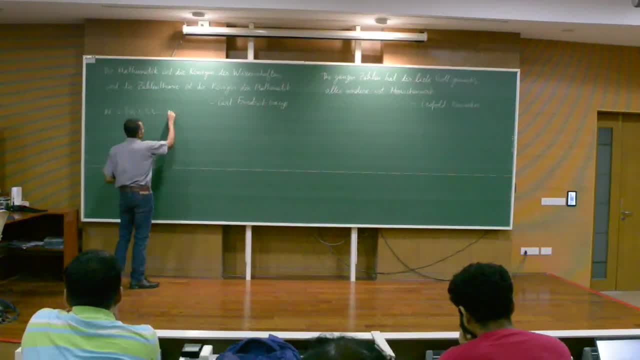 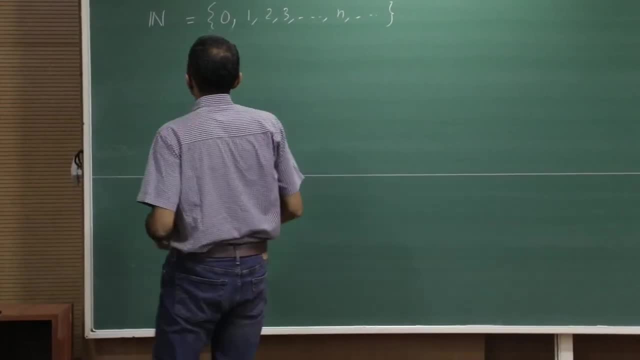 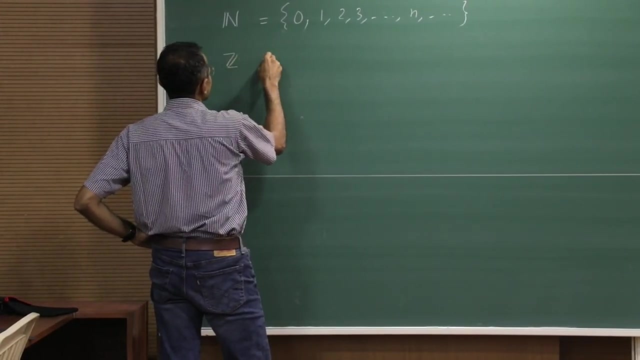 this is, And Burbaki- notation zero is included there. Go look up Burbaki, Nicholas Burbaki, And then, well, you can't live your life here. You know, even if you wanted to do some bartering, you need negative integers. 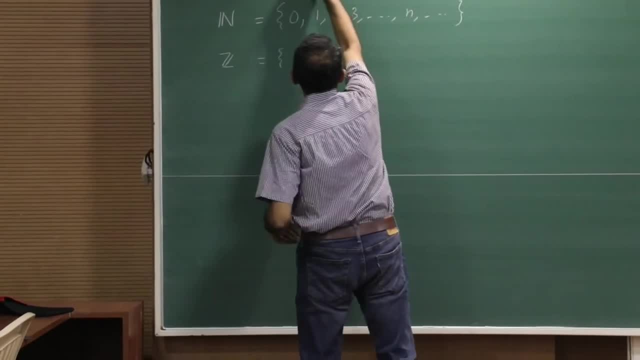 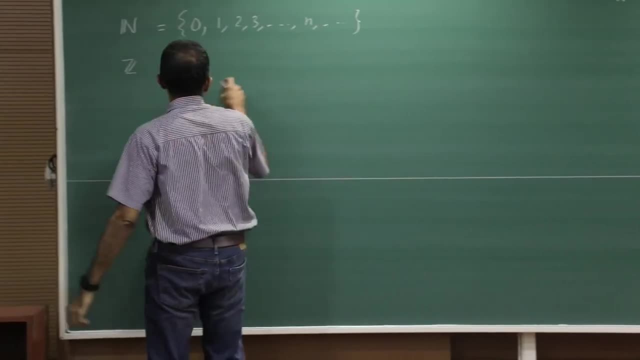 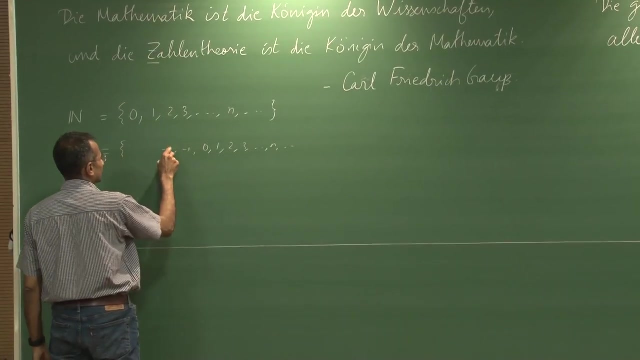 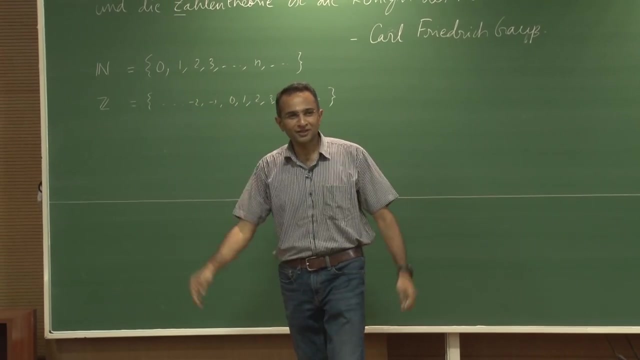 And one often denotes that by Z. The first letter of the German word for number is Z, And this is all integers. So So what is number theory? Number theory is the study of the set. I'm done, Let's get dinner. 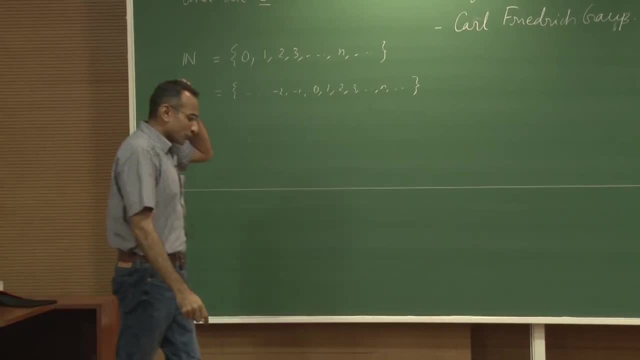 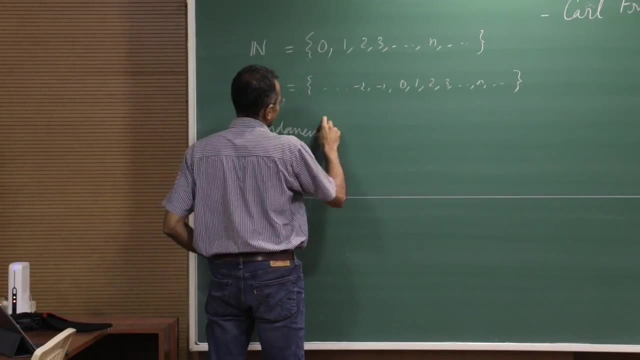 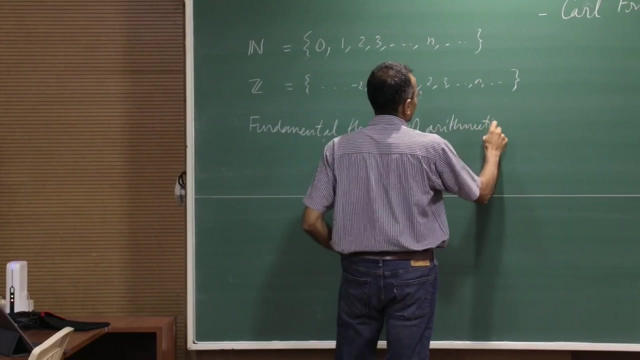 OK, so we get started here, and then you know, all of you would have certainly seen what's called the fundamental theorem of arithmetic, OK, So. So, the first thing is that every integer, which is a statement that every integer I 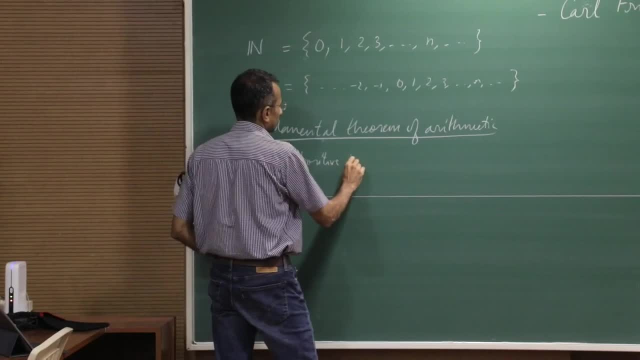 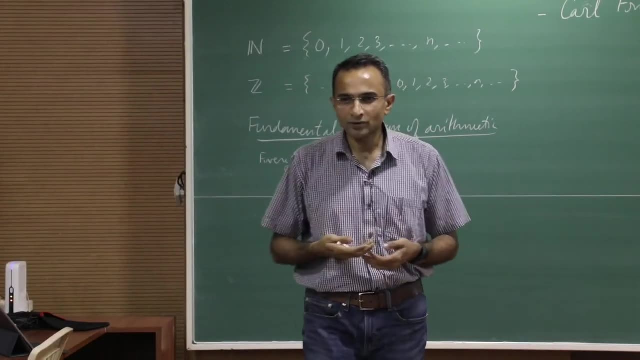 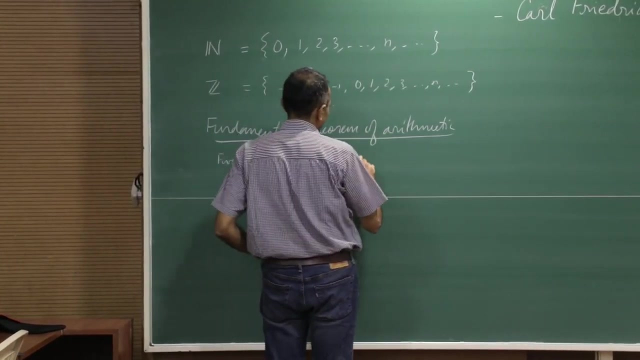 might just say positive integer. You know, take a number like six. I can somehow pull it apart as two times three, But two and three itself. I can't further factorize it in terms of integers. So every positive integer is And. 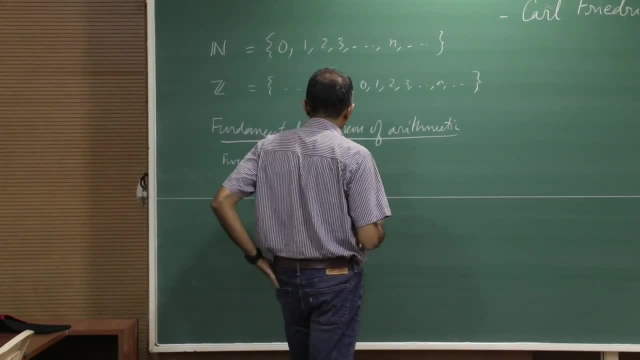 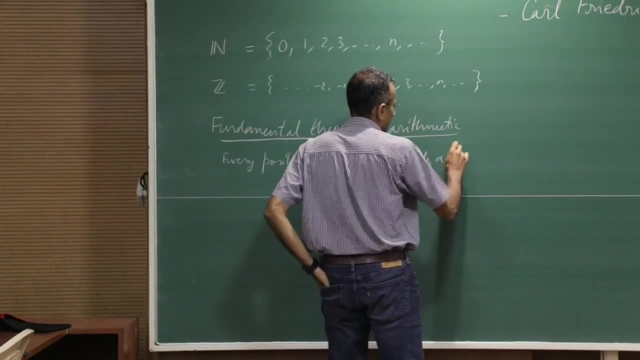 So every way six, I can write as in decomposable integers, which is called a prime, And that's unique: It's six is two times three. So more generally, every positive integer is uniquely a product of primes. So let's start here. 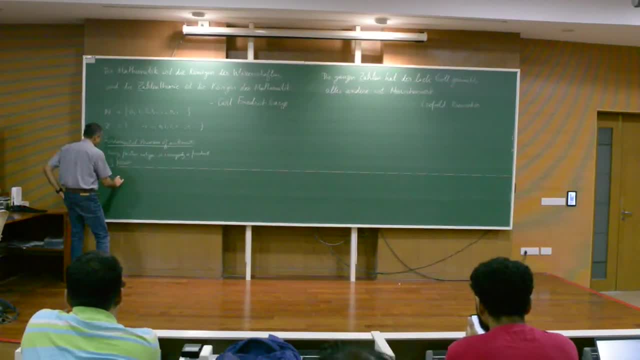 I've used the word prime, which I know is done in high school mathematics. So what's prime? Prime is the. A positive integer is said to be a prime If it's only divisive, Right. So the integers are one in itself. 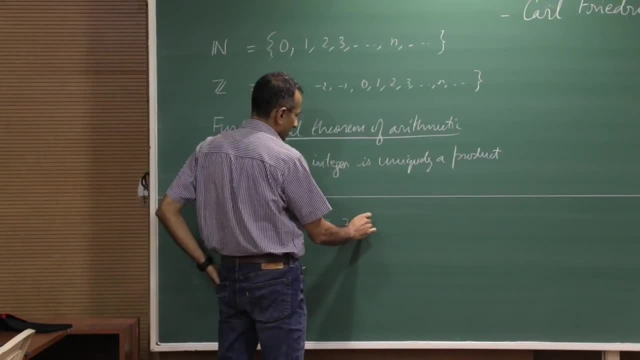 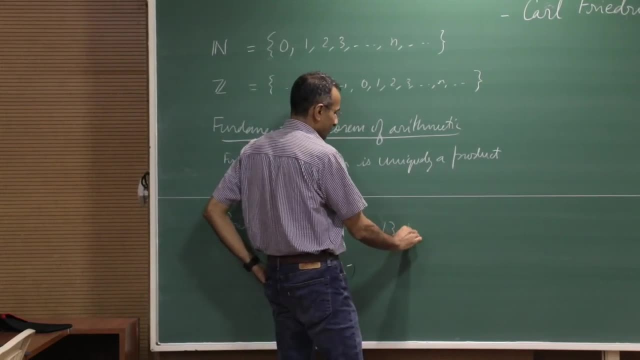 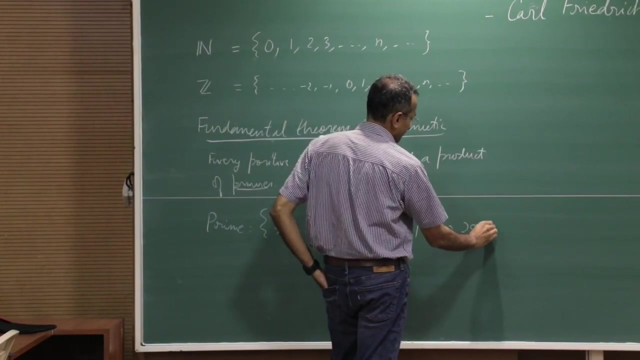 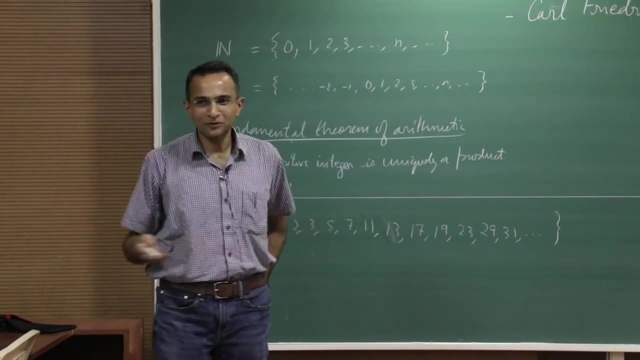 And then you know that the primes are two, three, five, seven, nine, 11,, 13,, 15,, 17, and so on. Typical math dating is, you know, you mug up the first so many primes and there used. 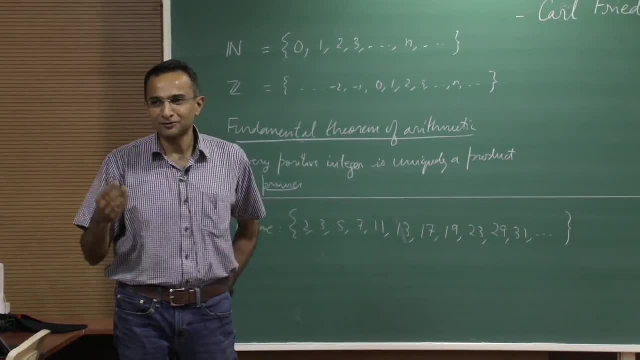 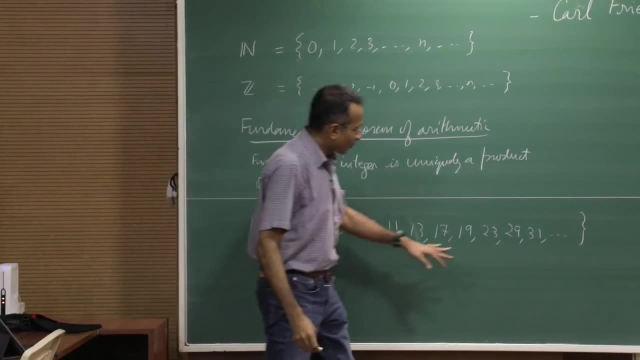 to be a prime number B in our mathematics, And if you have learned the first 200 primes, you might actually go back home with 500 bucks or something. So in any case, I've already fudged a little. I've just put a dot dot dot. 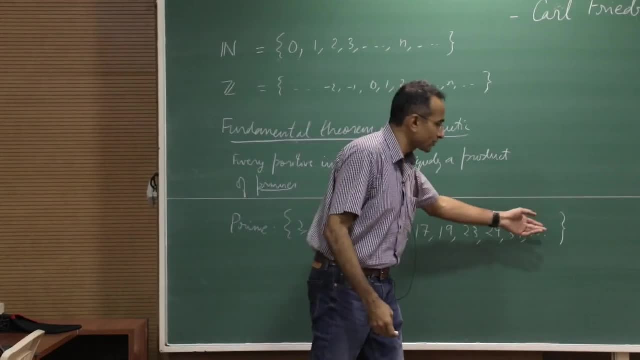 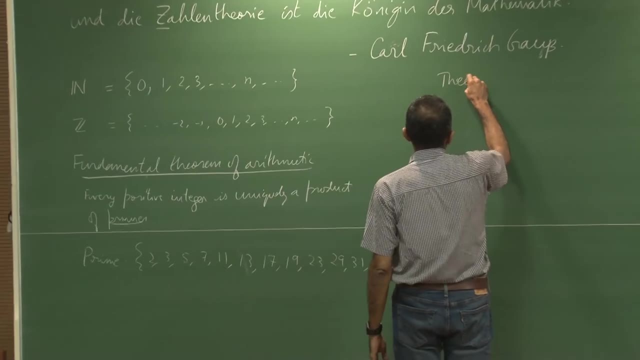 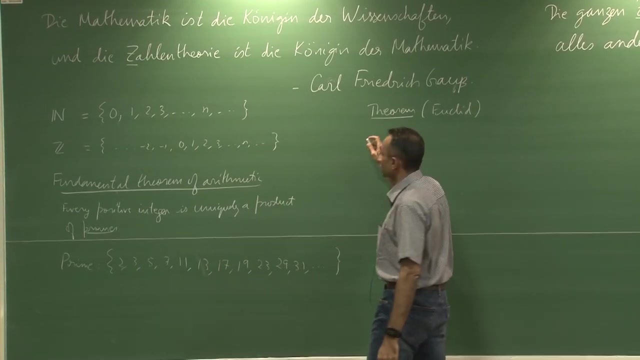 And the question is: well, does this set kind of finish up somewhere or not? And this is probably the first major theorem in number theory. This is a theorem going back to Euclid. What is the set? What is the set, The Euclid theorem I'm going to put down. there are infinitely many primes. 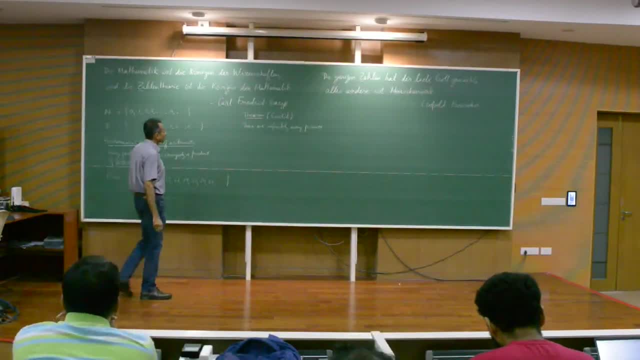 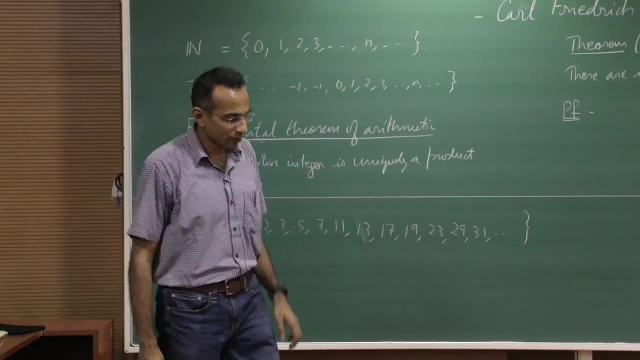 And I think everyone should know a proof of Euclid's theorem. Euclid's theorem will justify my dot dot dot here. So what's the proof? This is the first proof. This is the first proof. This is one of the most famous proof by contradiction. 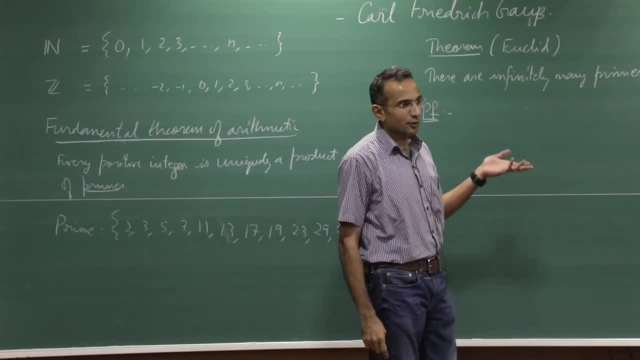 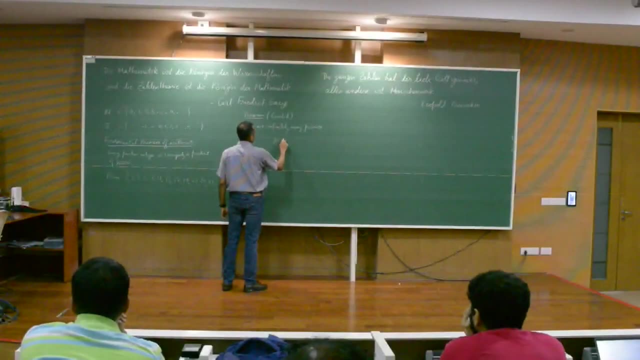 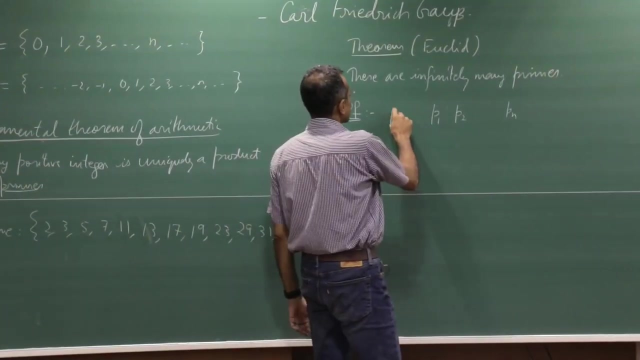 I'm sure many of you know this. Suppose, not Suppose, there were finitely many primes, Call them something P1, P2, through P, something PL. I don't want to put commas, but suppose this is all the primes. then you consider an integer. 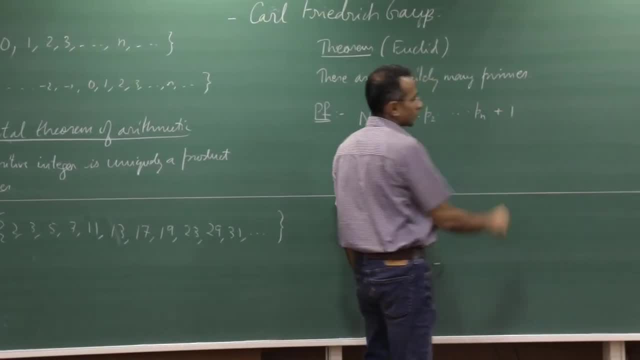 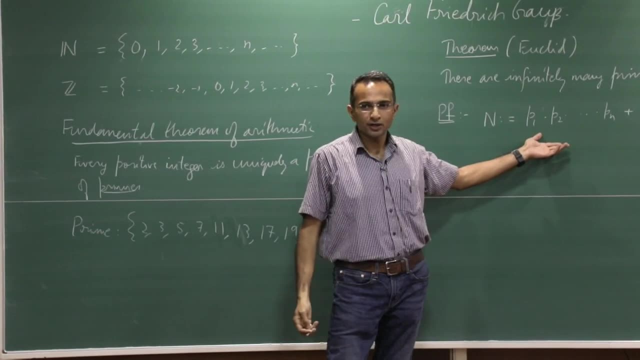 n, which is a product of these guys, and you add 1.. So this is a positive integer. Either it's a prime itself or not, It's a positive integer And if it's a prime, in any case there is a prime which divides it. 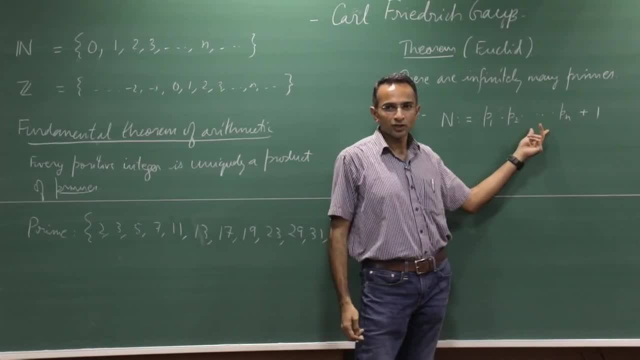 And that prime needs to be. since this is a set of all primes, it's got to be one of these PIs. But then it divides n. It divides if it's PI. it divides the first sum and therefore it divides n minus this. 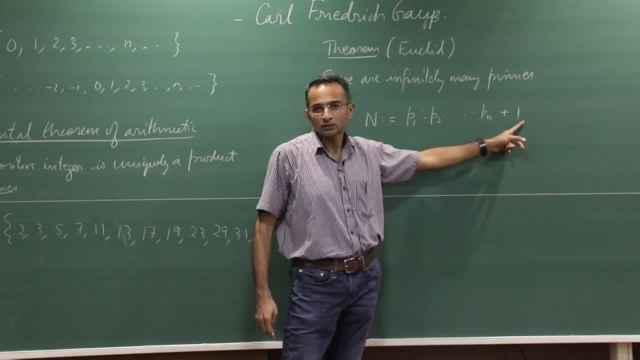 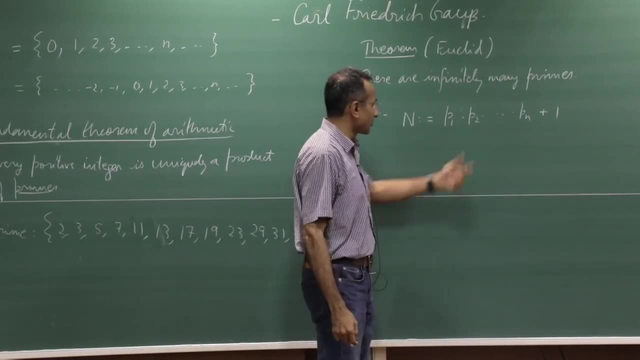 In other words, it divides 1.. But 1 has no prime divisor. None of these guys are going to divide 1.. So you kind of dig yourself into the hole by the supposition that there were only finitely many primes. 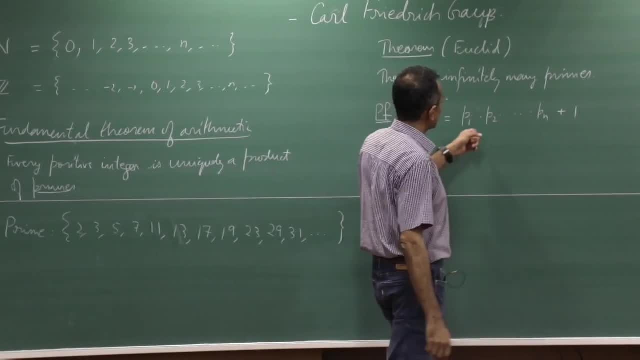 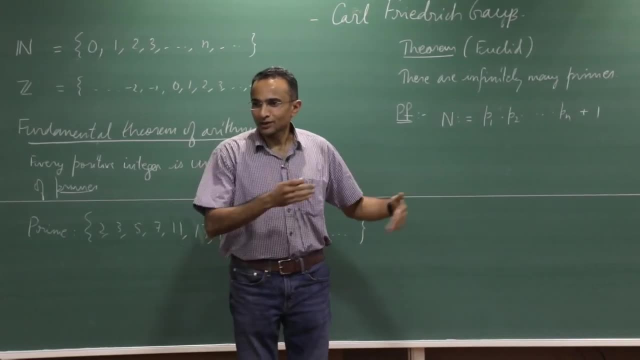 In other words, Yeah. So if that assumption is wrong, this is the proof by contradiction. So the essence is just this construction. Let me consider this. You can fill it out, OK, I'm not giving a course here, Just the essence of the proof. 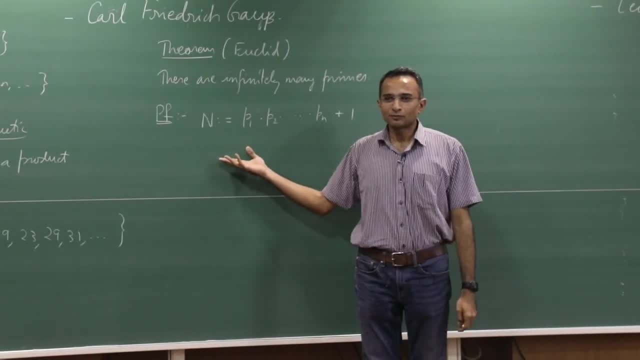 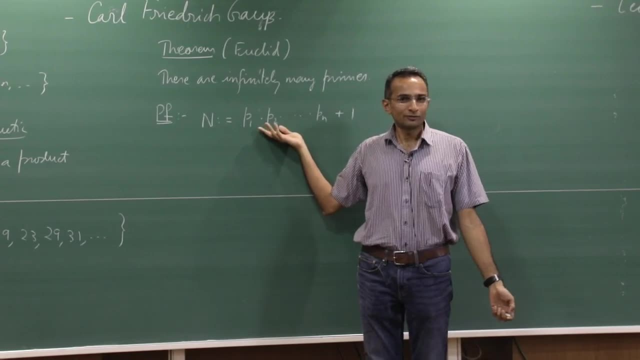 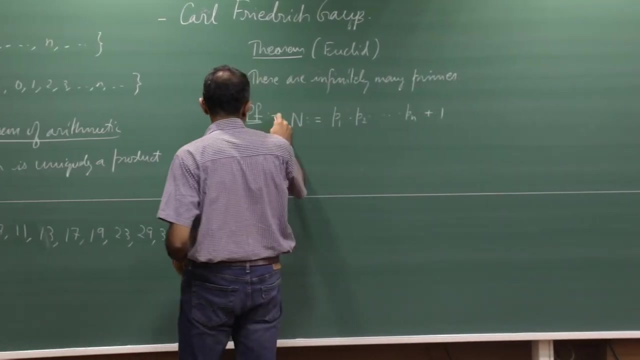 Let me do some other proofs. So this very likely don't feel embarrassed. How many of you have seen this proof? So I like to say almost all, OK, Let's play around with it. So this is proof number one. Consider: 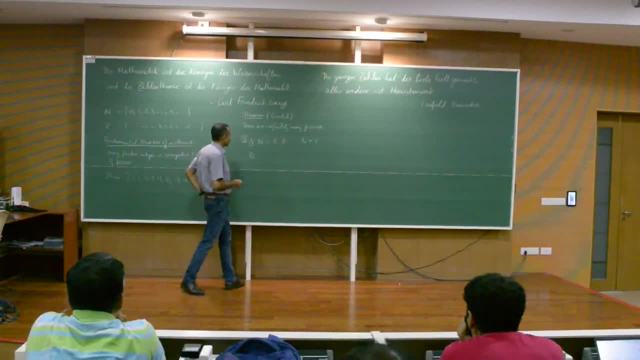 So again it's kind of. It's almost like a proof by contradiction, It goes slightly differently. So suppose P1 to P, let me say L of n are all the primes less than n. I'm going to do a little his. 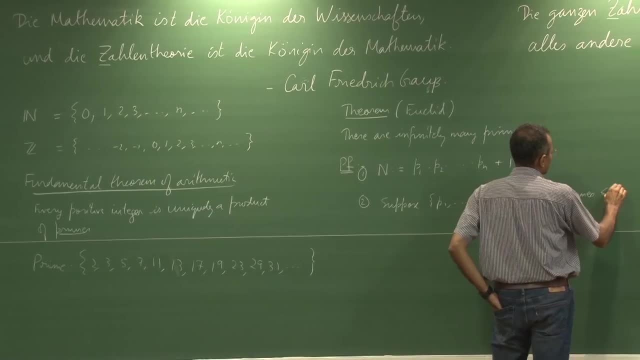 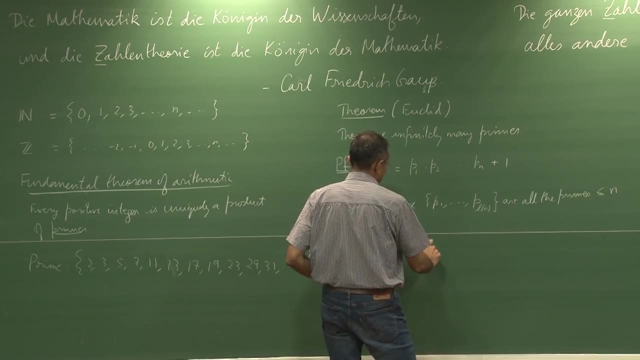 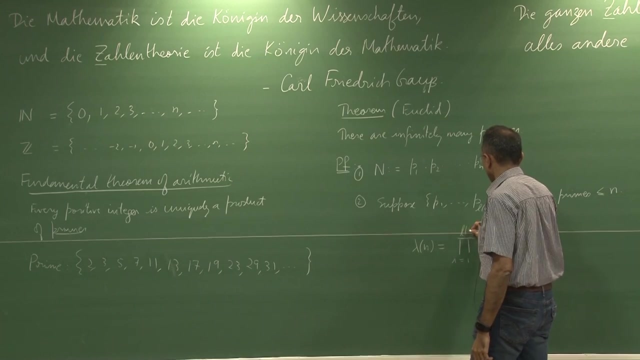 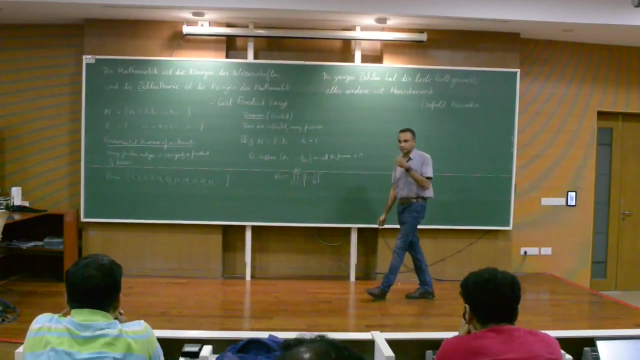 I don't know what the other answer is. Maybe I can do this. Oh my God. less than equal to some integer n. And consider now this quantity: lambda n. lambda n is the product of i going from 1 to this L of n of 1 minus 1 over p, i inverse. Consider this: 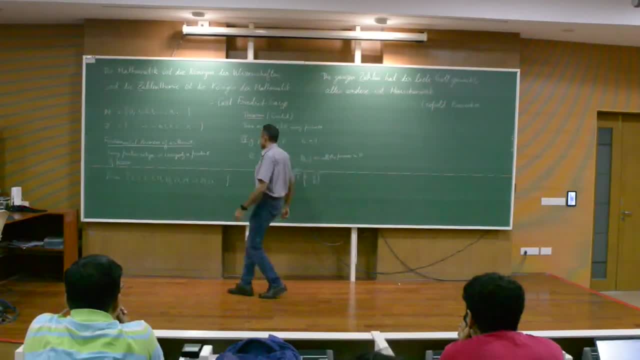 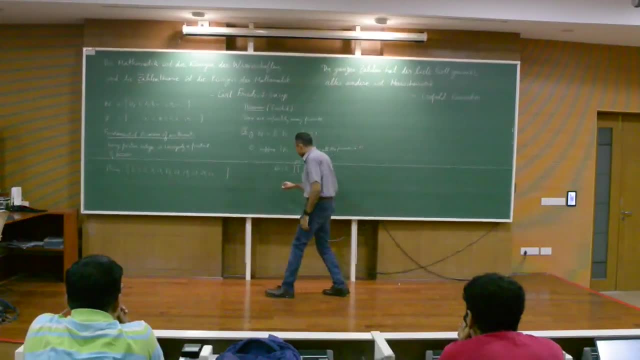 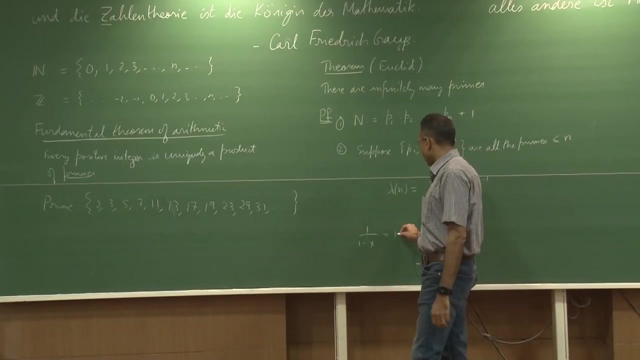 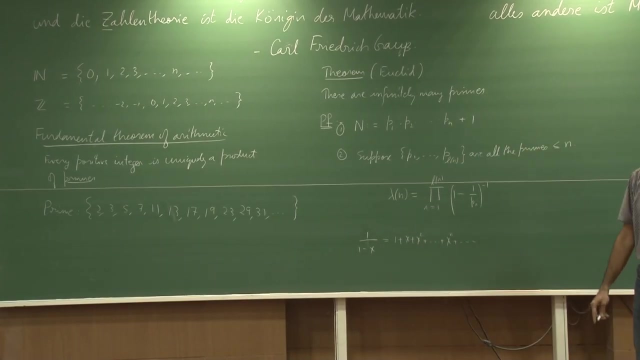 What kind of quantity is this? Well, you have done your geometric expansions: 1 over, 1 minus x. if x is small, you can write this as 1 plus x plus x, squared plus dot dot dot x to the n, plus dot dot dot. This is an exercise. I can do this. This inverse is really 1 over. 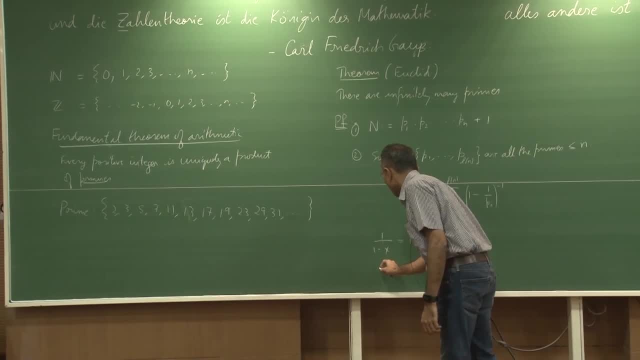 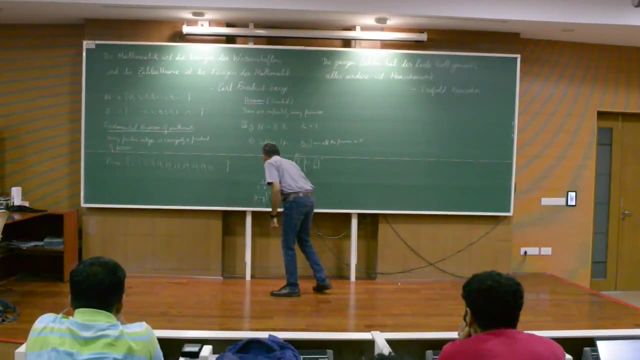 1 minus. So if I were to take x as 1 over a prime, this looks like 1 minus 1 over p. this guy inverse looks like 1 plus p plus p squared plus all powers of. So this n is. 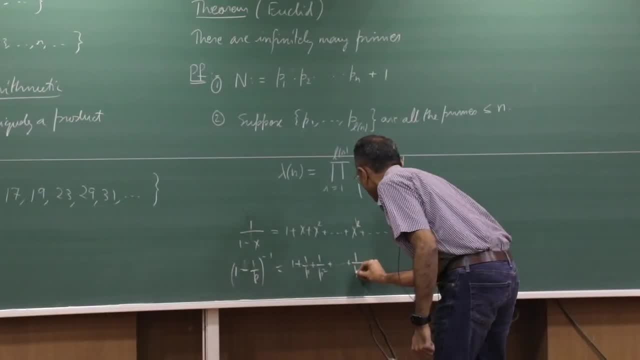 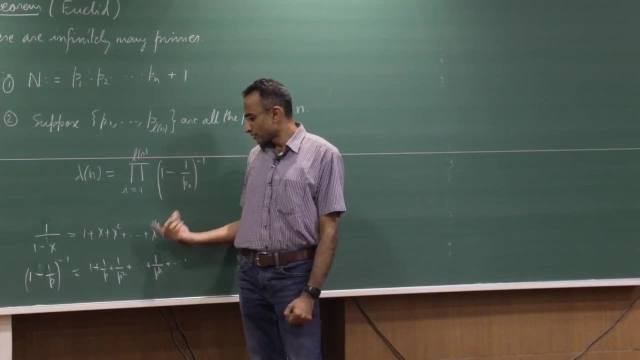 not that n, Maybe I'll make this a k 1 over p to the k, plus dot dot dot. So what does this finite product represent? So every factor captures the sum of reciprocals of all factors. So every factor captures the sum of reciprocals of all factors. So 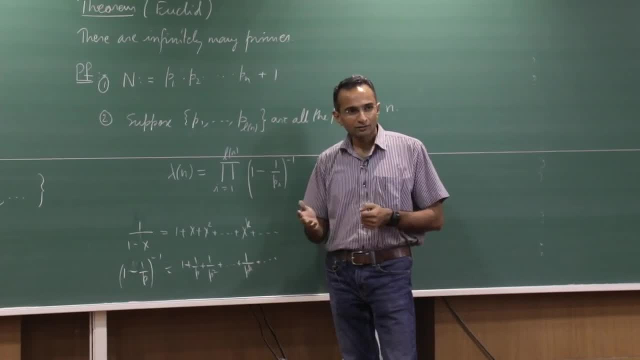 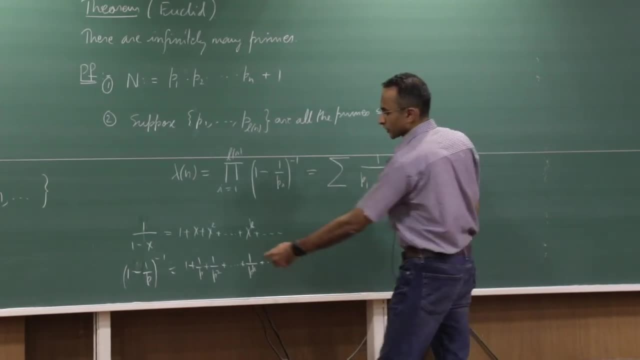 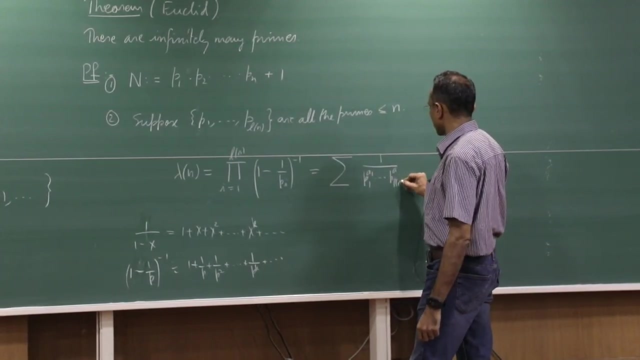 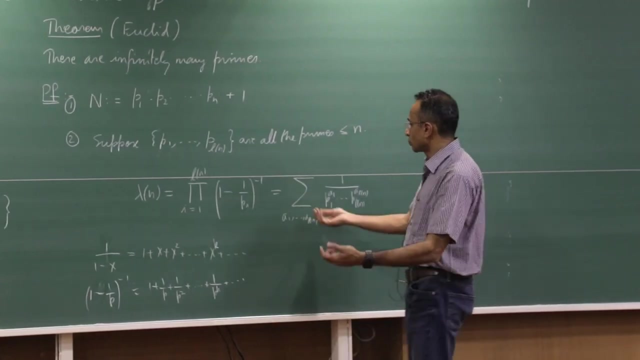 if I multiply all that particular p power, if I multiply this together, then this would be: it's going to look like a sum of terms: p 1 to the sum. maybe it picks up the a 1 term there. So p 1 to the a 1 to p k to the a k, whatever l n with the a l n where. 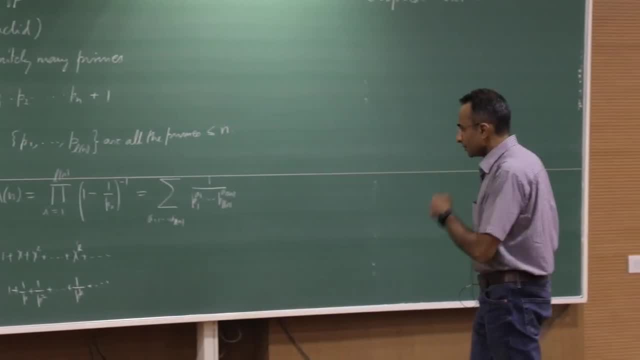 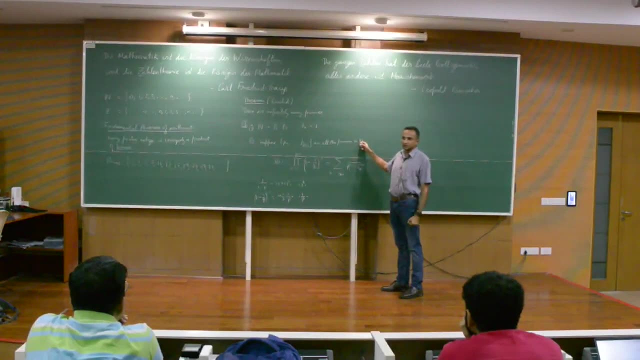 the summation is over all triples, l, n, triples of nonnegative integers, ai's. Now, if I ask, appeal to the fundamental theorem of arithmetic. This is what is this capturing? So every this n is itself a prime, or the fact. 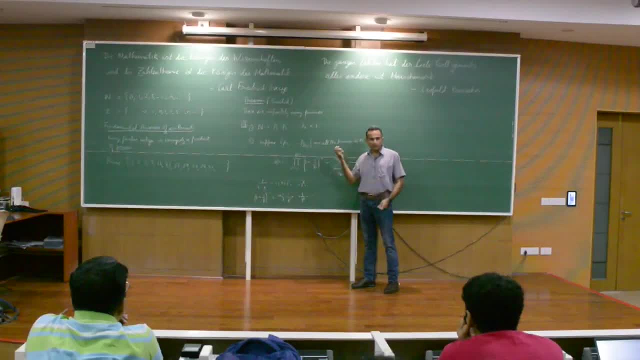 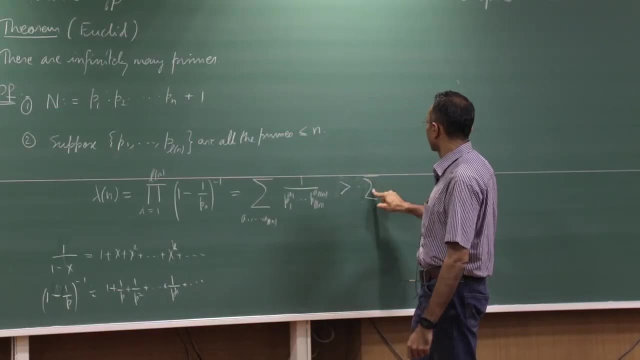 is a product of primes and the possible products. the primes will have to be smaller than n, So it's amongst this set. So this is really well, it's at least one over, is at least summation one over. give me some other letter. m m going from one to n. 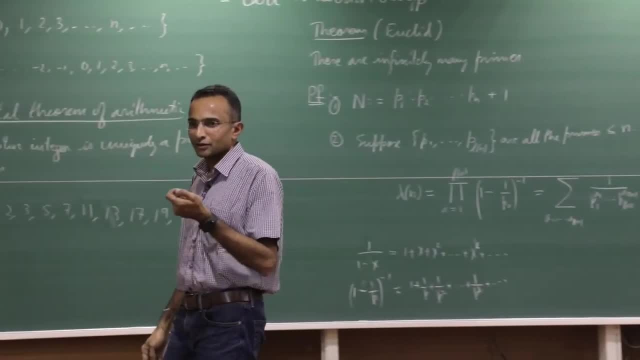 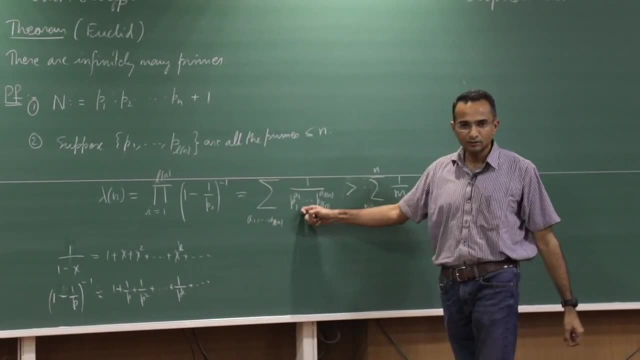 All the. any take any integer less than n m. I look at one over m, look at its prime factors. it's amongst these. so that should appear here And this might have more terms. So this term is at least this much. 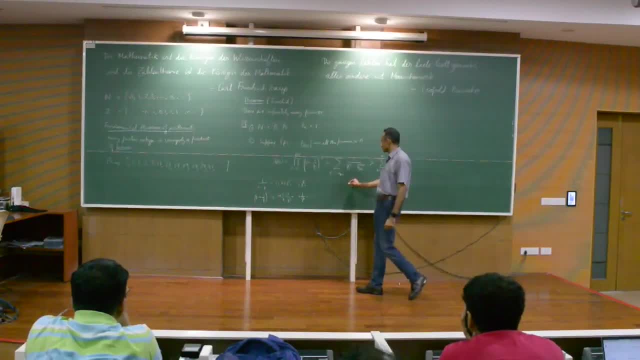 And what do I know about this guy? This you have seen in calculus courses. You know that. so now, if I take limit as n goes to infinity, I know this diverges. I know that this diverges. Yeah, so you've seen this as the harmonic series. 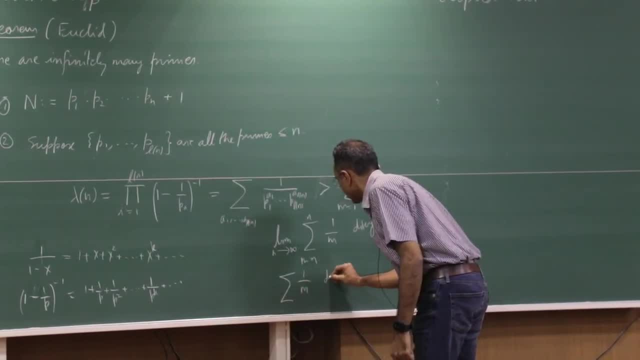 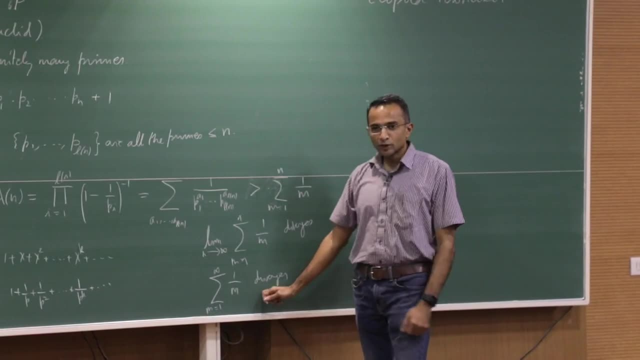 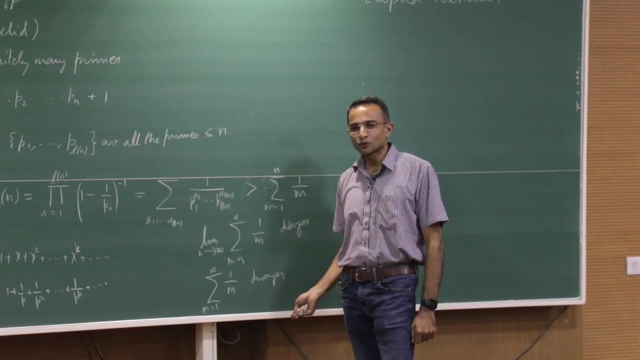 maybe summation one over m diverges, m going from one to infinity. This, by the way, is a 14th century theorem. I don't know how many of you know this. There's a nice math trivia. Anyone knows who proved this? 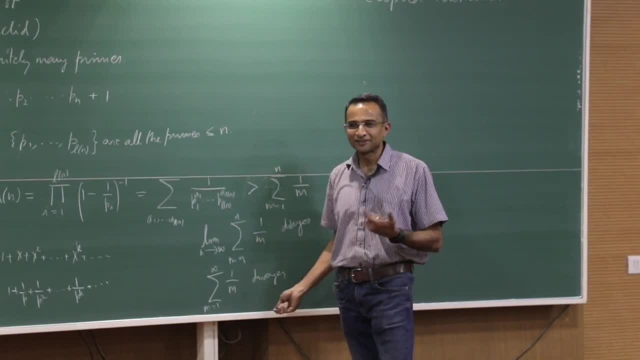 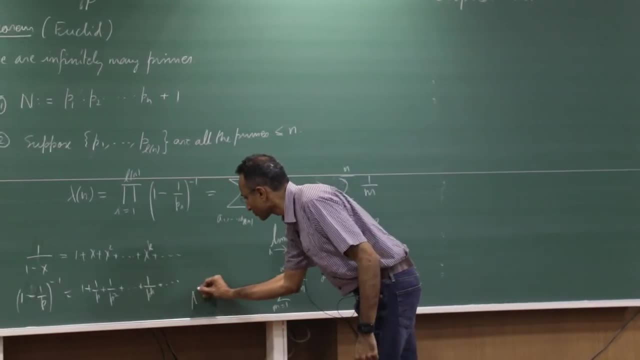 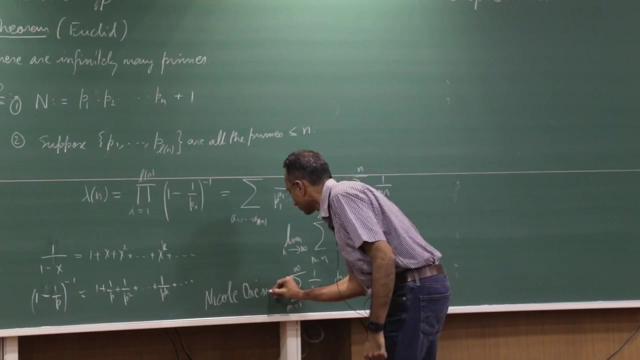 The 14th century theorem: Math club people, you should have a math trivia quiz. This was proved by a French philosopher, Nicole Oren. I am not sure about the accent, In any case this diverges. So now this gives me a proof that. 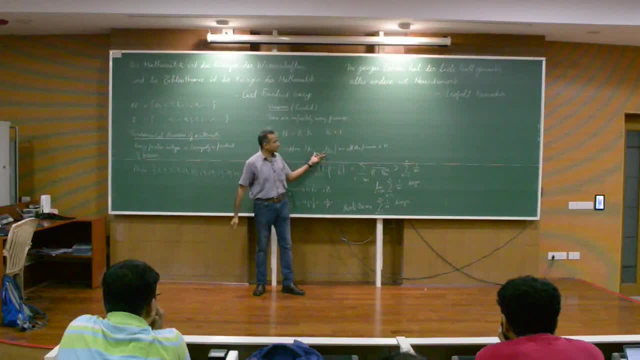 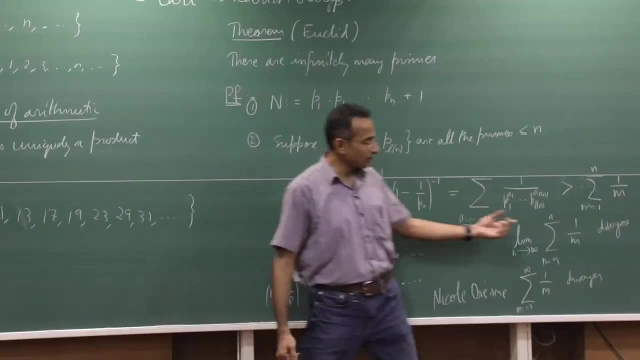 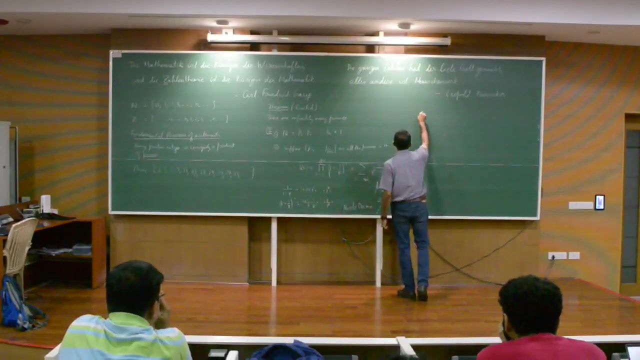 they have infinitely many primes, because suppose not, if they're only finitely many, and maybe they were all less than something, then this term here cannot be shooting off to infinity. If the finite product is finite, it converges. Third proof, which pushes this a little further: 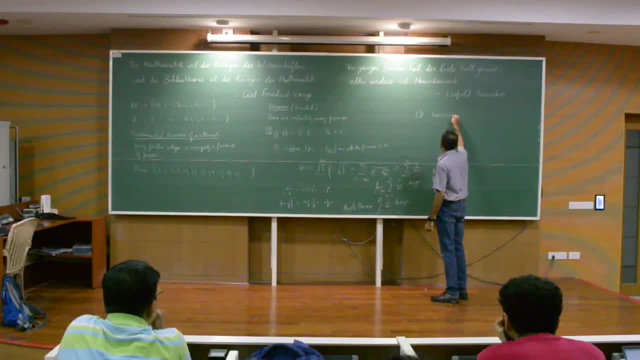 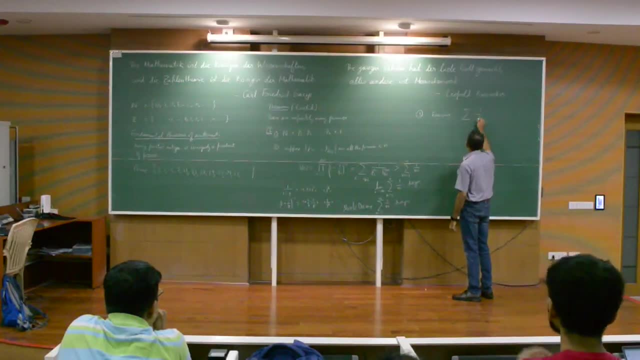 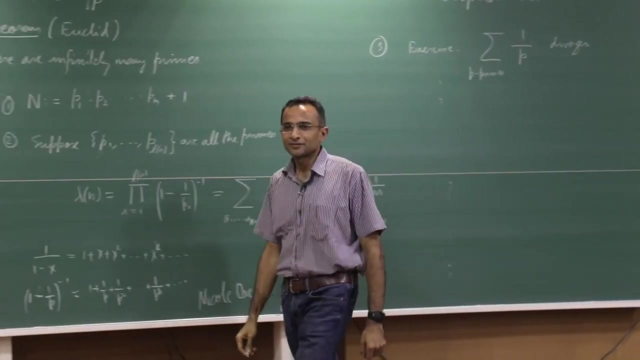 which I won't do, but I'll leave this as an exercise. It's somewhat like this: The divergence of this harmonic series proves that summation one over p, as p runs through all primes diverges. Anyone knows the proof of this. 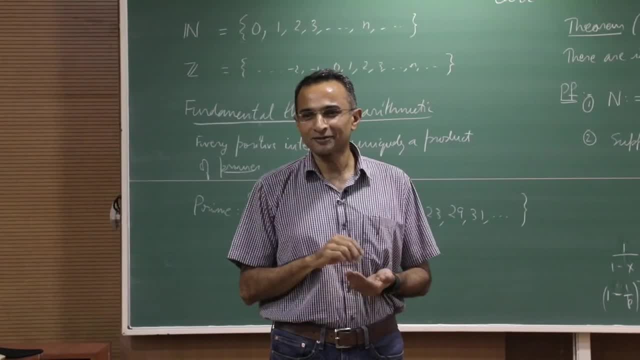 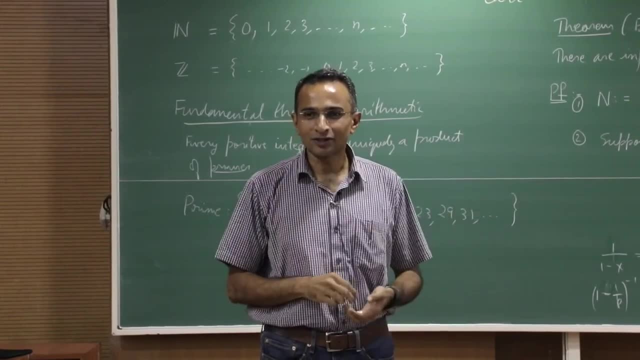 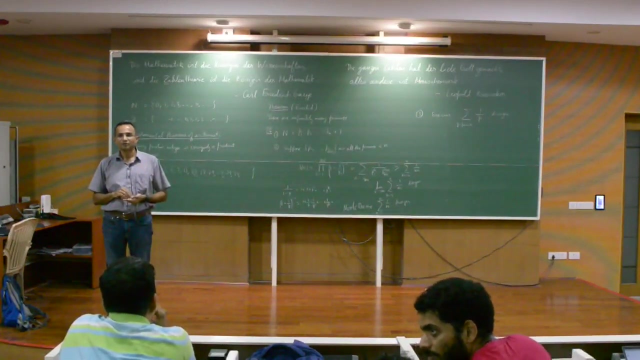 Now it's. the floor is open to the PhD student. Very good, Give me a proof, Go ahead. Do you know a proof of this? Yeah, Okay, Tell me. We have to write this as something like 1 by 1 plus 1 by 2 plus 1 by 3.. 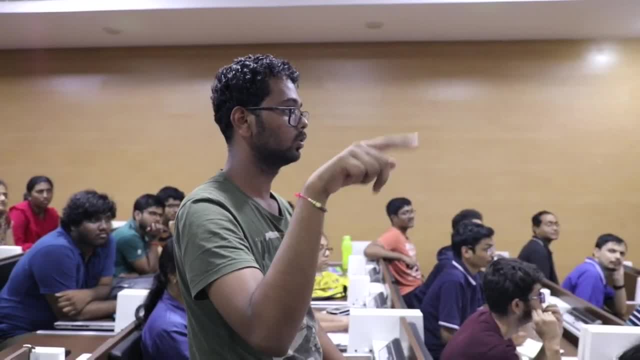 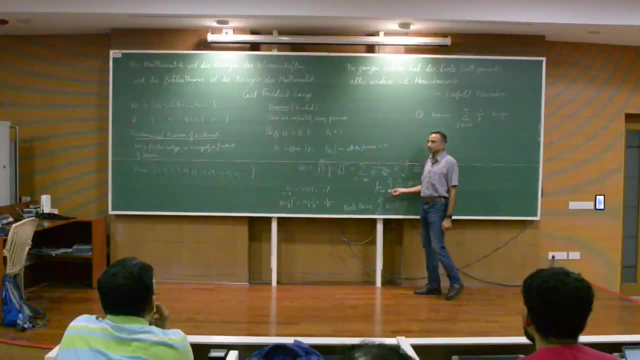 Of course It's greater than or equal to 1 plus 1 by 2, plus 1 by 2, plus 1 by 4 plus 1 by 4.. You're talking of the divergence of this series, Yeah, So here I'm running over only primes. 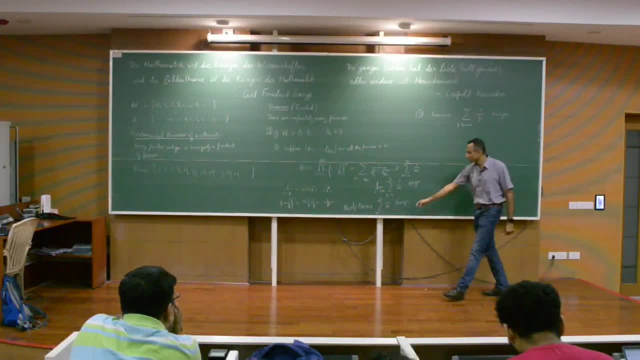 That argument is not going to work. Your proof is actually what you just gave. that's fine. That is, in fact, Orem's proof. That is the 14th century. This was the original proof of divergence of this, This one. you won't be able to club together the first two terms. 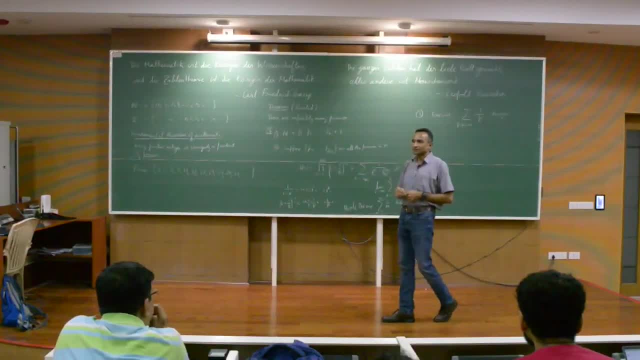 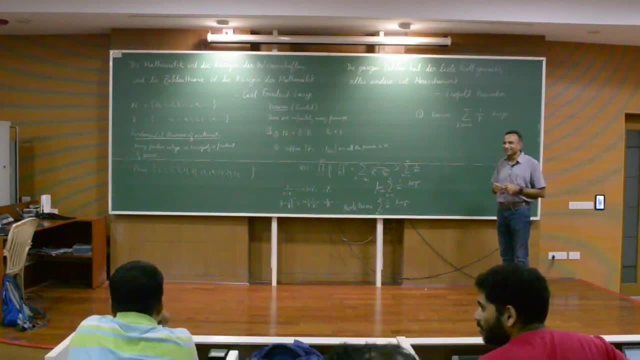 the next four terms, the next eight terms and so on. It's a little subtler. Has anyone seen a proof of this? Uh-huh? So actually I will be honest with you. I also knew a proof and I forgot. 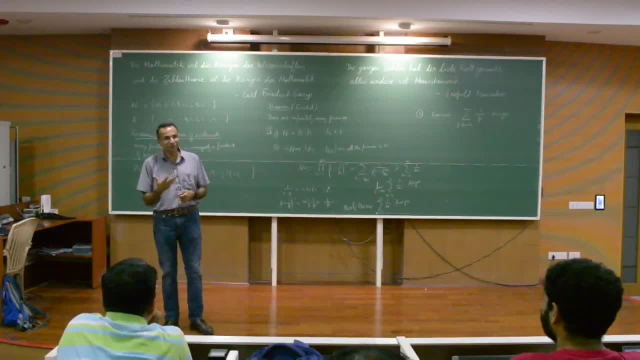 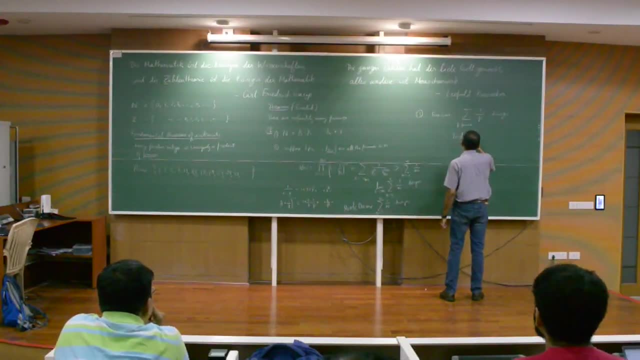 And while I was preparing this talk, I was like, okay, this is a cool statement. I know it's a non-trivial exercise and I reminded myself how it goes. You can look this up in Ireland and Rosen It's. the book is called A Classical. 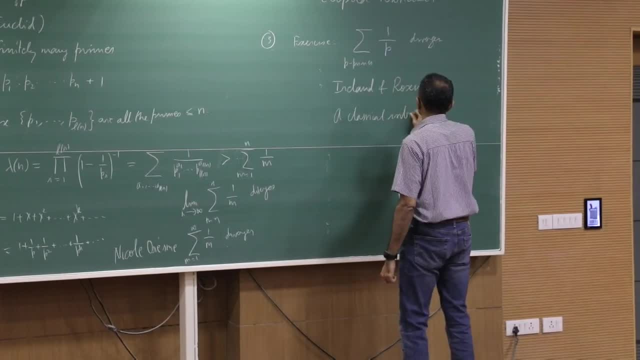 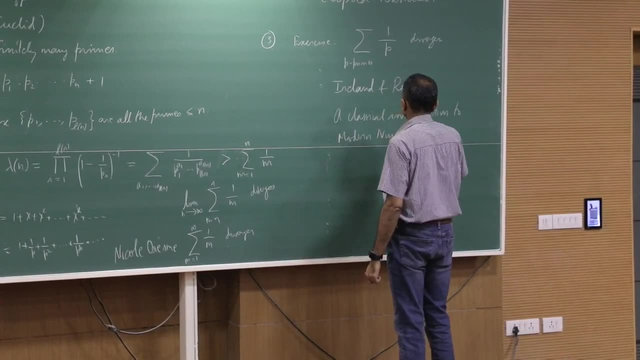 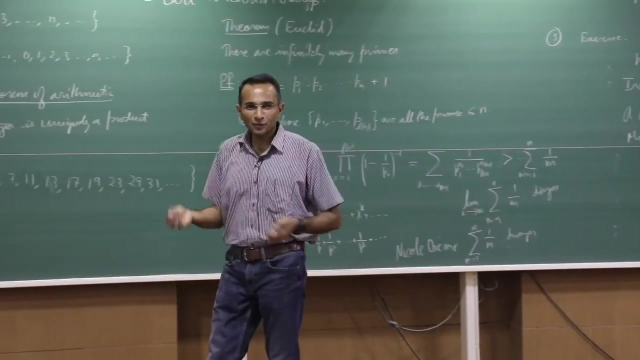 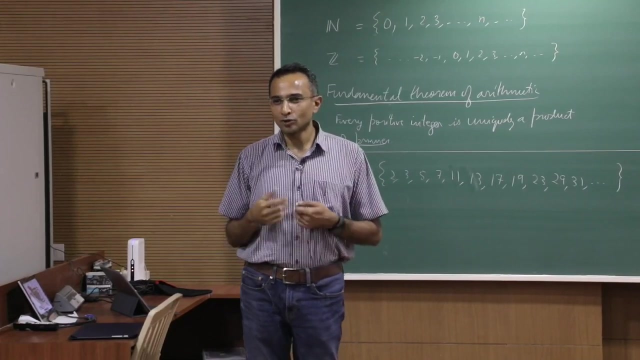 Introduction to Modern Number Theory. Many times I get e-mails by someone or the other in typically first year, second year, third year zone, who will email or come to my office asking what to read and my standard answer is: go read. 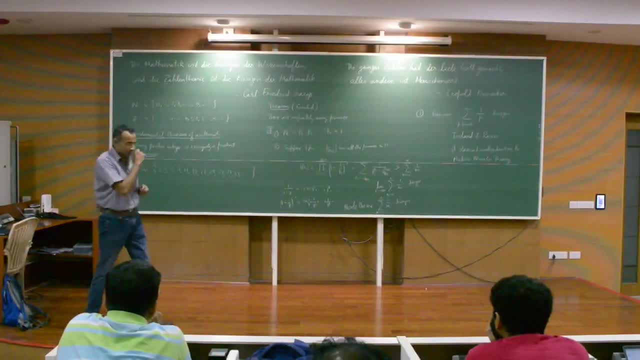 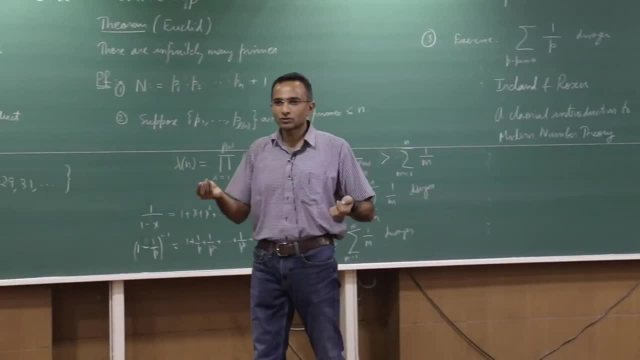 I learned in Rosen's book. If you wanted to read number three to get started Somewhere. in our ICER curriculum we don't chew on basic number theory. There's only a course on algebraic number theory, which might change in the near future. 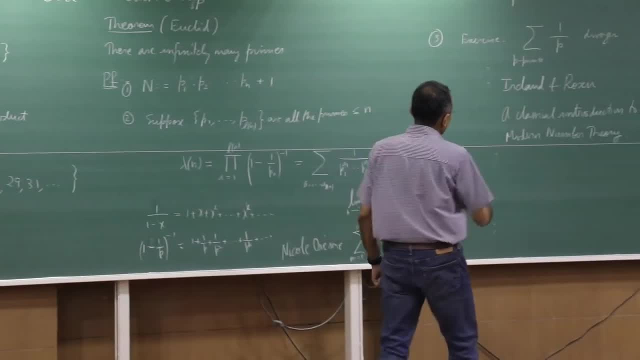 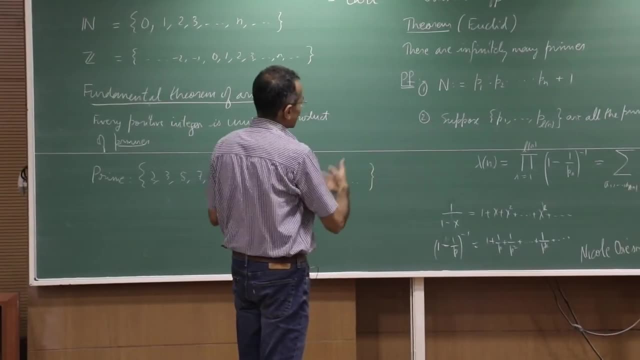 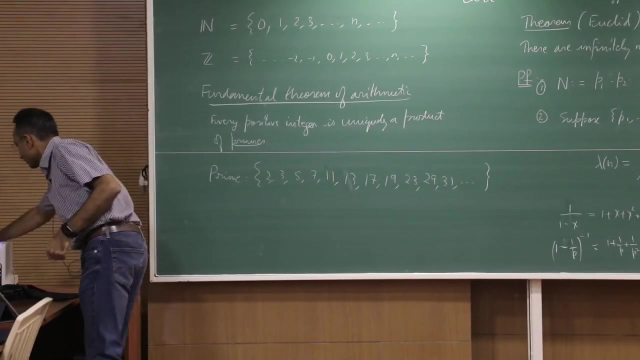 but you guys may not see it. Anyway, this is a wonderful book, All right. So we have infinitely many primes and I was almost going to say there are infinitely many proofs. here is two. Now I want to play around with this idea of 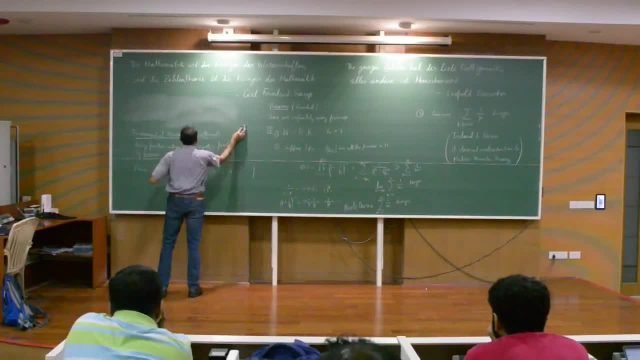 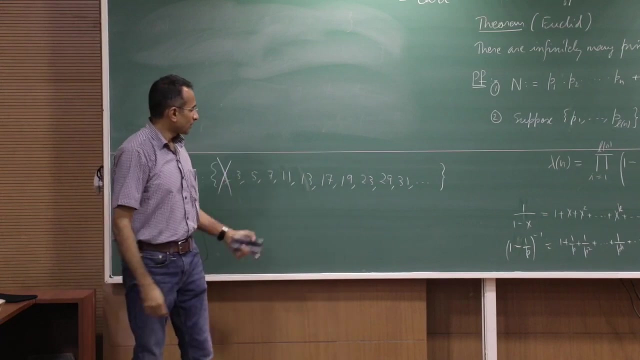 infinitude of primes, slightly focusing my attention. Well, I got this list of primes. Of course, this guy is an aberration, So you've just forget that All the others are odd numbers. If I take any odd number, two and plus one. 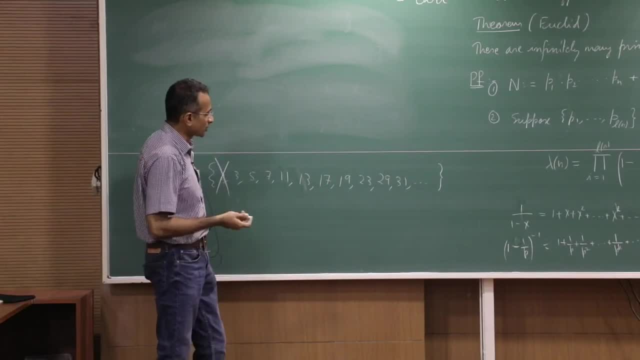 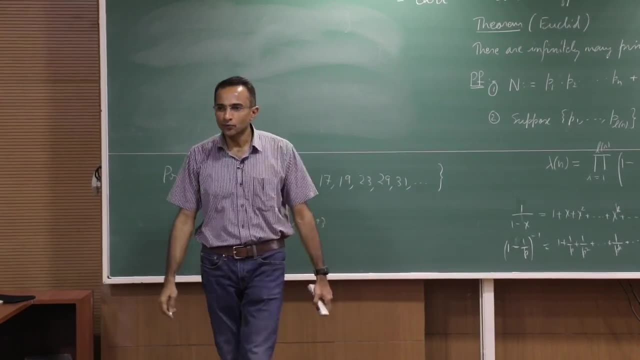 depending upon whether that n itself is even or odd. you know that any odd number is of the form either four k plus one or four k plus three. If I take an odd number and divide by four, if I take any number and divide by four, 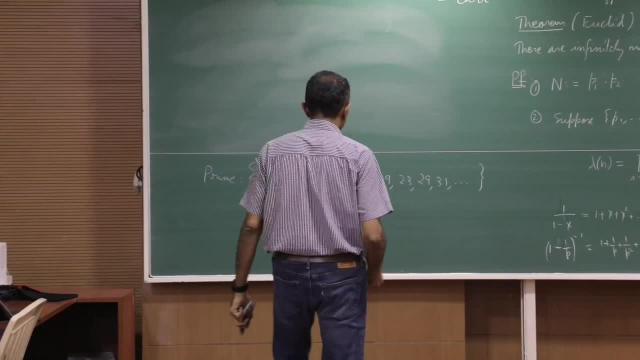 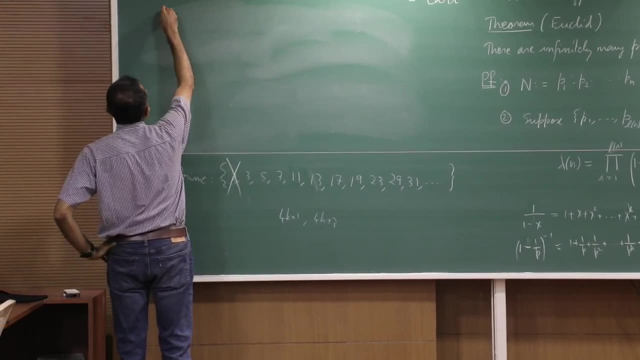 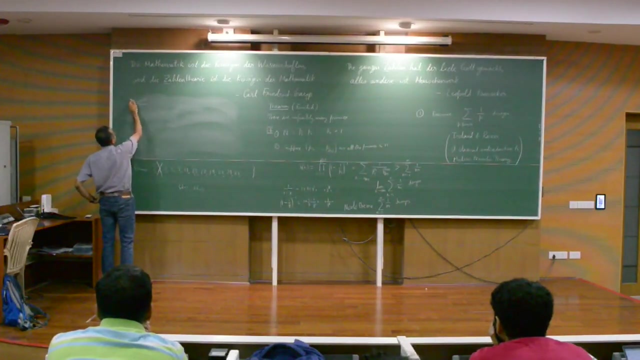 the possible remainders are zero. one, two, three. Zero or two will force the guy to be even, and one and three is odd. Now let me tweak Euclid a little. I'll maybe just call this a proposition. Maybe let's elevate it to a theorem. theorem. 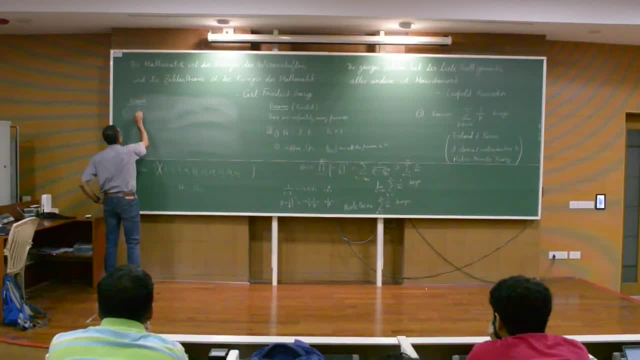 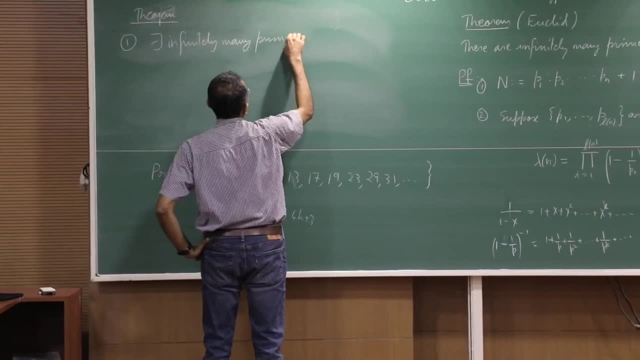 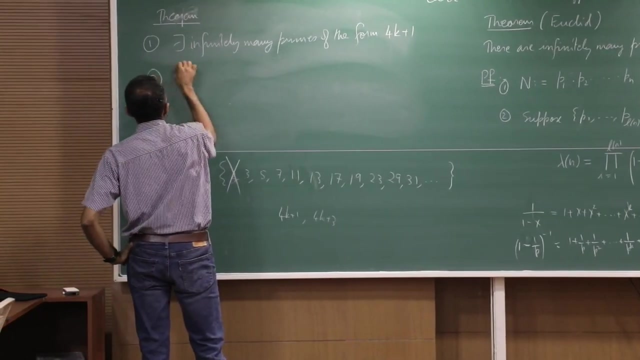 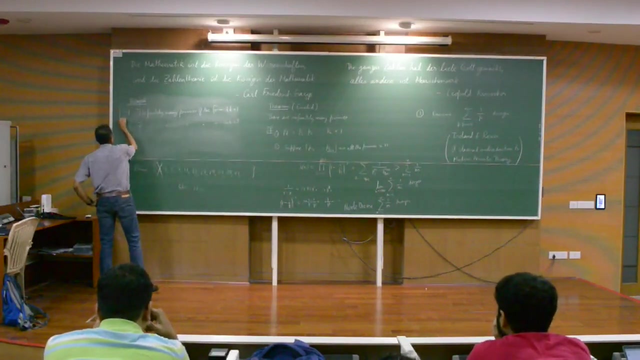 So first statement: there exists infinitely many primes of the form four k plus one. And secondly, there exists infinitely many primes of the form four k plus three. These are typical examples of this. Okay, Typical exercises in a basic, in a first course, in elementary number theory. 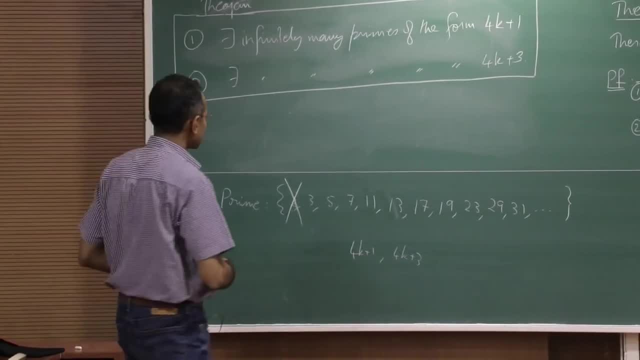 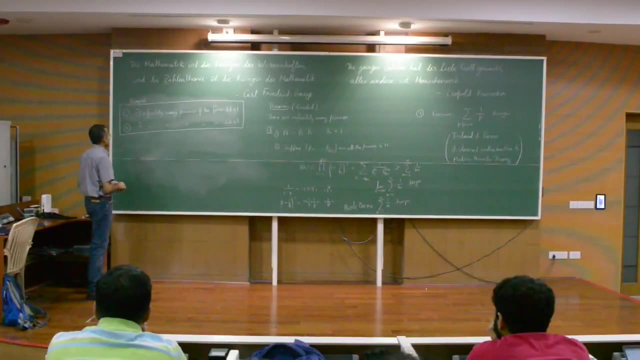 So I'm going to do this. I'm going to do this exercise for you. Let me start with the easier one. I want to prove the infinitely many primes of the form four, k plus three. The proof are all modeled on Euclid. 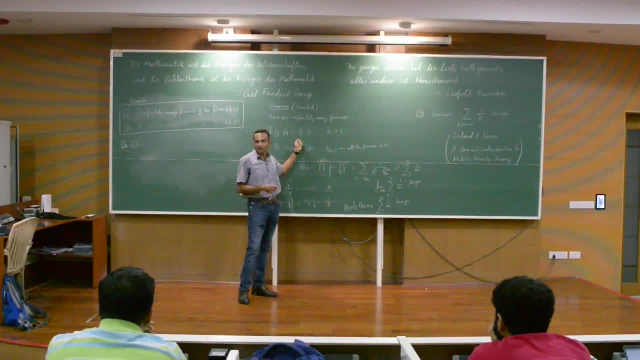 Suppose not, You cook up some integer which will have a prime divisor, and then, if you have cooked this up cleverly- here the cleverness was taking the product and adding one- You do something like this and you follow your nose and out will pop another prime. 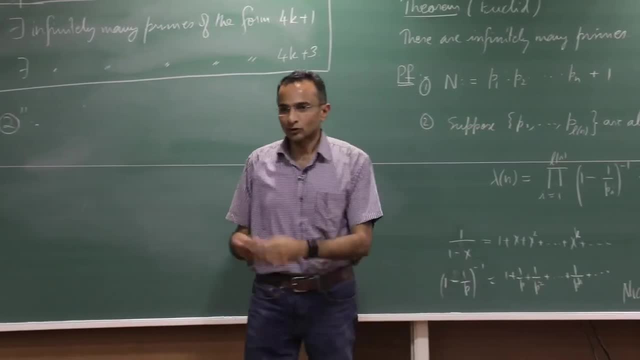 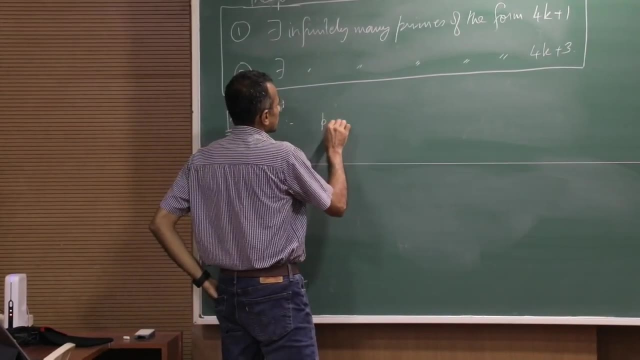 which is necessarily of a certain type, which can't be in the set. Okay, So that's the nature of the proof in either of these two cases. So let me do this here. So suppose P1 through Pn. 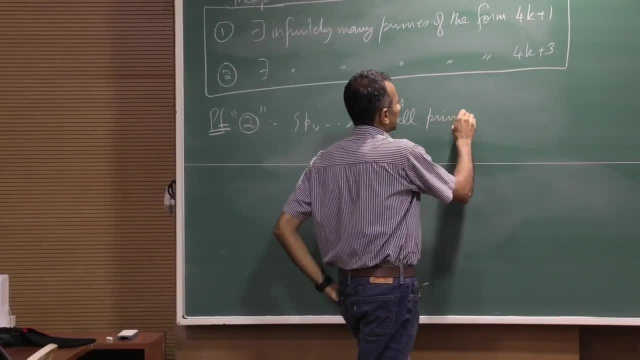 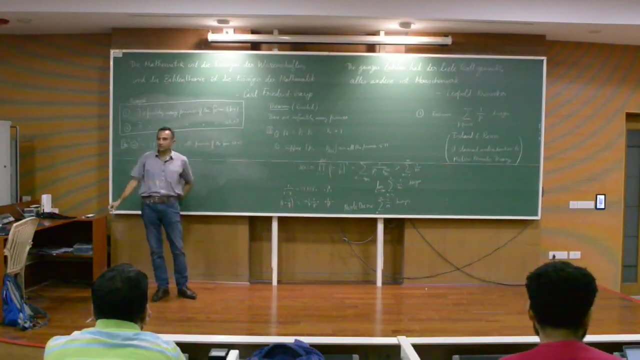 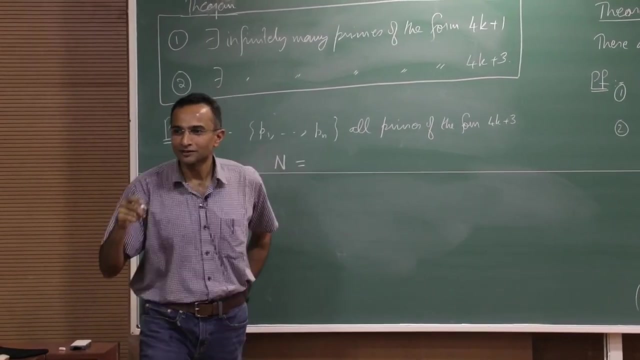 this is all primes Of the form four k plus three. I'll do that. the easy one first, And then anyone who's had some basic number theory. can you tell me what will I write down? Sorry, did I hear a Jordan holder? 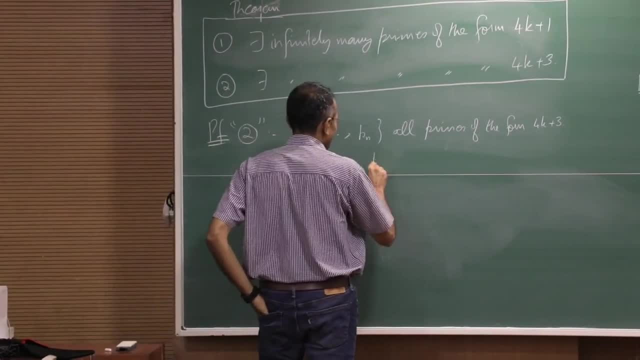 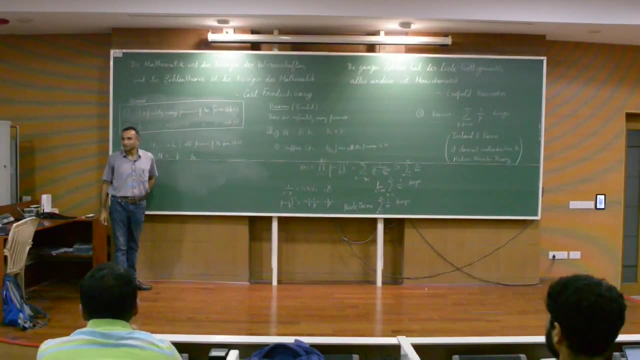 Product. Yeah, Okay, I take the product And then Let me look at this. Okay, So it's some artifice of this kind. So suppose this is the set of all primes of the form four k plus three. 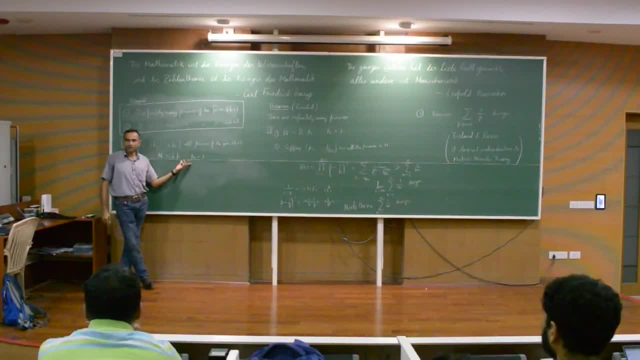 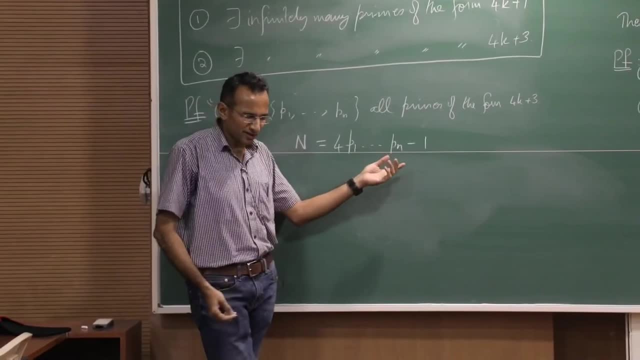 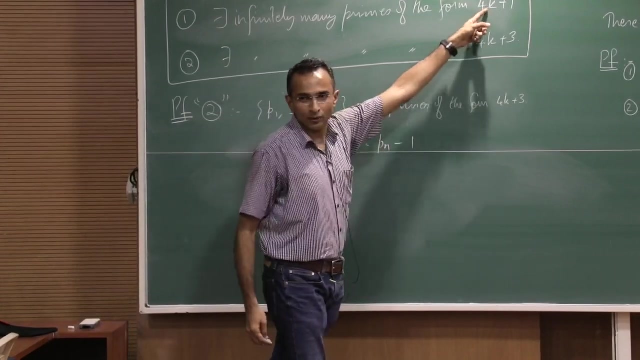 consider this integer, This is going to have a prime divisor. This guy, upon dividing by four, also has a divisor. reminder three: If all the primes dividing this were are not of this type, then they're all of four: k plus one. 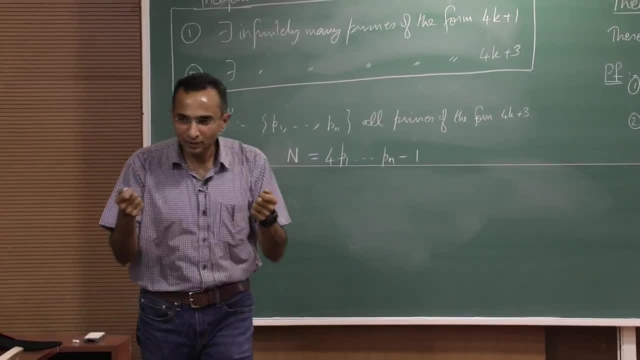 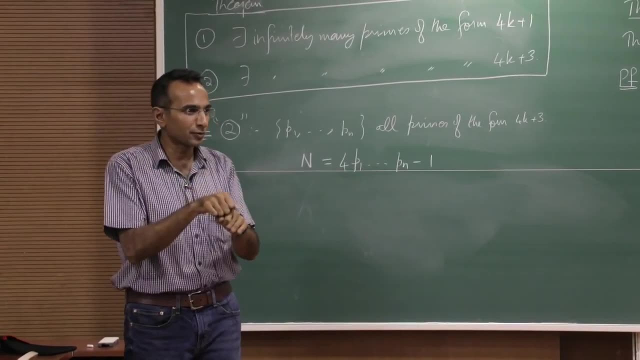 but two numbers of the form four k plus one will. the product of two such numbers is again of the form four k plus one. If two numbers leave a reminder of one, upon dividing by four the product will also leave the remainder, leave the same reminder one. 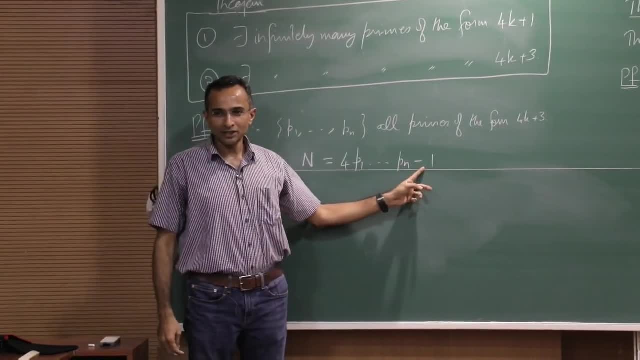 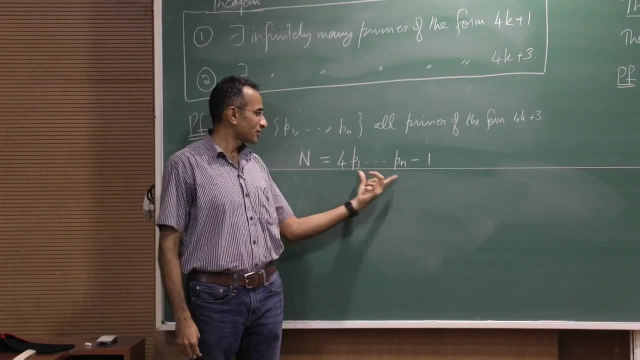 So this guy, not leaving the reminder one necessarily has a prime of the form four k plus three, So it's to be one of these. Therefore, that prime divides this, it divides this, it divides minus one. that's not possible. 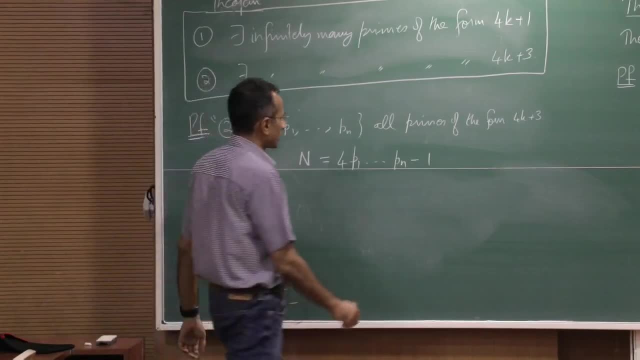 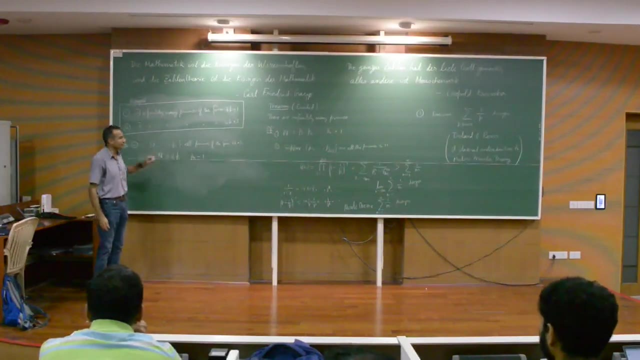 So this is the key, Key point: you can fill out the proofs Already. by a few blank looks I can tell that some of you didn't quite work with me, but that's okay, It's stare at this and figure it out. 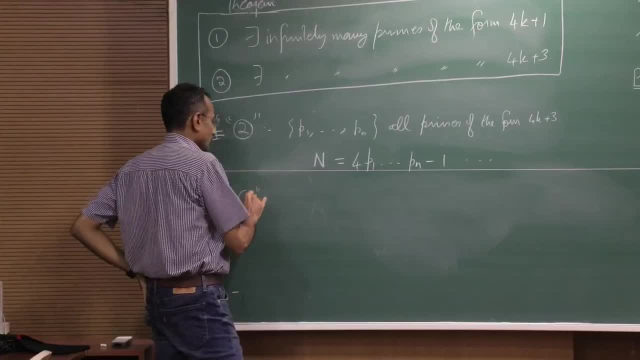 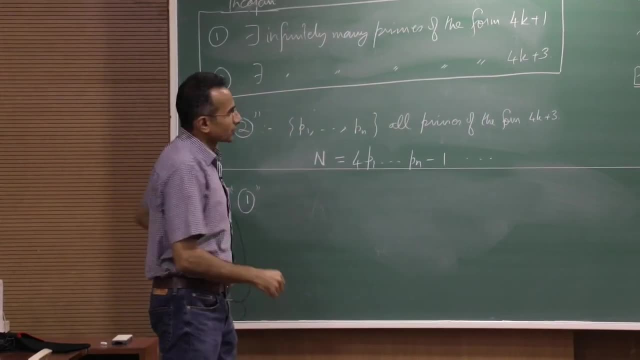 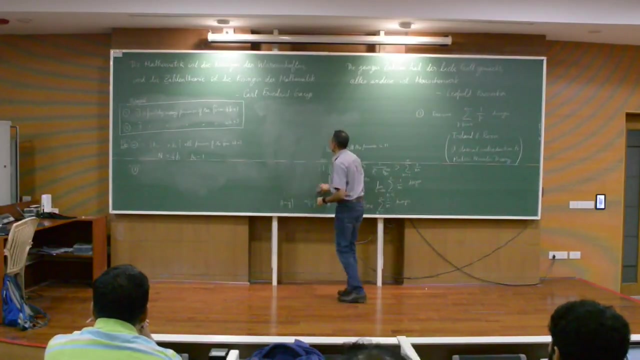 It's not hard, Let me do a slightly harder one. four k plus one. So I want to prove the infinitely many primes of the form four k plus one. For this I want a sub-theorem, Just so that you go back from having. 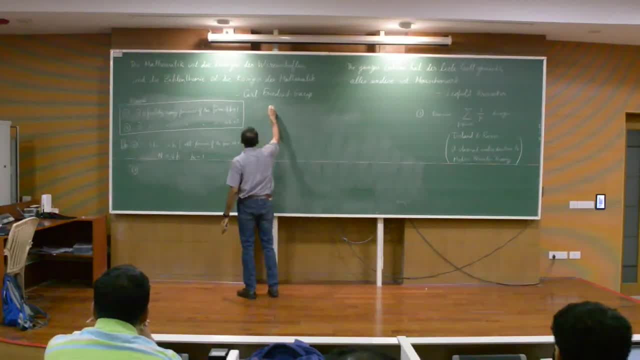 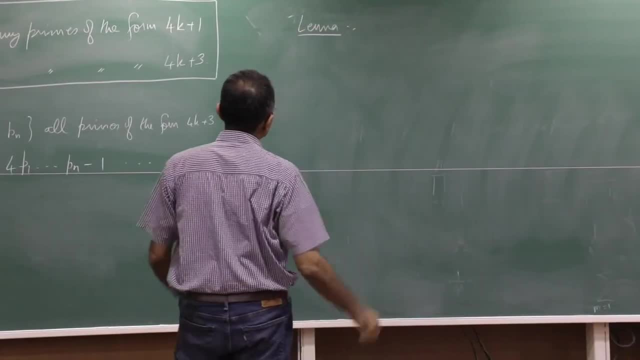 actually learned some number theory here. Here is a. since I'm using this in the aid of a proof of a theorem, let's call this a lemma, but this is a theorem in its own right. If so, p is a prime. 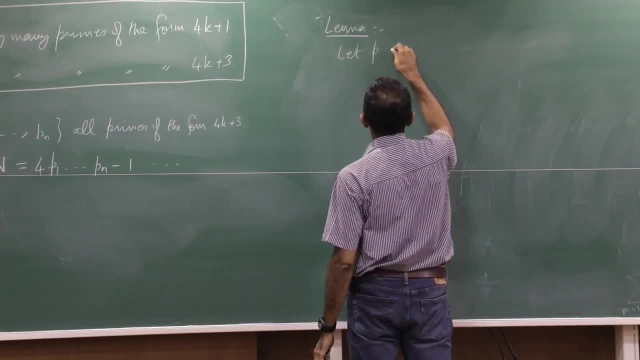 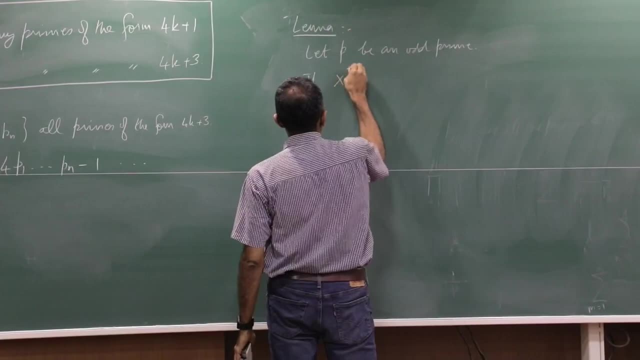 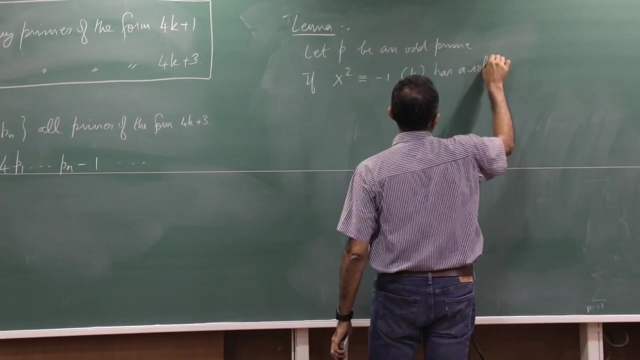 P is always a prime in number theory. Let p be an odd prime. If, if, if, if, if the equation x squared congruent to minus one mod p as a solution. So this is, by the way, this notation is due to Gauss. 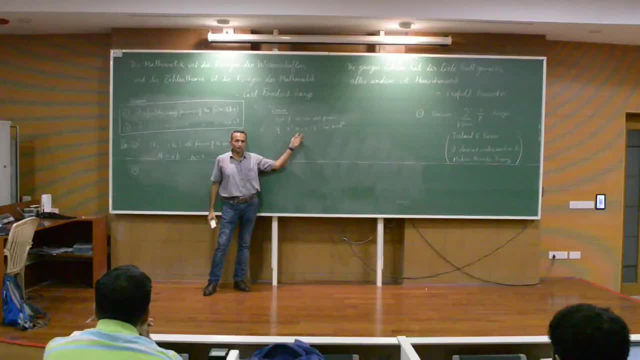 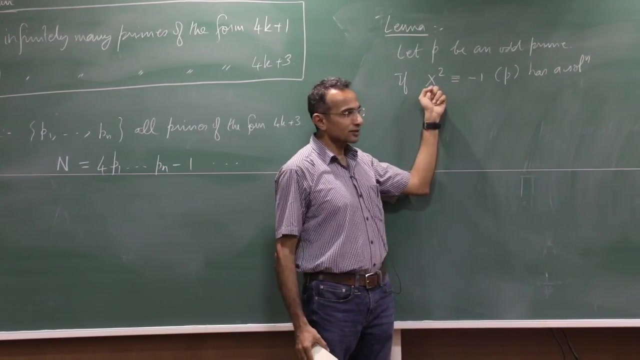 He should go and look up somewhere his meditation over notions versus notations and somehow having a good notation aids a lot in mathematical thought. That's all that rhymes well, It aids a lot Anyway. so this means I'm trying to find integers. 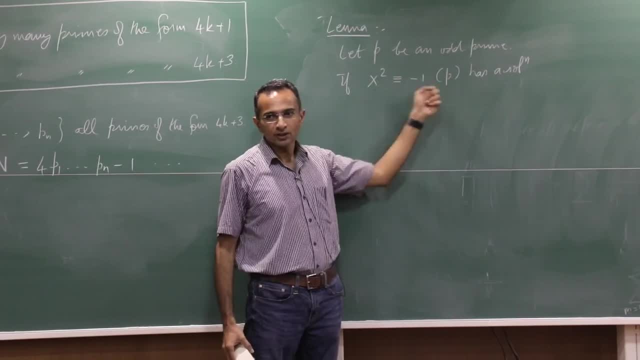 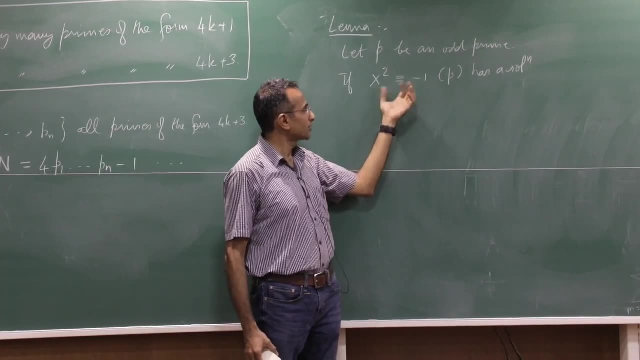 whose square is minus one modulo p. In other words, after dividing by p, it leaves the remainder of minus one. This, this notation A, is congruent to B mod. something means the difference is divided, is divisible by that modulus. So I'm trying to find square root. 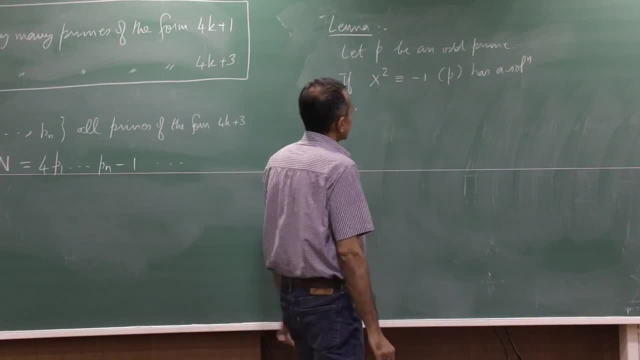 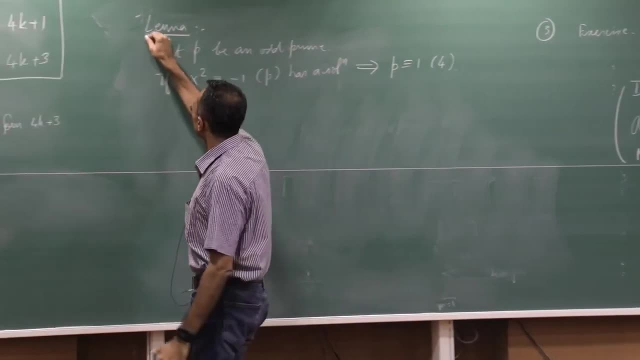 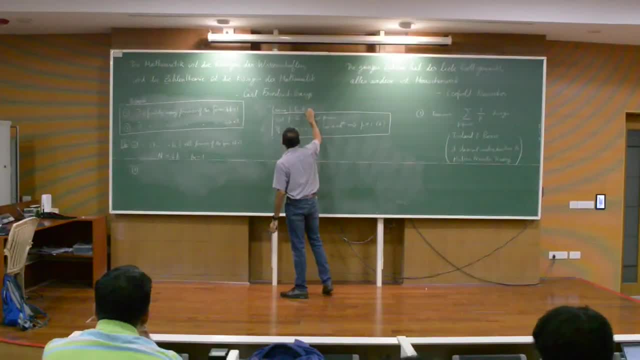 a, not a. this is, this is. this is, By the way, so when you come out of school, many people in school pronounce this as Euler. it's Euler. Euler came out of the German-speaking part of Switzerland and EU, in German is OI. 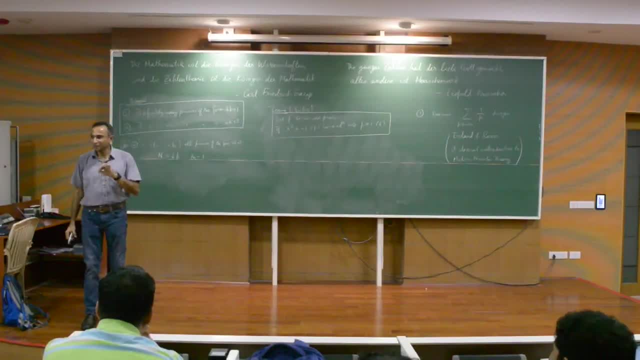 But Euclid is Euclid and not Euclid. Euclid didn't come out of any German-speaking part of any. Where did Euclid come out of So anyway, so proof of this. So suppose there is some integer which, suppose I have some integer which. 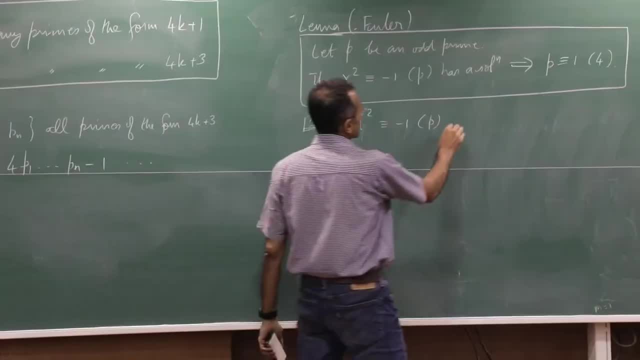 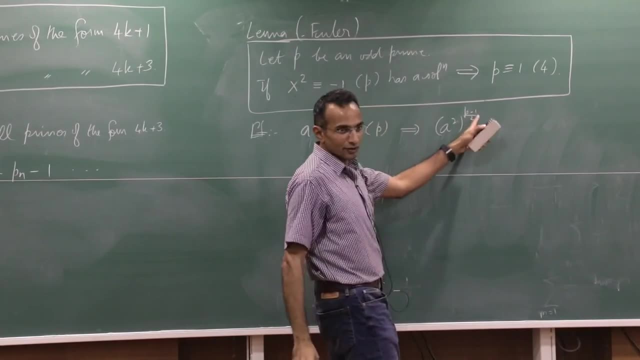 pretends to be like the square root of minus one. What you do is you raise both sides. P is an odd prime, So I raise both sides to the p minus one by two-th power, which is an integer, p being odd. 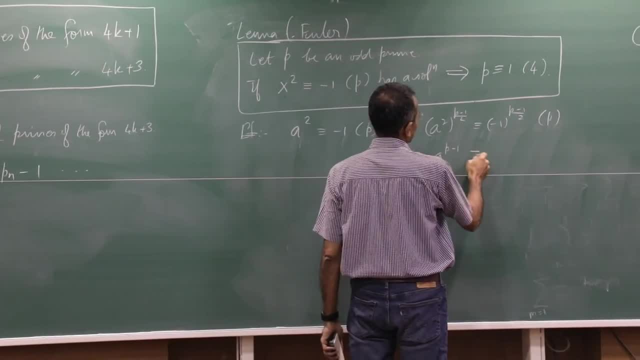 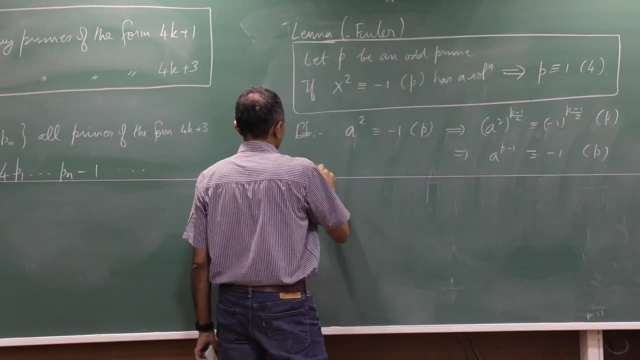 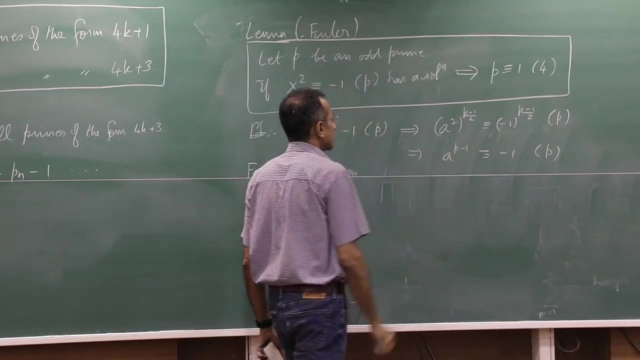 And this side is a to the p minus one and that's congruent to minus one. And there is what's called Fermat's Little Theorem, which says that if I have an integer a not divisible by p, then it's p minus one's power itself is congruent to one. 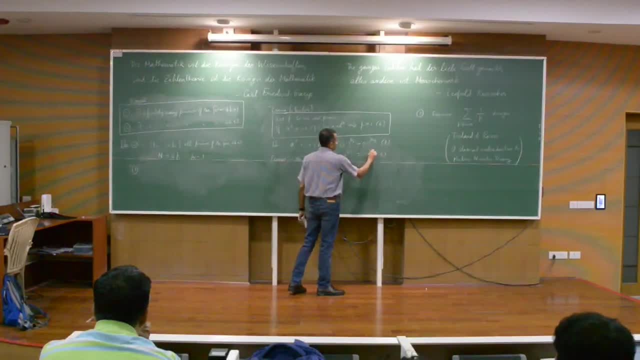 This is congruent to one, So I get minus one to the p. minus one by two is in fact one. That congruence actually becomes an equality. Think about that step a little. And this will imply that, well, p has to be of the form one modulo four. 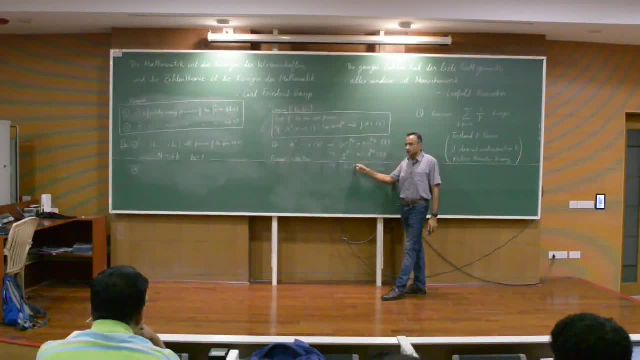 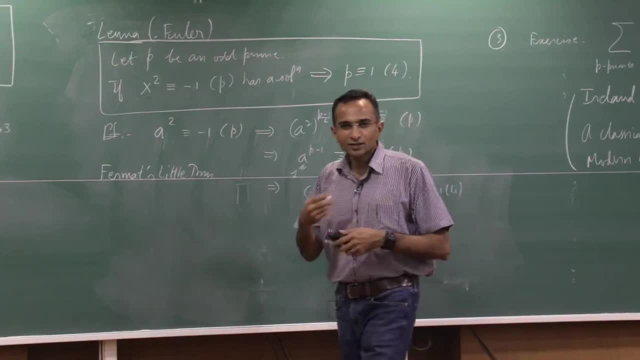 If p is like the number three, then three minus one. by two this becomes odd. so minus one that becomes minus one. left-hand side of p is three mod four. So there are this kind of any number of this type of congruence properties. 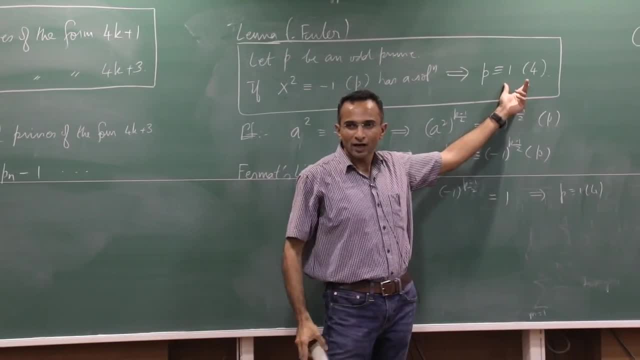 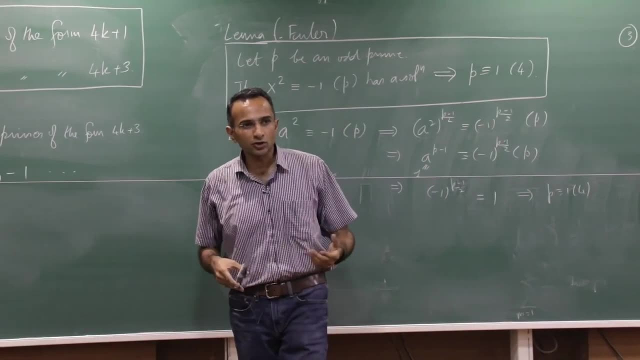 capturing something about the shape of the prime, And Gauss's greatest achievement is one of his greatest achievements, at least. number three's greatest achievement is what's called quadratic reciprocity. He was so fond of that theorem that he gave several proofs in his lifetime. 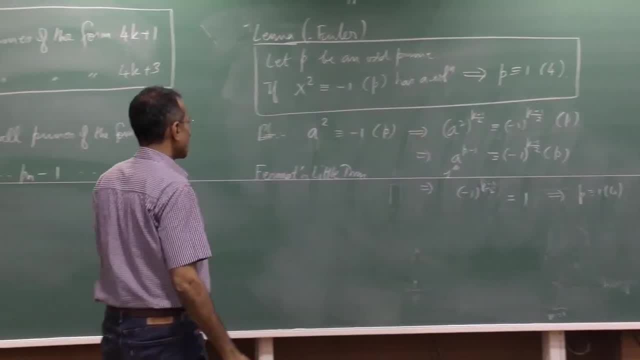 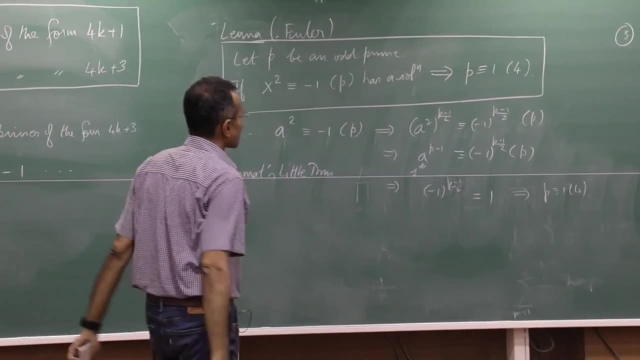 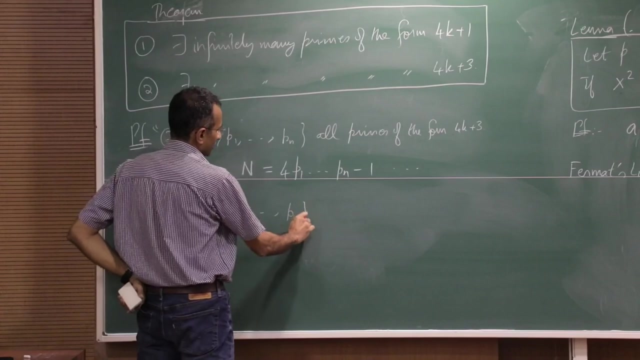 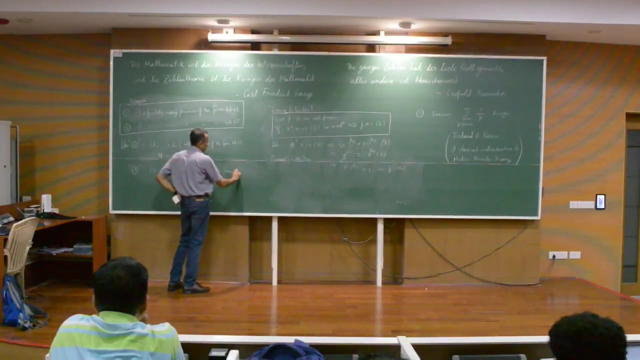 captures statements like this. So this gives you a handle on some prime to the form four k plus one. And now we go back here. suppose now these are all the primes of the form four k plus one. Your ingenuity is cooking up an integer n. 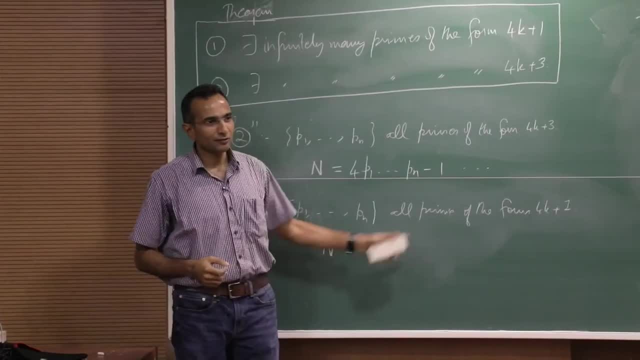 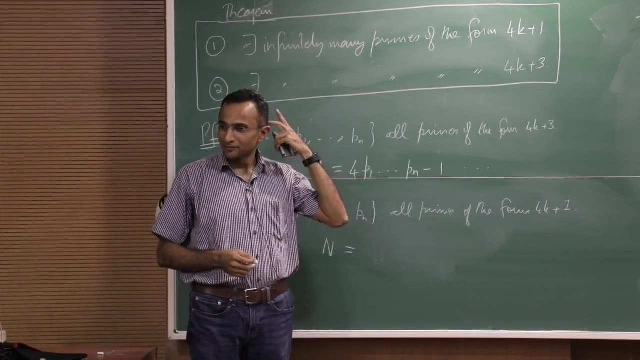 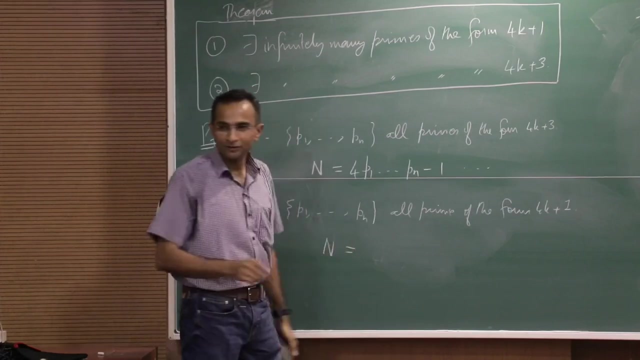 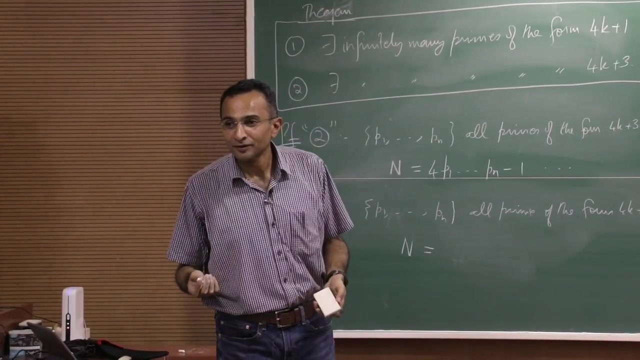 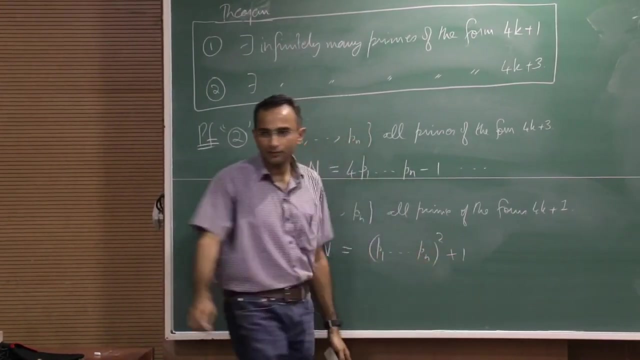 which somehow includes all these primes. Give me the integer. I've done some exercise for you in some sense. Say it again: It's okay. at worst you are wrong, That's right. I take the product of all these guys, square it up and add one. 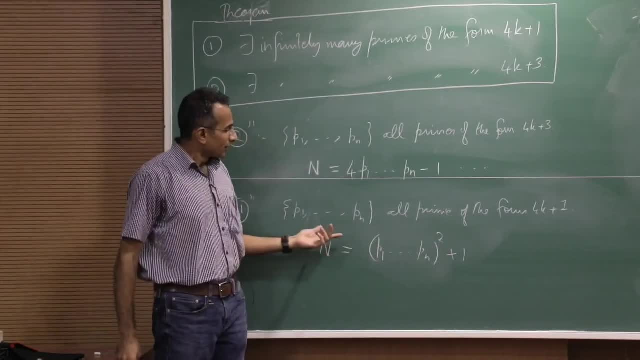 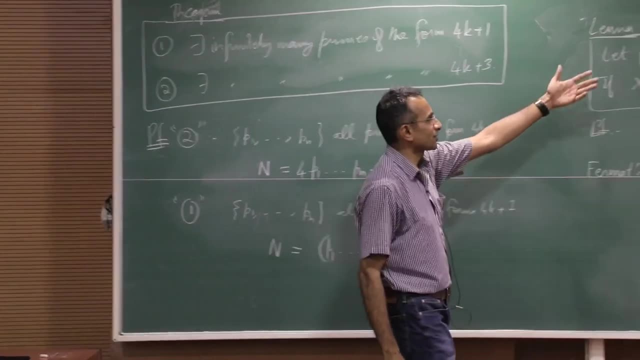 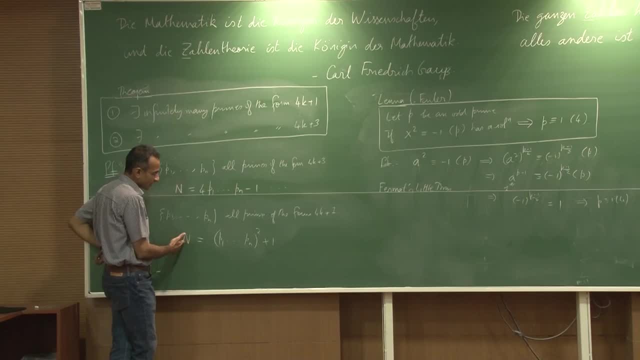 because of well, there is some theory which says that I can identify primes of form four k plus one because of well, there is some theory which says that I can identify primes of form four k plus one through some such gimmick. So if a p divides this n. 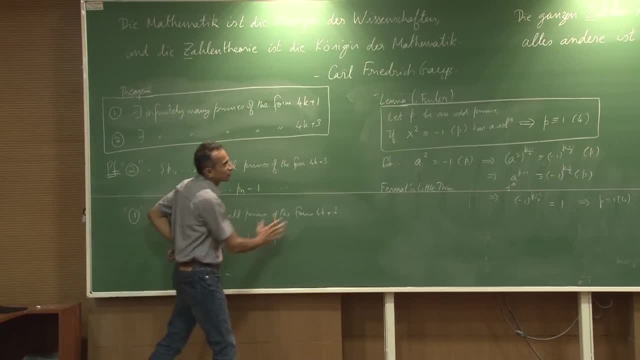 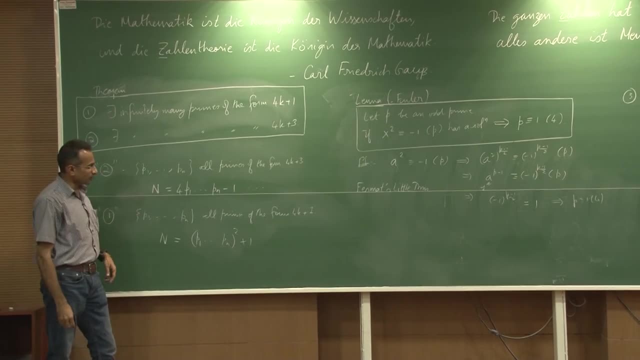 well then, this guy, this product of numbers, p, one through p, n, is a solution of this equation. If p divides this, that's to say, well, this little a is this: So this p is of the form four k plus one. 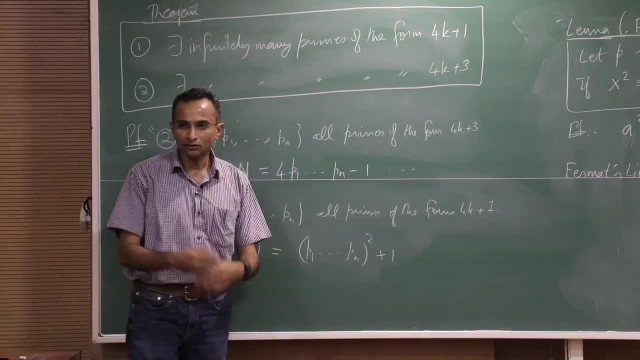 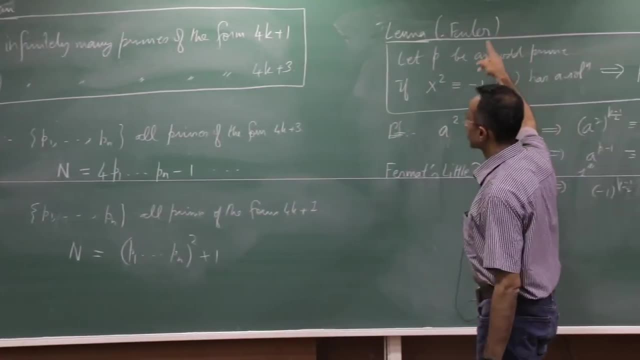 it has to be one of these. it divides this, it divides this, so it divides one contradiction. The rest of the proof is really the. formally it looks the same. So the only well, Euclid has gone there. the only thing was to cook up the right sort of integer. 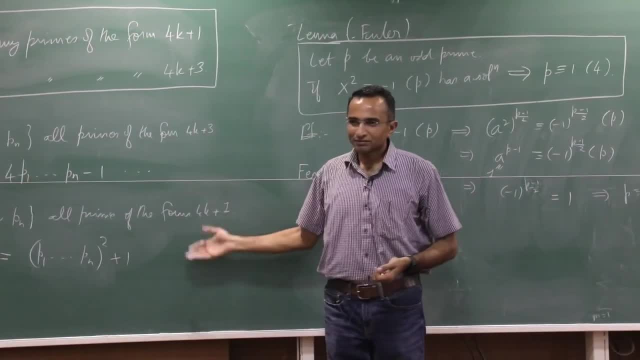 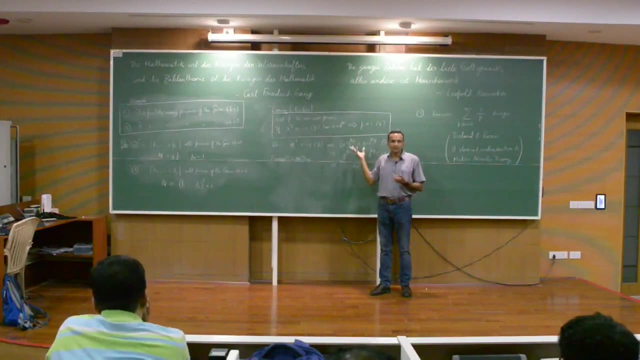 As you can imagine, already for four k plus one. this was not totally trivial. okay, I mean I needed some. it's important, it's serious number theory, but it's, you know, this is all well known and 200 year old mathematics. 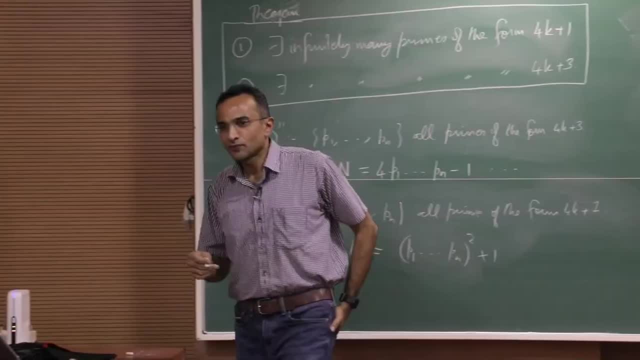 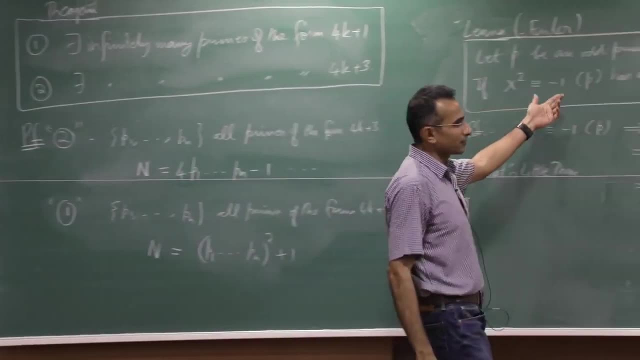 Suppose you ask yourself the question: are there infinitely many primes of the form 17 k plus five? Then you're going to be really hard pressed in coming up with some kind of criteria like this which captures that sort of shape of that prime. 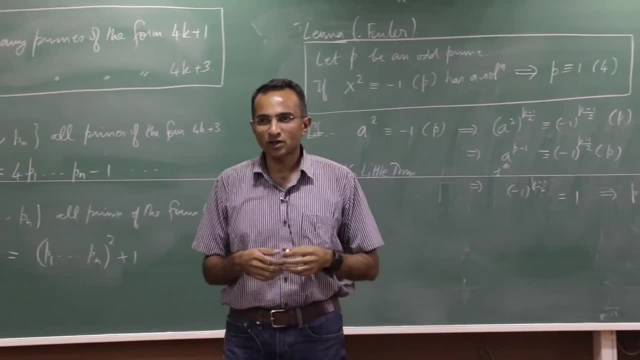 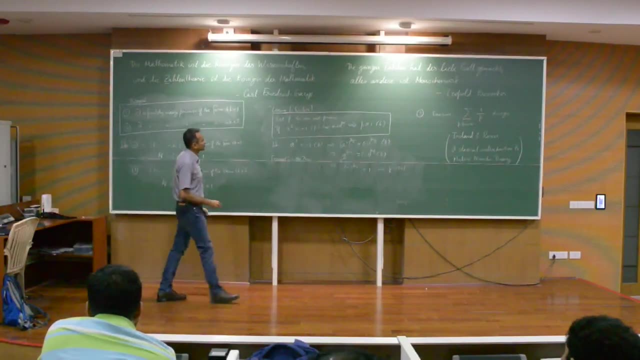 So there is some one wants to think about this in some systematic, some structural way And now enters. so you see I've mentioned so far. what are all the names I've mentioned? There are already. Gauls Kronecker hasn't showed up in this, but Euclid. 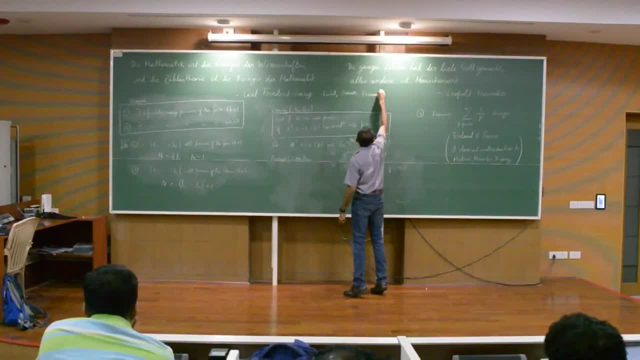 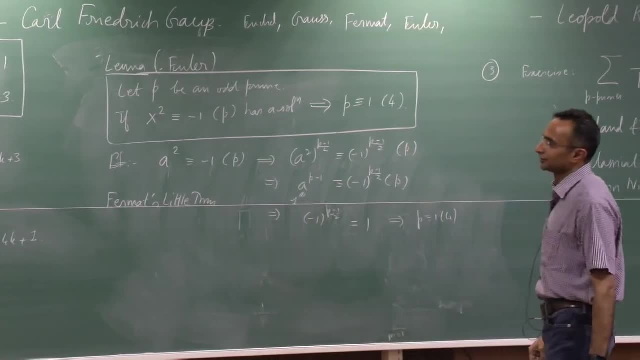 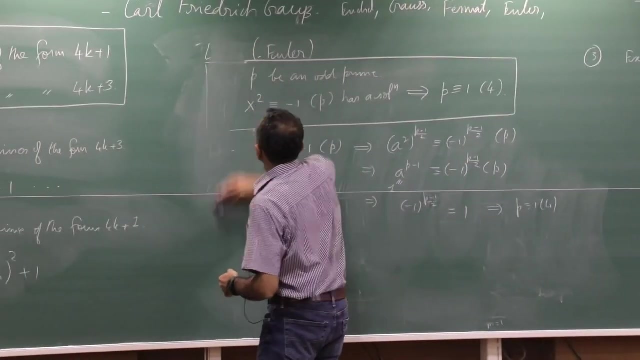 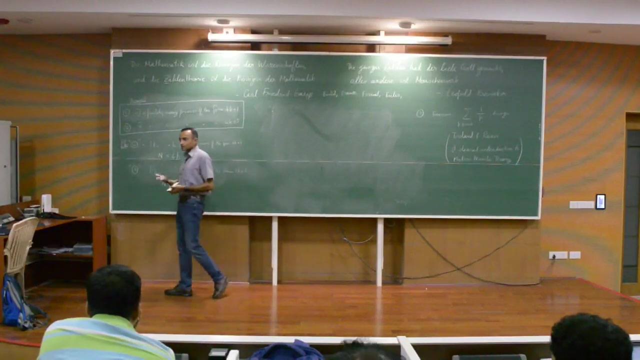 Euclid Gauls Verma. By the way, it's Verma Euler, anyone else? And now for the next one coming up is: before I mention that next name, You can ask questions. So of course, the whole point of research. 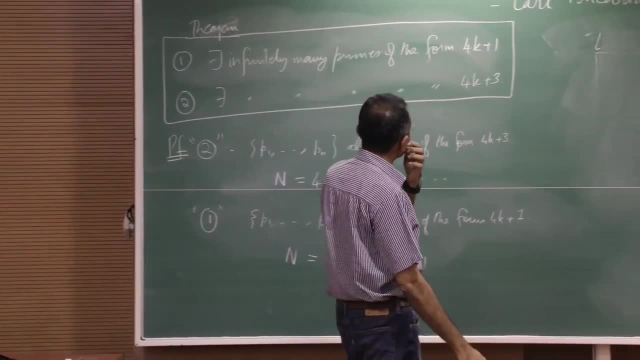 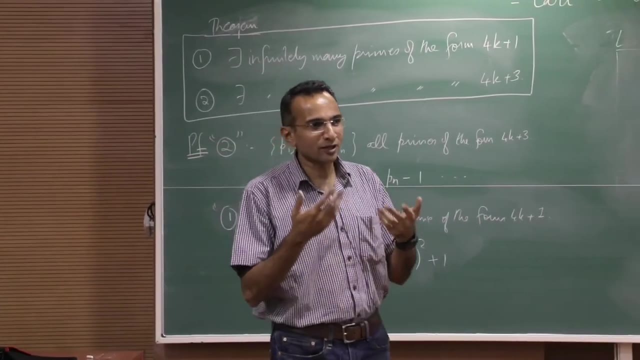 I have to say something about doing research. okay, The whole point is to keep asking questions. You ask 10 questions, quite likely, but by you I don't mean you in particular. When one asks 10 questions, it's quite likely that 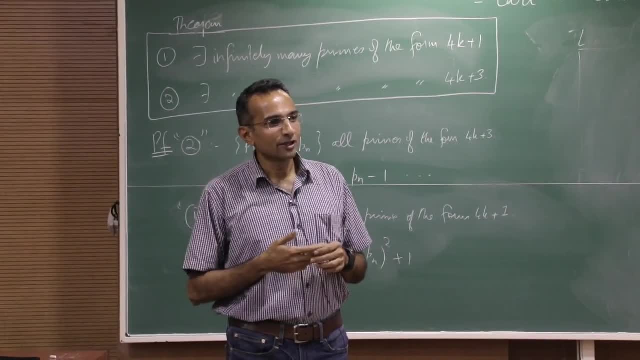 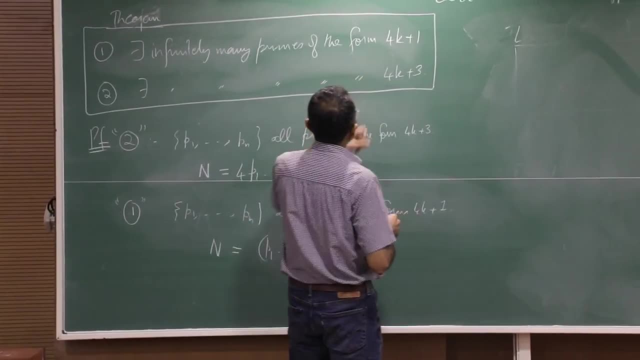 I don't know. five or six of them are just impossibly naive and stupid, which is certainly the case with me. Maybe there might be a hit here and there, meaning there's something reasonable. For example, here there are the infinitely many primes. 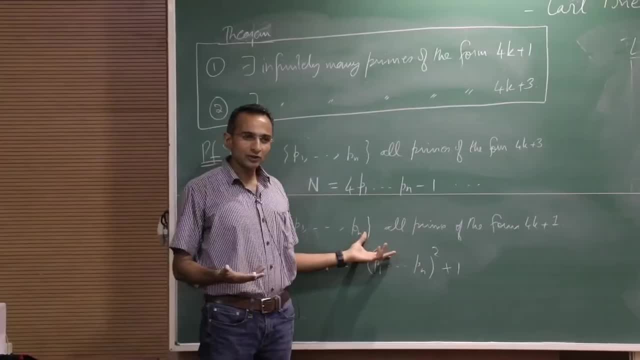 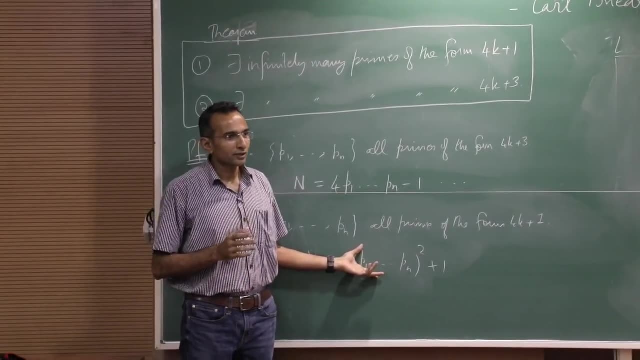 of this type, infinitely many primes of this type. It's conceivable that there are. this is a larger, larger infinity. Now, this has to be qualified. Now you know that, of course, everything is a subset of integers and that's a countable, countably infinite. 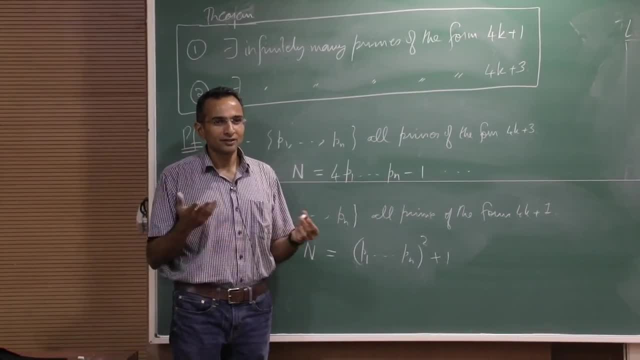 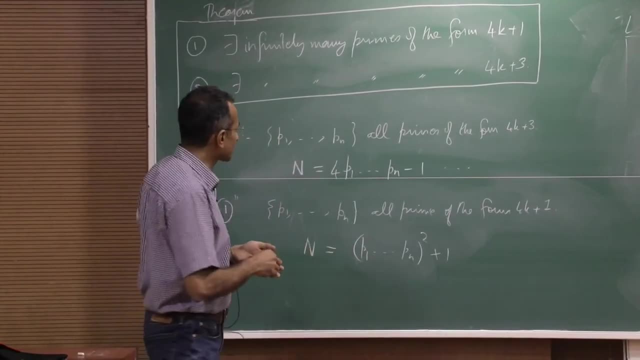 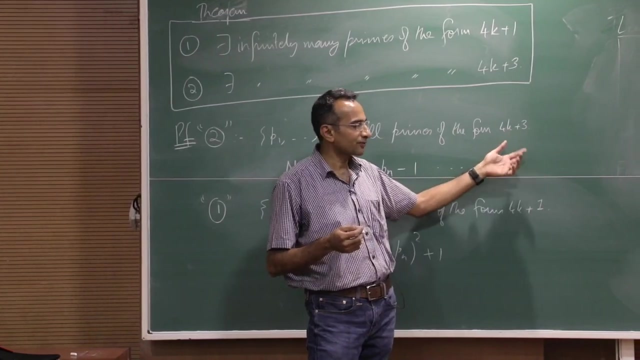 Such words make sense: Countably infinite, uncountably infinite. Some of you are not okay, So it's literally the same kind of infinity, but still in this, is it? if I throw a prime at you at random, is it is the chance, is the probability half? 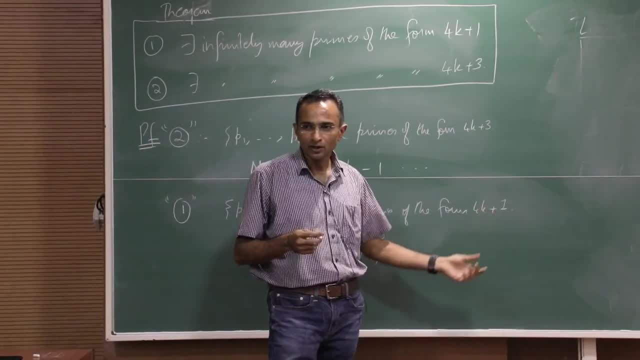 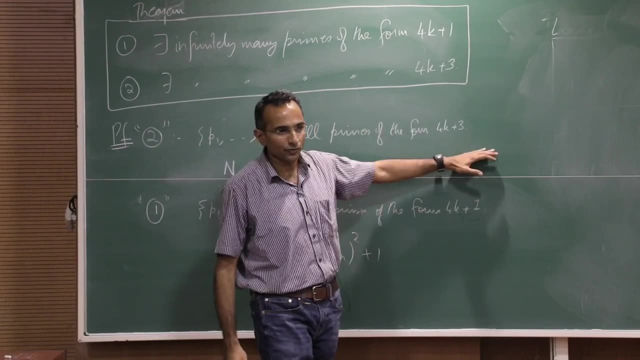 that it's of the form four k plus three, 3 and probability half of the form 4k plus 1? or is it so that maybe it's highly probable that it's 4k plus 1 and sort of less likely of the form 4k plus 3.? 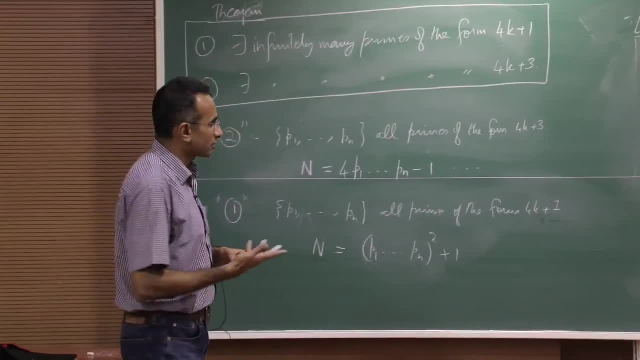 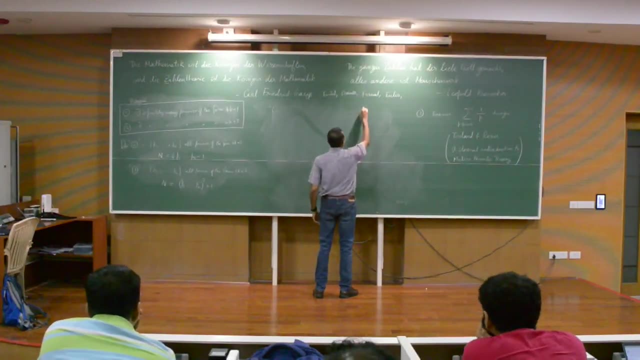 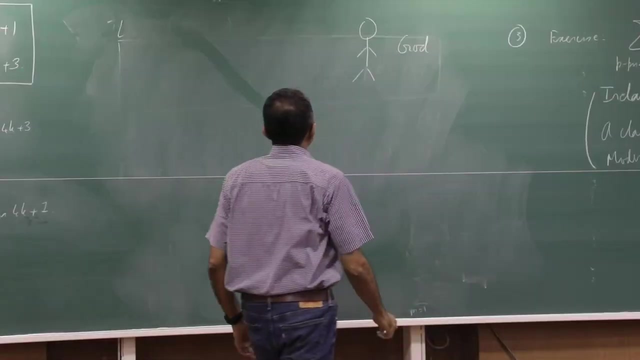 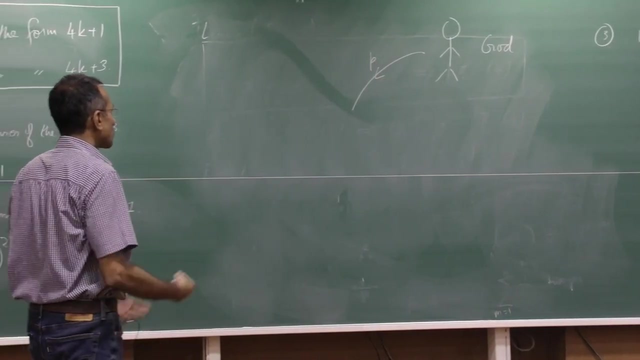 You can ask this question and you can try to formalize this. So suppose. I don't usually do this in a math talk, but it's okay. Suppose there is an entity that let's just call this God. This God throws- I mean, he's not relieving himself, he's throwing primes. 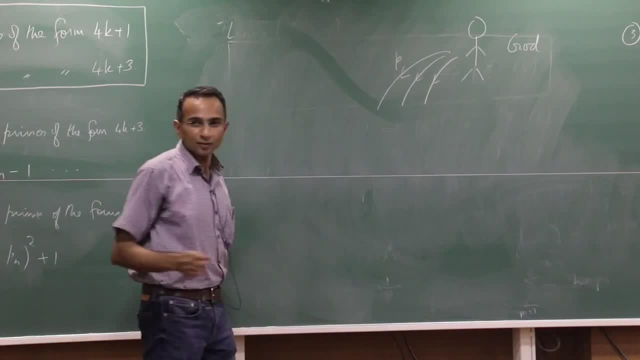 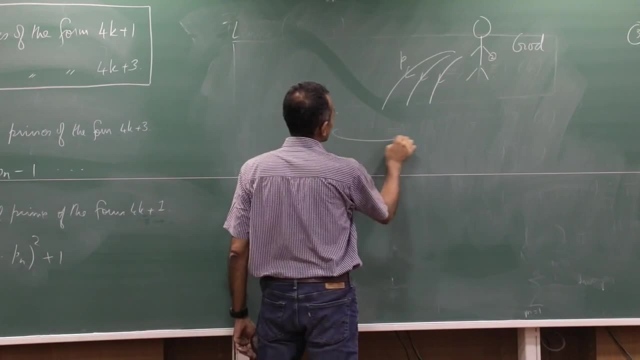 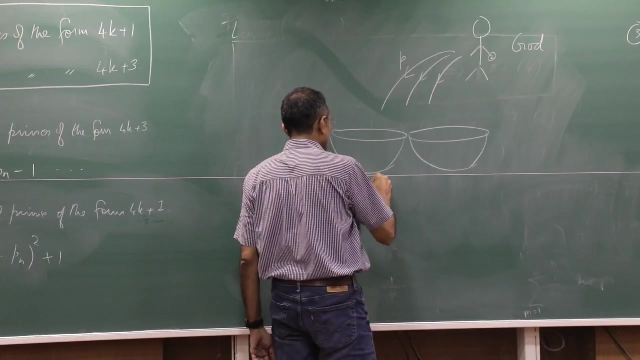 He's throwing a lot of primes other than the prime 2, which he keeps in his hand. He throws all the odd primes and we humans are trying to collect them into two buckets that we label as 4k plus 1 and 4k plus 3.. You can formalize this question a little better, Will I? as they start filling up, suppose I go up to a million and ask myself what is the fraction of primes here and of the total number of primes up to a million, and what fraction is here? 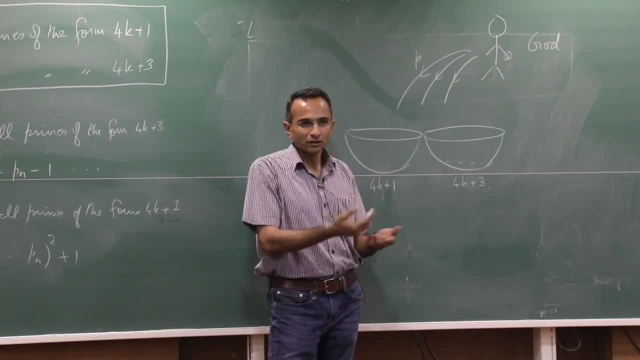 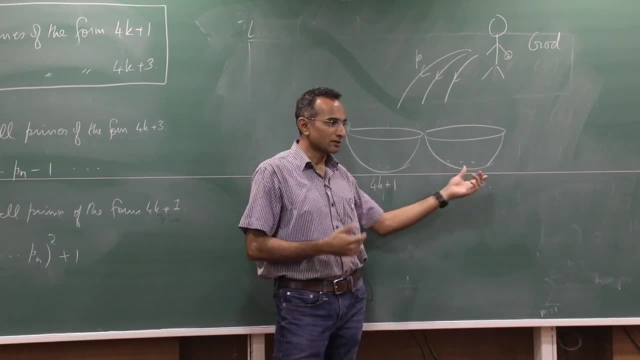 There's nothing special about million. So you go up to an integer n. take the set of all primes less than n In that, ask how many landed here and how many landed here. So those fractions will give you some kind of probabilistic statement. and what do you think is the answer? 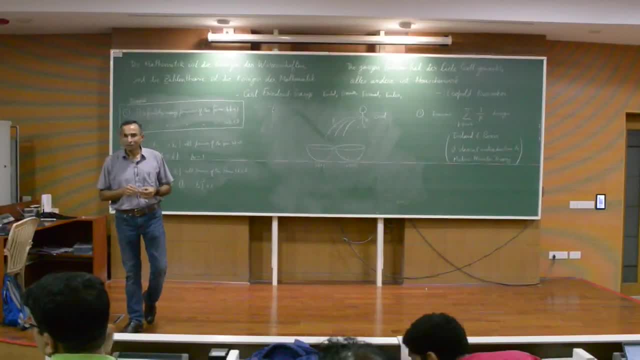 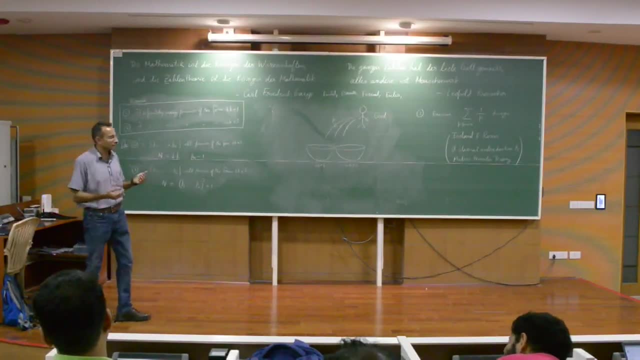 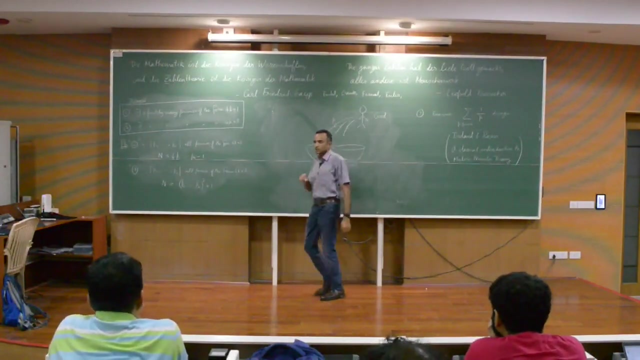 How do you know? You know this. So of course one just can say that I just have divine intuition and I just know that this is the case. So this is a deep theorem, that in fact half of the primes lie there and half will come here. 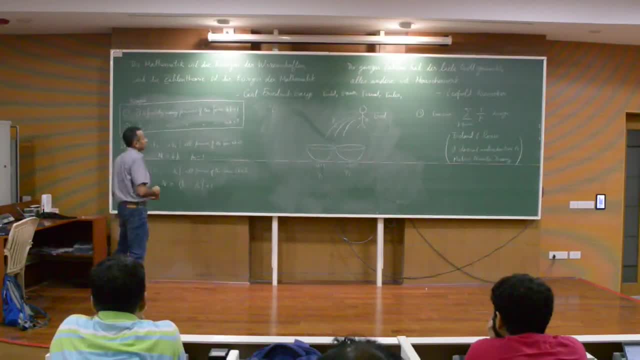 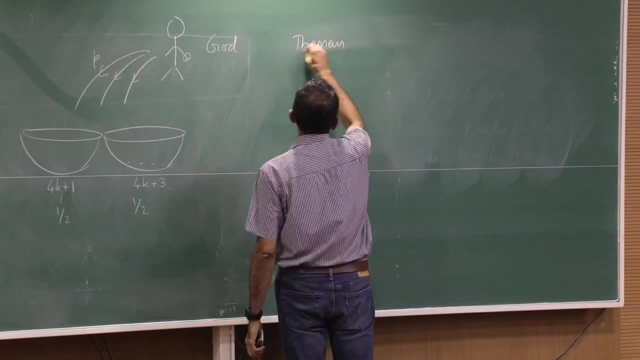 This theorem is due to another great German number theorist of that era. I want to talk about Dirichlet's theorem, But now I'm going to completely change tracks. I go back to another 14th century theorem to which, as is very popular in the current milieu, 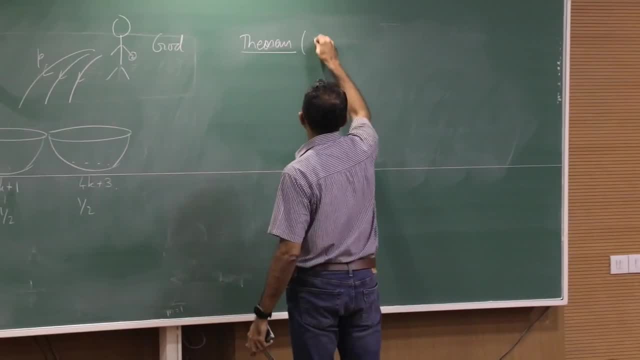 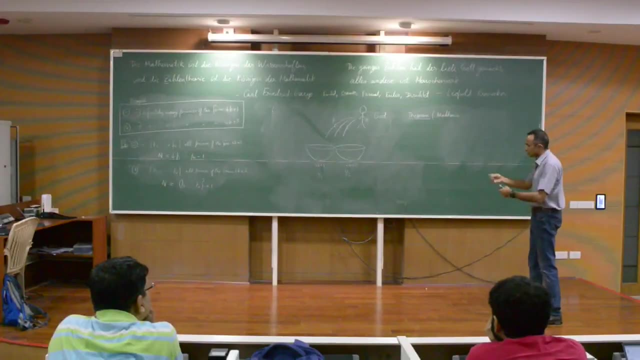 we claim everything is. the ancients knew this, But in this case there was a person by the name Madhava. not exactly clear what in particular Madhava did, but there was a Kerala School of Mathematics in 14th century. 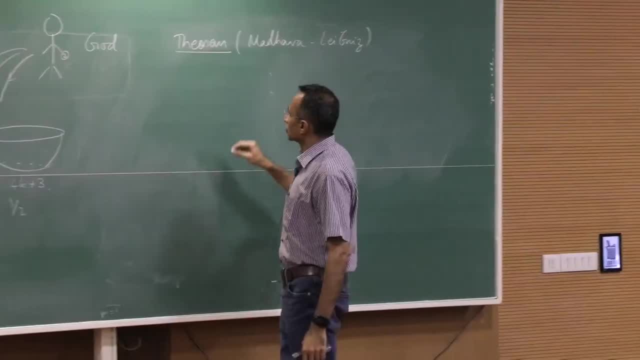 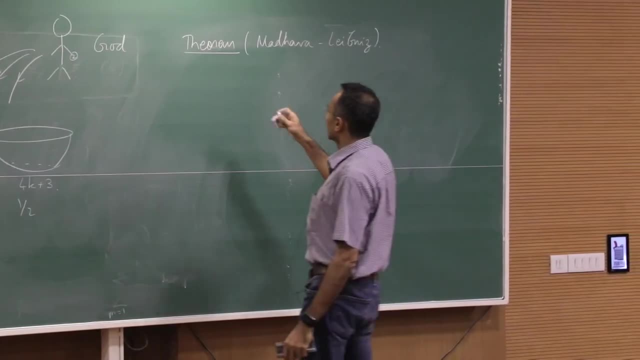 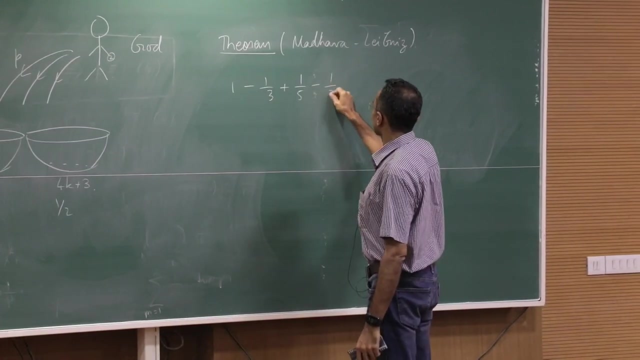 This goes back to Madhava, But in calculus books. given the Eurocentric development of knowledge, this statement is attributed to Leibniz- that if I take the alternating series of reciprocals of odd integers, positive integers, 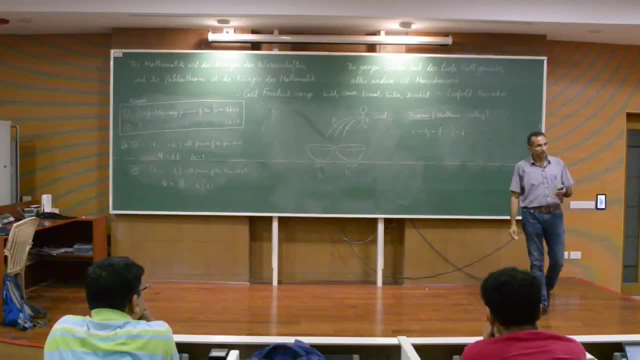 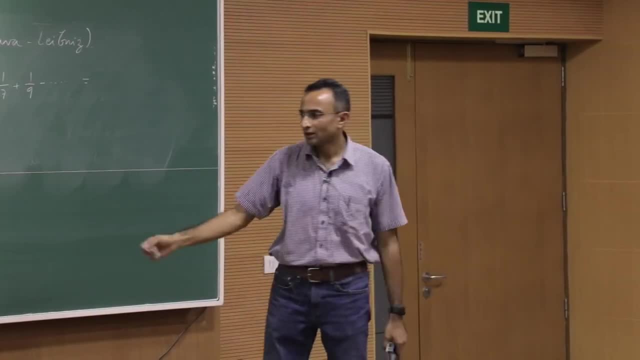 this first of all converges. that's easy. You would have seen this in a calculus courses. You can apply the alternating series test Any series with alternating terms whose in value they go to zero. you can actually hand wave a proof for it. 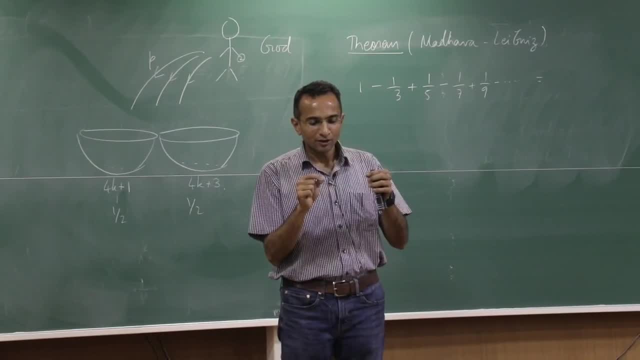 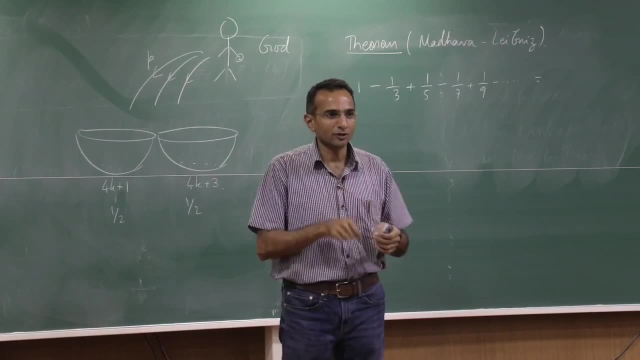 I take one, I subtract one-third, so I'll come back, and then I add one-third, but so I don't go all the way. Then I subtract something, I add something. You can literally feel that it's converging to something. 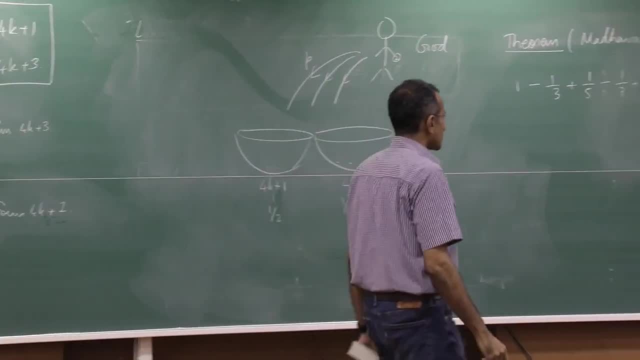 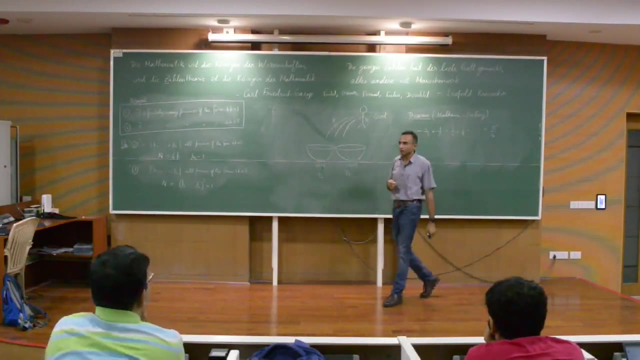 and you can make a proof out of this hand wave. So this converges, that's easy. What it converges to is interesting, and that's- oh, maybe I should have asked you if you knew this, but anyway, it converges to pi by four. 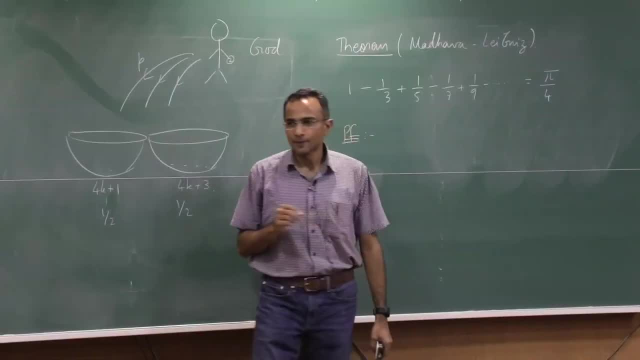 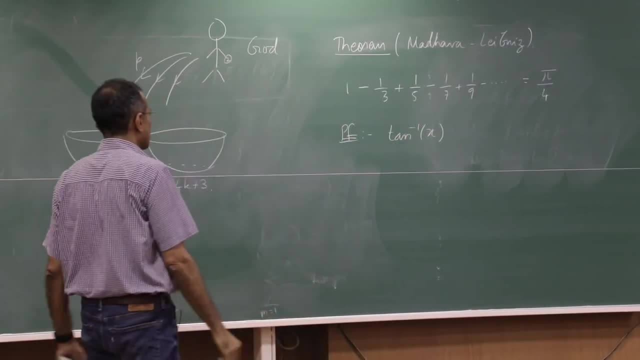 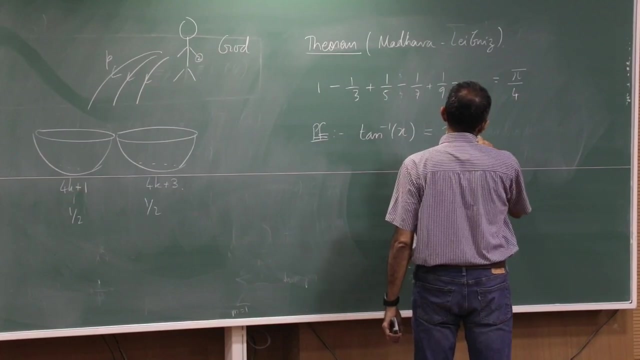 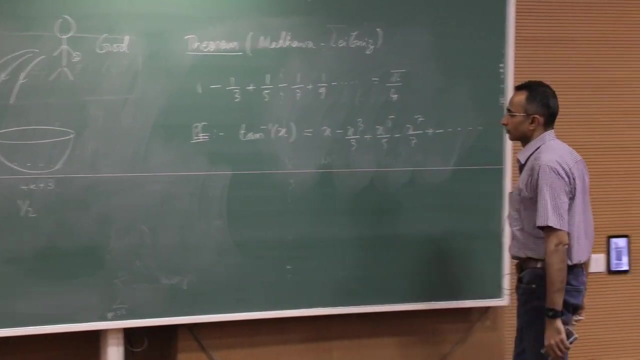 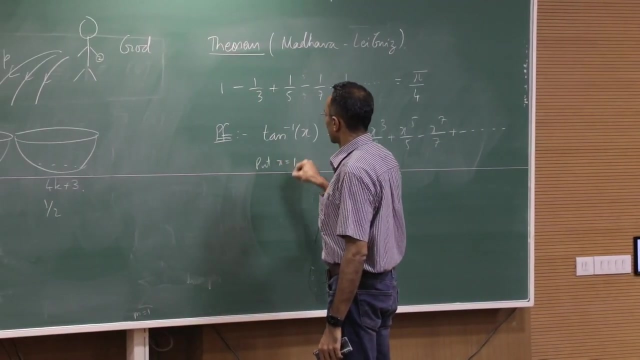 Proof? Yeah, okay, So many of you are-. so you look at tangent inverse of x, some people call it arc tan x, and you can look at this Maclaurin expansion in a neighborhood of one, And then you put: x equals one. 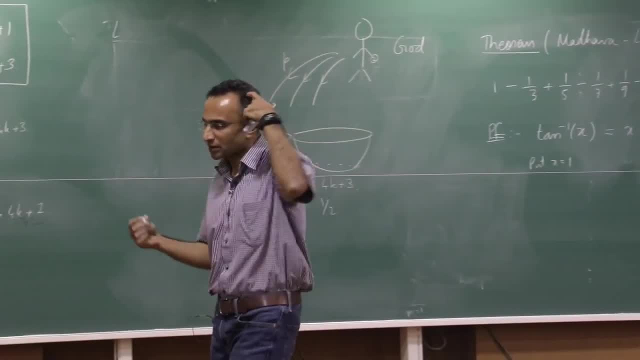 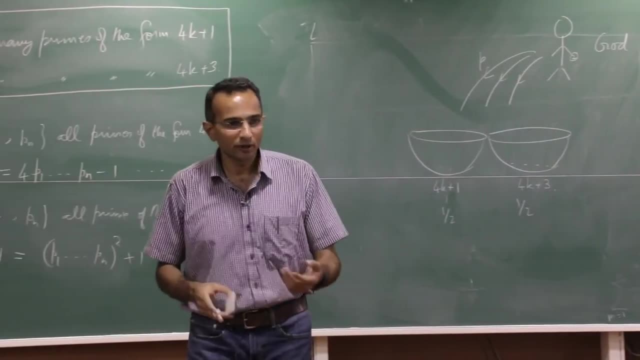 and then out pops tangent inverse one as pi by four, and on the other side you get that series. This was actually Madhava's proof, also couched in Sanskrit verses, so no one understood till very recently. There is a person in IIT Bombay, Ram Subramaniam. 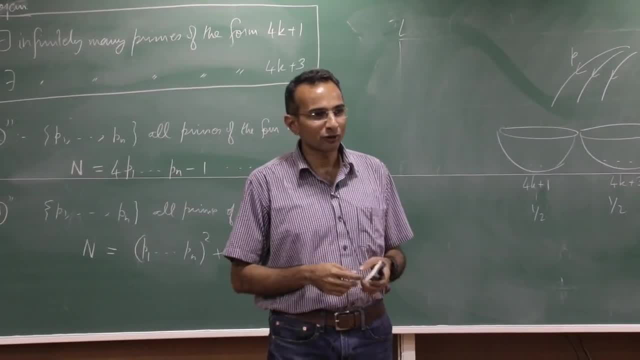 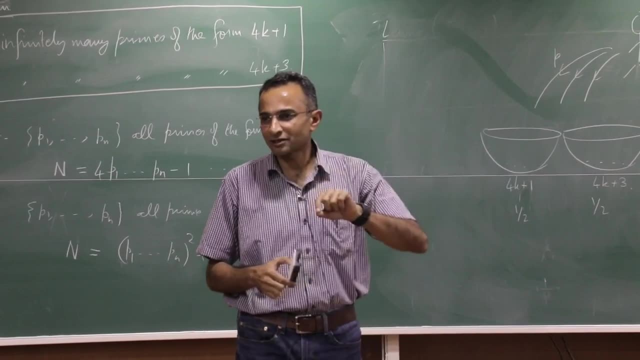 He's a bit of an expert. we have had him here give an institute colloquium. He talked about what Madhava and Kerala School of Mathematics actually knew- the Sanskrit verses and how exactly it translates- and he gave a very interesting talk on the proof of this theorem. 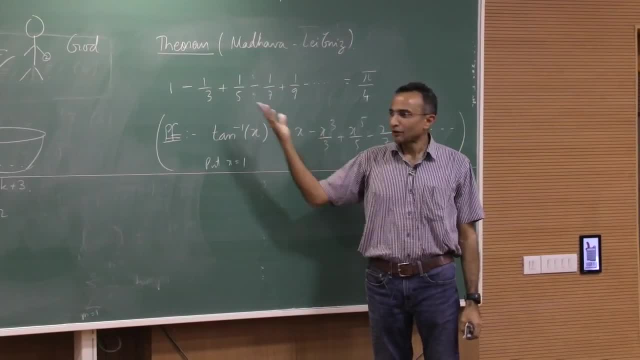 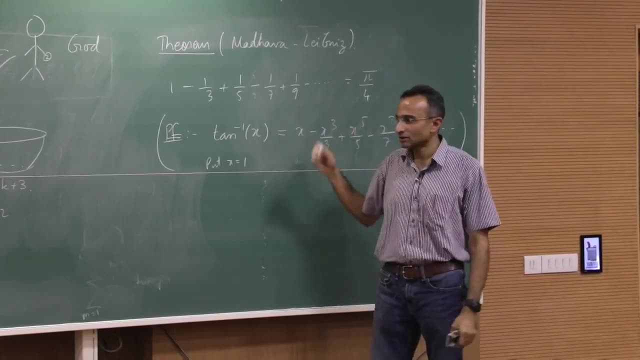 I seem to have completely changed tracks. I was talking about primes, infinitude of primes, then infinitude of primes of a certain type, and then I'm just throwing some other series here And it's- So this, I'm gonna take this off. 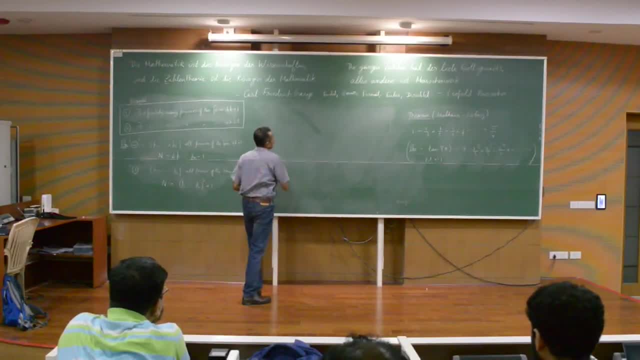 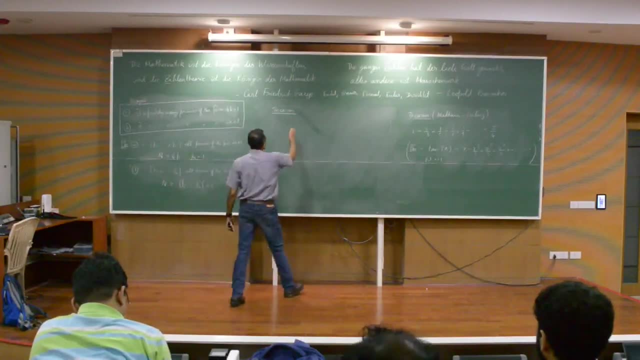 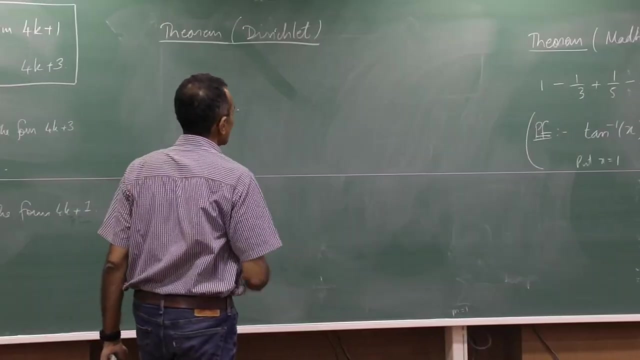 It's a great theorem in number theory which, in fact, is considered by many as one of the starting points of analytic number theory: The theorem due to Dirichlet, which states that the fact that this series- well, I don't care so much about the pi by four. 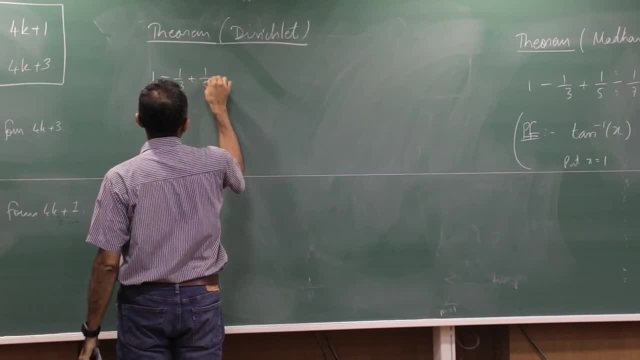 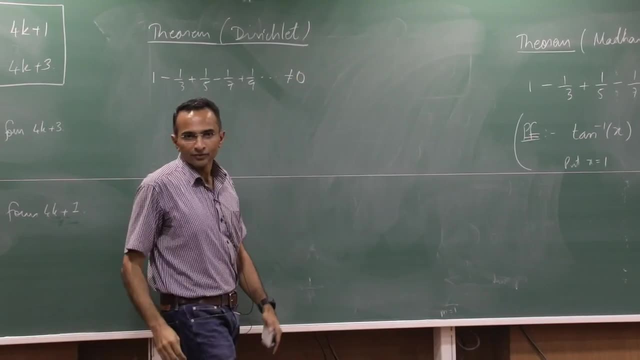 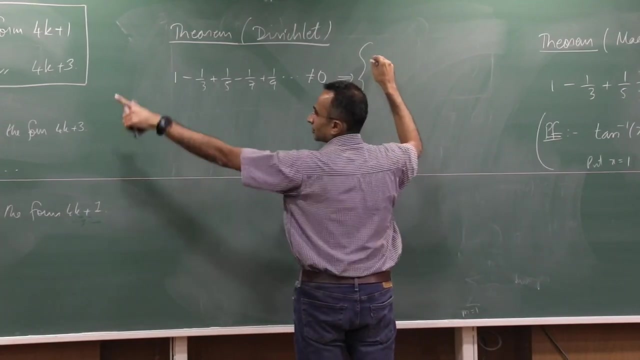 The interesting thing is that this series adds up to something which is not zero. This innocuous looking statement implies- and this is the content of Dirichlet's theorem- It implies there exists infinitely many primes of the form four k plus one. 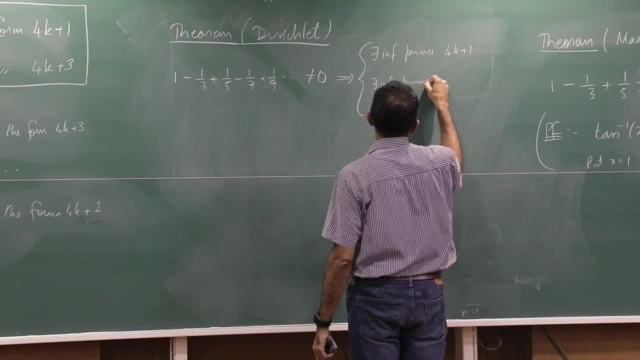 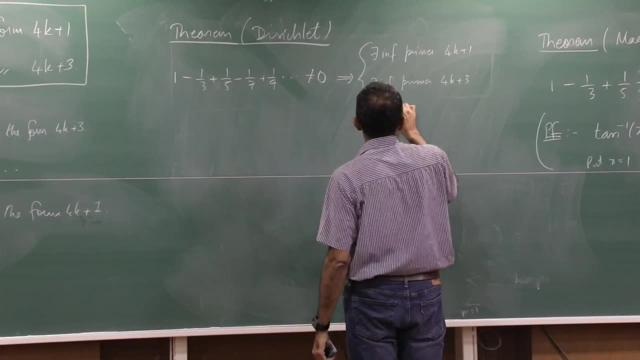 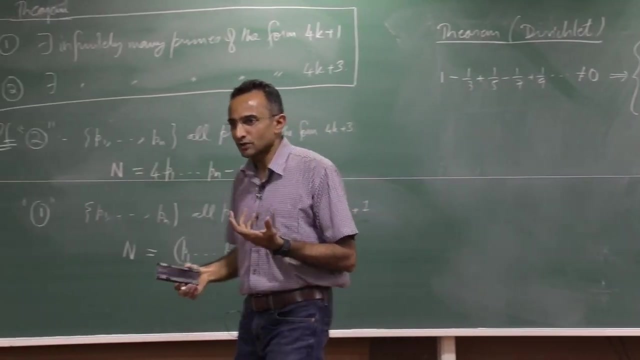 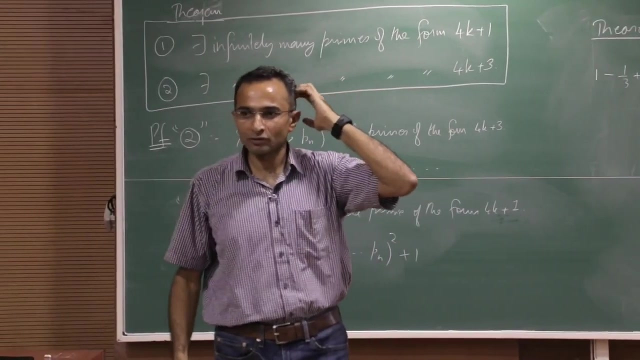 There exists infinitely many primes of the form four k plus three and in fact- and these are equal- of equal densities. half-half All of that is captured follows from non-vanishing of this particular series. This is amazing. you sit down and just stare at it. 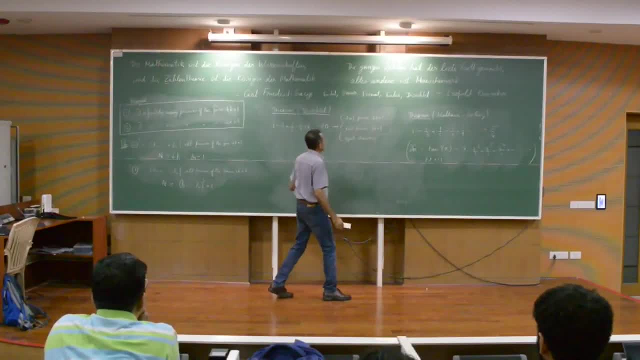 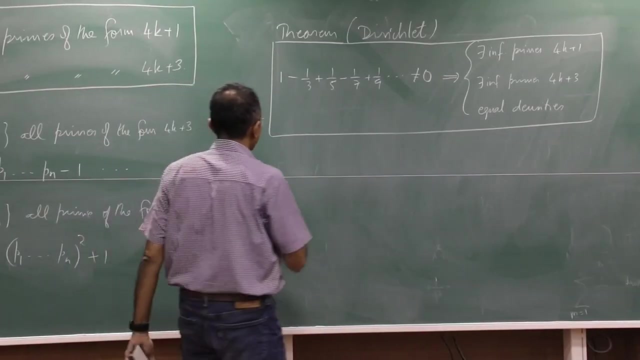 You know what is this guy got to do with. Some of you are fond of doing these reading courses. This makes- I've given you one reference- Ireland and Rosen. Ireland and Rosen's book has a proof of this theorem. Another great reference is this book by Sayre: 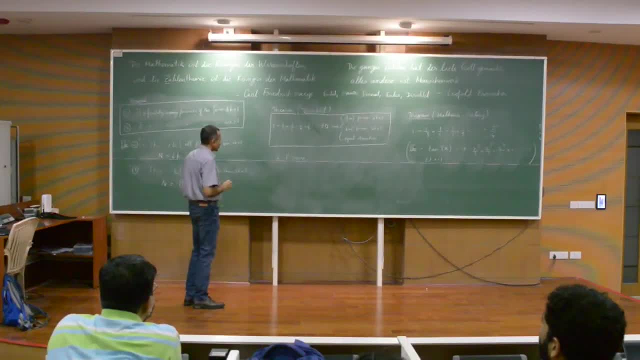 Or if you want to pretend that you know some French- which for me is, I'm certainly pretending I don't really know French- You have to say Jean-Pierre Sayre or Jean-Pierre Sayre Sayre's book. on course, in arithmetic, 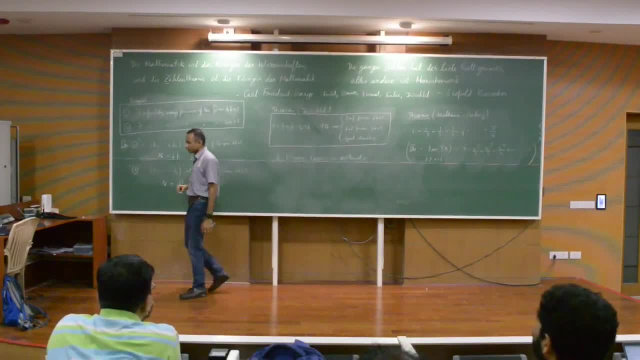 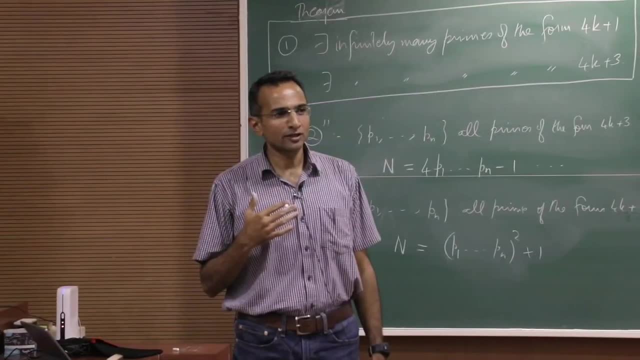 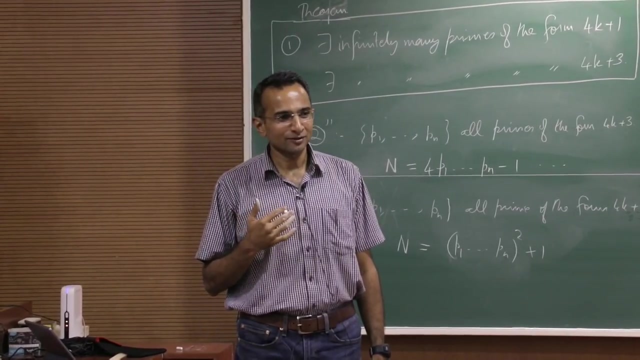 Sayre? I don't know, someone could correct me. He's probably the oldest living Fields medalist and Abel laureate. He's in his 90s. Atiya has passed away, so Sayre probably he's in his 90s. I know this for sure. 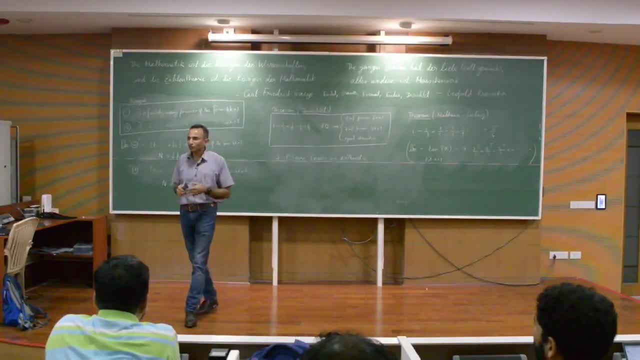 Sayre and Tate were, by the way, I mean many of you. I don't know how many of you know one of the greatest number theorists of our times passed away a few days ago: John Tate. Tate and Sayre were contemporaries. 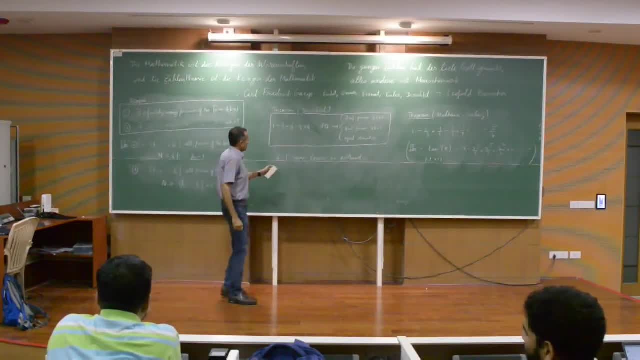 Anyway. so back to this. So this is another reference for this theorem. So I want to talk a little about the kind of philosophical content of this sort of a. how does this relate to primes of the form 4k plus one and 4k plus three? 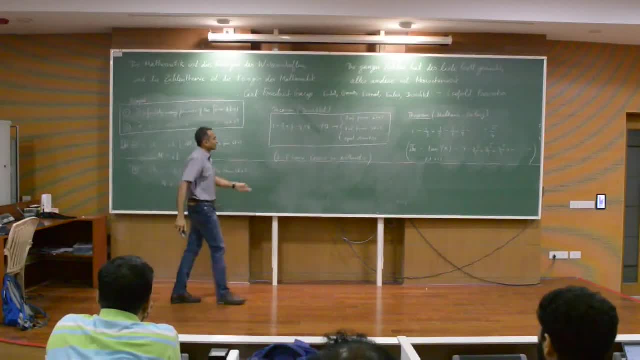 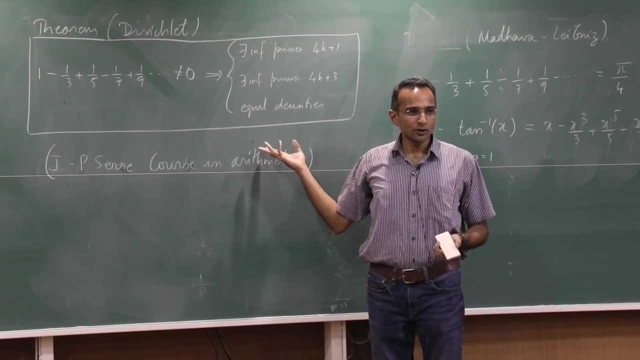 So I'll give you a little bit of what Dirichlet did. I can't give you a proof of this theorem. Yeah, what I was going to say was: this makes a fantastic one semester reading project. You can just read this by yourselves. 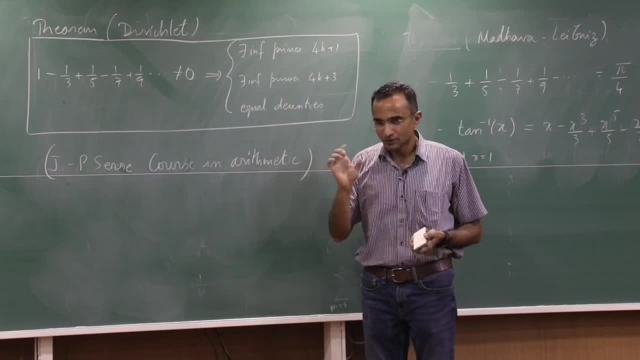 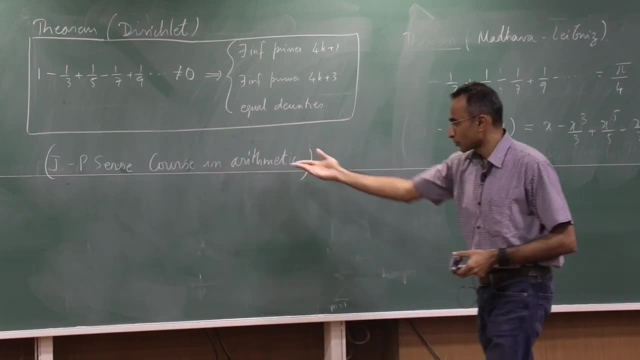 In fact, when I was a student in IT, Kanpur, the first course in analytic number theory was starting from scratch and ending with a proof of this theorem, literally, And this was one of the references. There's also a book by Apostle called 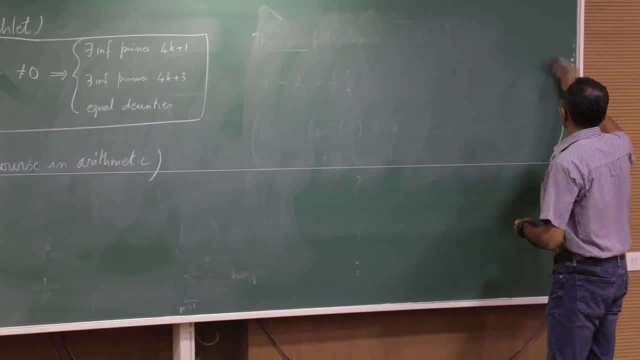 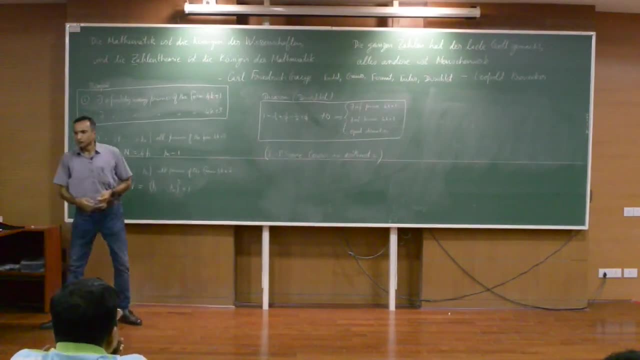 Introduction to Analytic Number Theory and that also helps. But really my favorite, and in fact favorites for many, is this book by Ireland and Rosen, Both of you who want to read some number theory. just spend the next summer, Okay, or whatever. just read through that book. 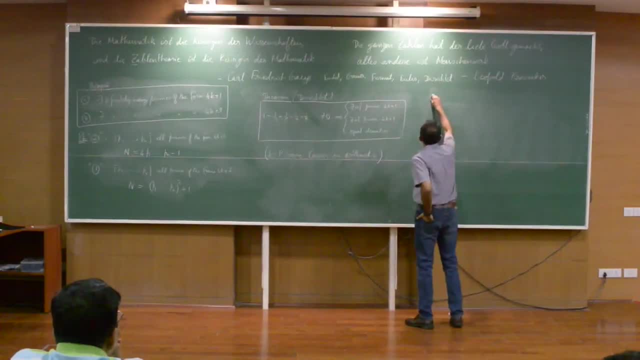 Okay. so let me give you a hint of what Dirichlet really did. So you take an integer n and you look at residue classes, modulo n. so this is notation for all integers. When I divide all the possible remainders I get upon dividing by n. there is some structure to this. 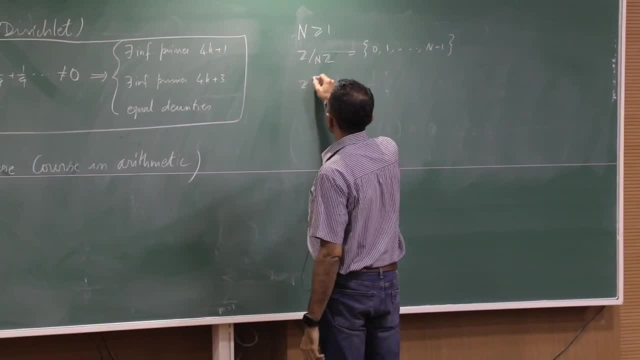 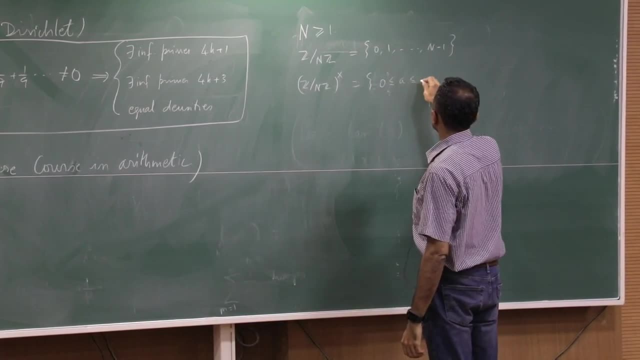 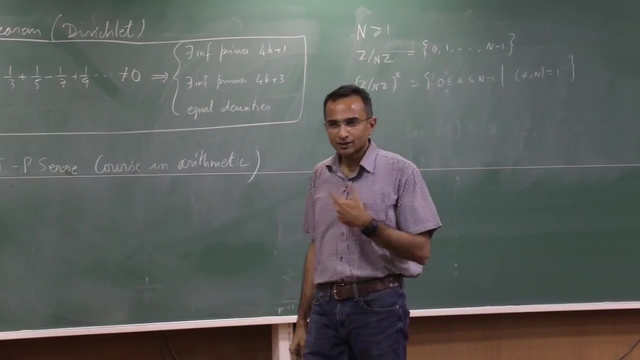 I can add and multiply. it's called a ring. I can look at those which are relatively prime to n in the set. So I look at those whose GCD with n is one. This forms a group. there is some idea of taking an inverse. 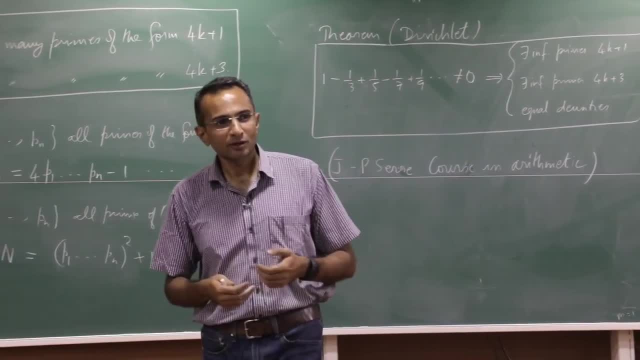 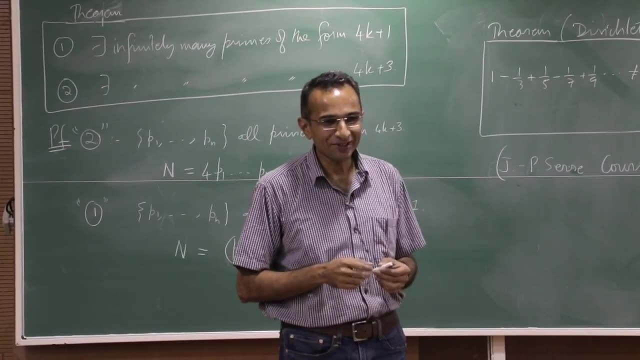 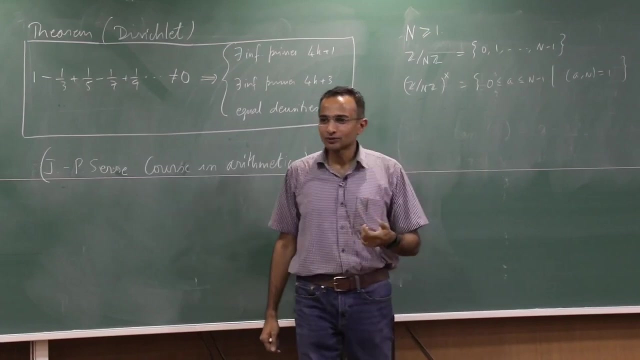 I can take n is seven. take the number two. What are the inverse of two, Three, four, four? yeah, So two times four. So I can invert the number two If I just work with integers: relatively prime to seven. 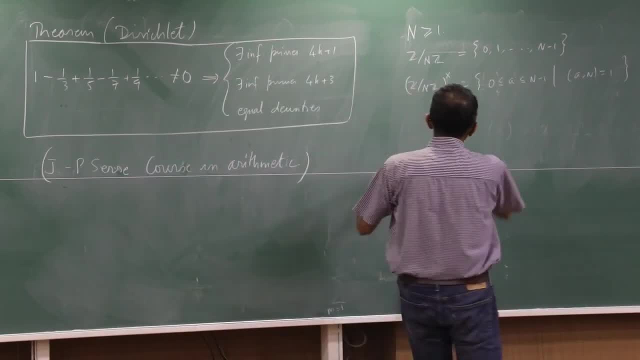 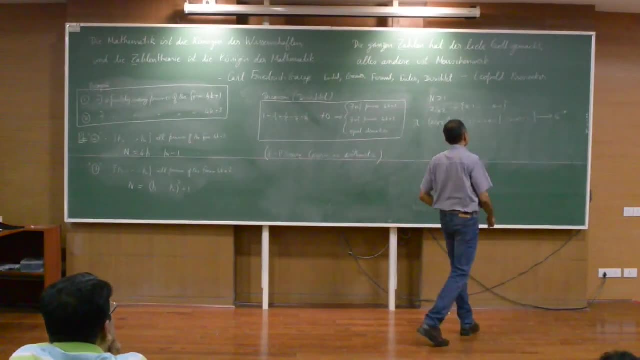 two times four is one. It's as if four is like one over two. So there is some structure to this And you take some a map from this to non-zero complex numbers. For those of you who know such words, take a homomorphism of this group. 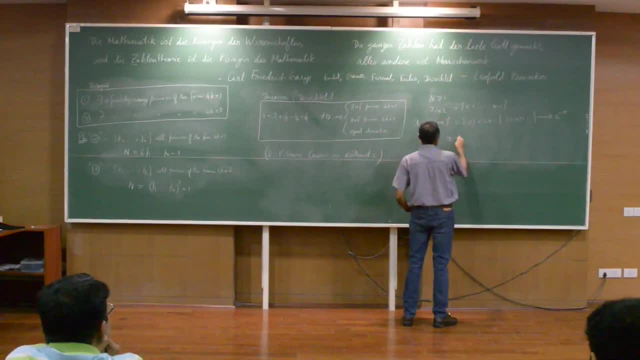 And then you inflate this to a function which I'll also denote chi on natural numbers to seven. Okay, So you can see, by defining it to be on an integer a, it is the previous chi if they were relatively prime and zero if not. 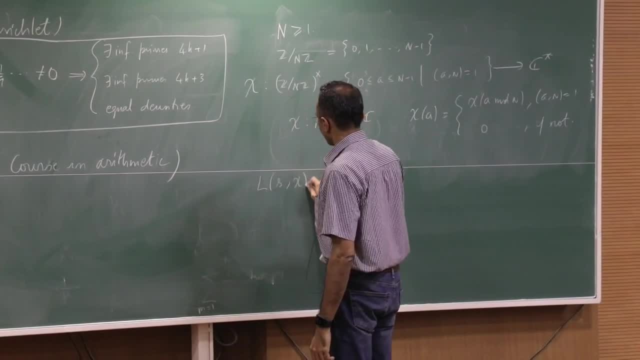 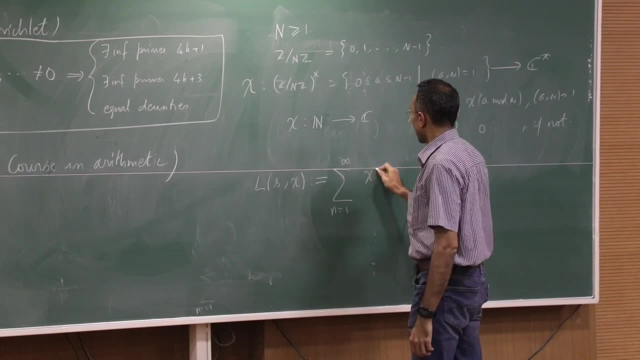 And Dirichlet studied a function and this is actually Dirichlet's notation: Ls chi is a sum from one to infinity of chi n by n to the s. And this is actually Dirichlet's notation: Ls chi is a sum from one to infinity of chi n by n to the s. 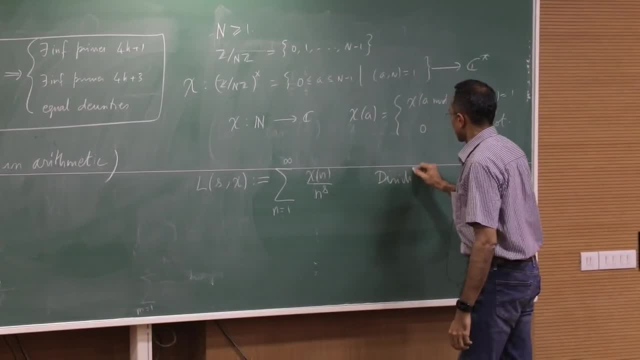 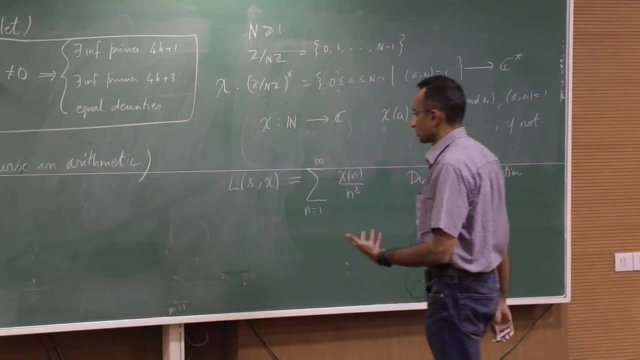 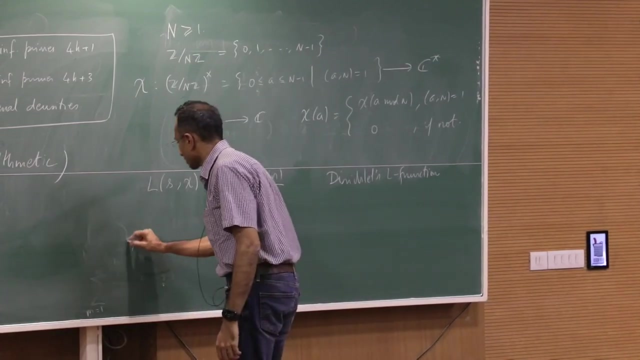 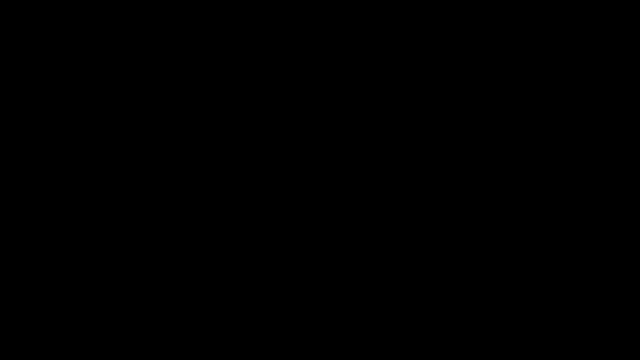 And so this is Dirichlet's L function Functions. the study of such functions is a very important part of the Langlands program, which is a big part of modern number theory And what Dirichlet really proved. so now this: I need some more board space. 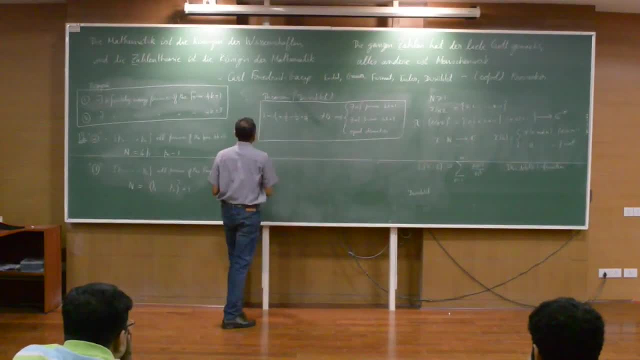 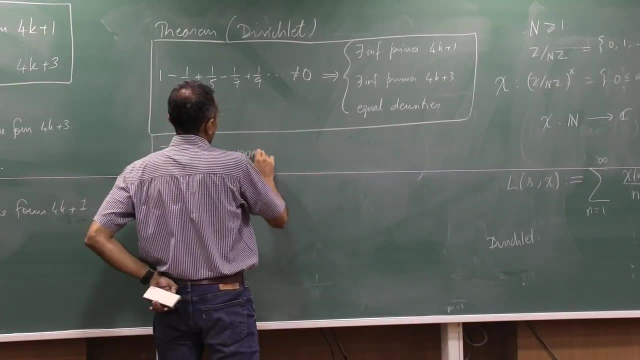 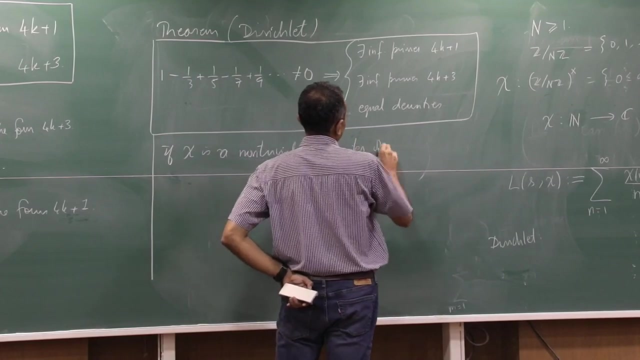 So maybe I'll put down the real theorem of Dirichlet here. So continuing: if chi is a non-trivial character, non-trivial is non-trivial such a function, we'll call it a character of z mod nz cross. 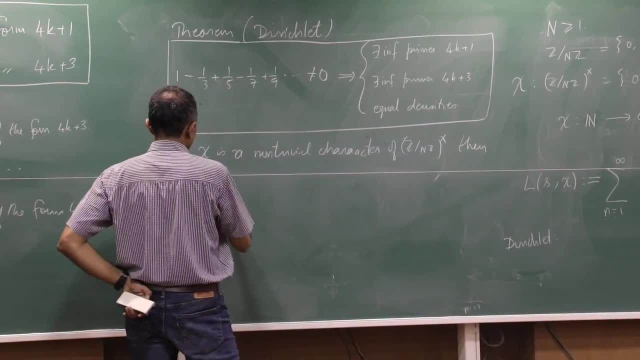 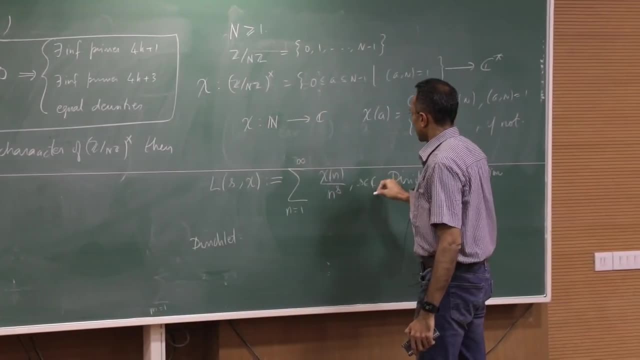 then he proved so. the first statement is: he proved that l1 chi, the value of this guy, if I put so s- is some variable. so if you put l five times l, we hopelessily substitute both of these operators for zero, because gl DONT. 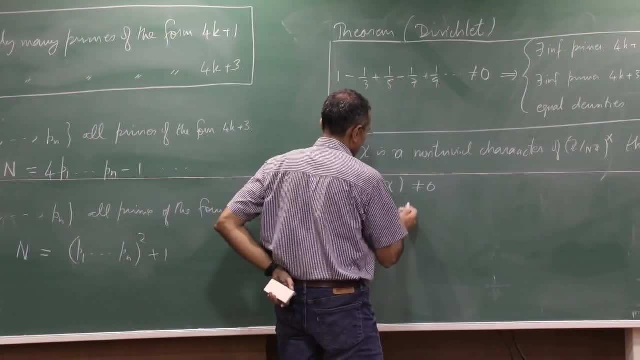 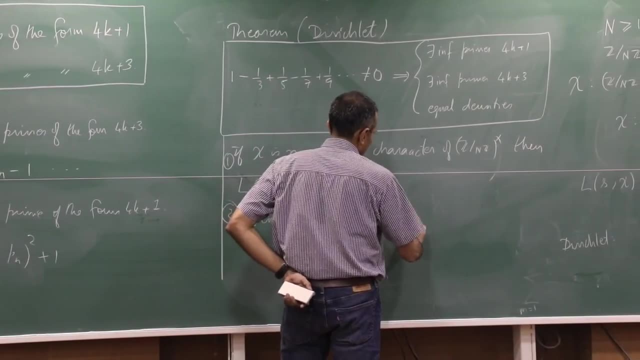 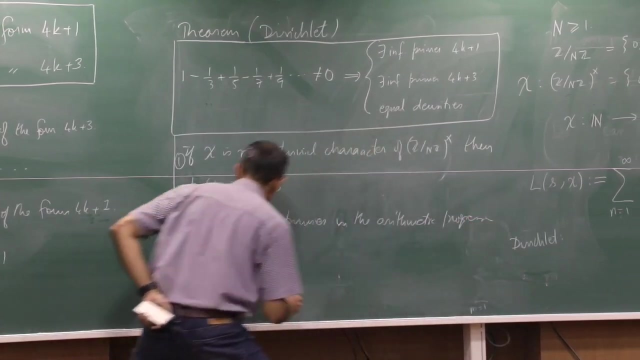 the interface is: gl doesn't give an answer. So you put the value of one, you prove that this is not zero. And then he deduced from this that there exists infinitely many primes in the arithmetic progression. In the arithmetic progression they can a. then add a plus n, a plus two, n. 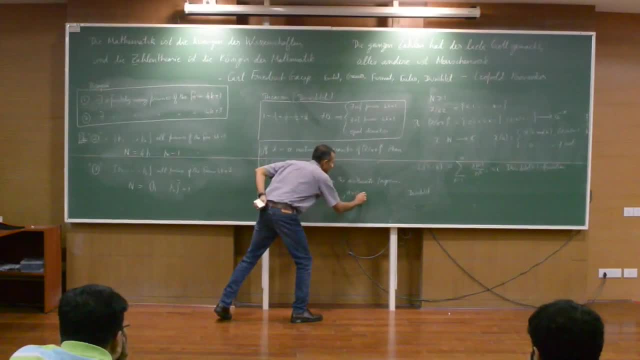 Chromium's series would be a plus k minus one times n, So this n could have been four and I could take one, one plus four, one plus eight and so on. So I'll be looking at all integers of the form one mod four. 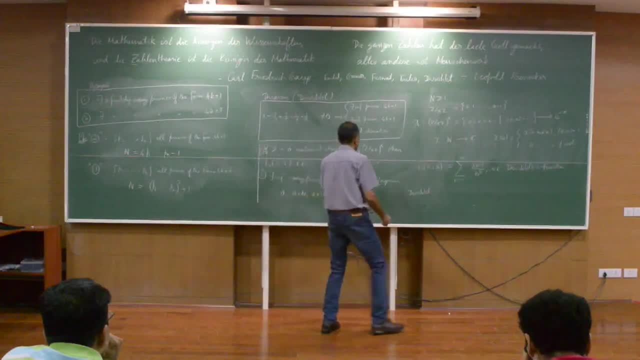 or all integers of the form three mod four. if I work with n equals four. And he proved: and this has density. the set of primes in this arithmetic progression has density, one over the number of such integers. So let me, this is standard notation. 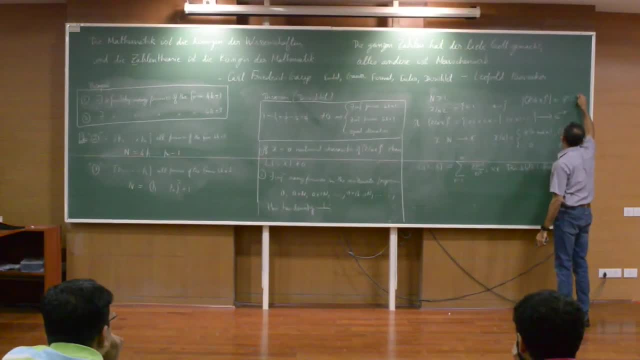 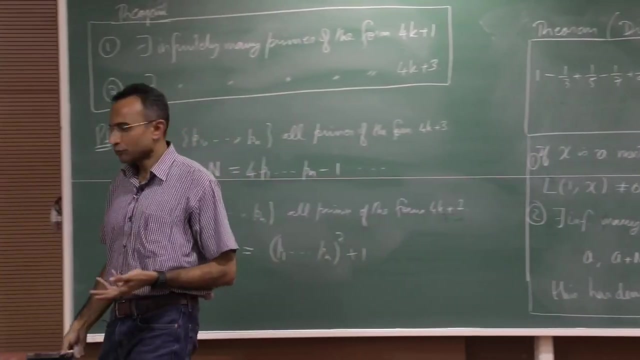 The number of integers relative to prime, to n is denoted by phi of n. This is called Euler's phi function. It's one over phi of n. So what sort of statement is this? Why do people? why do people care about it? 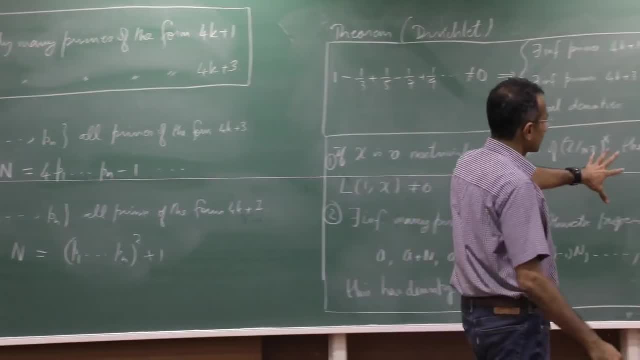 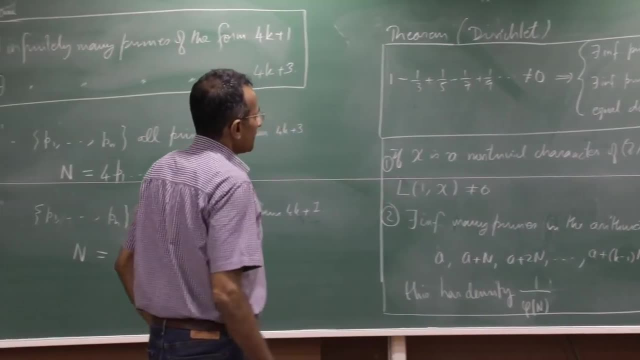 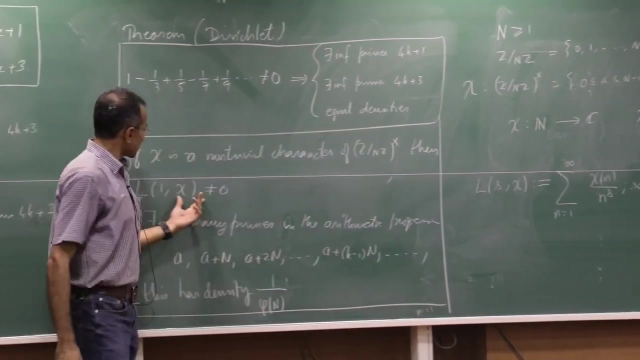 Well, what's happening is there is a certain function that he very cleverly cooked up in some very it just came out of the blue this thinking, And this is a function of a complex variable. It's some purely analytic property of this function. 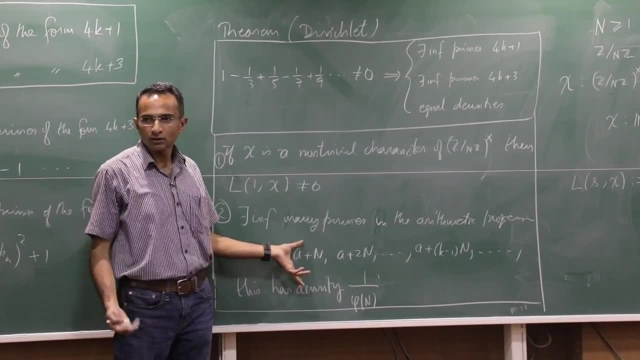 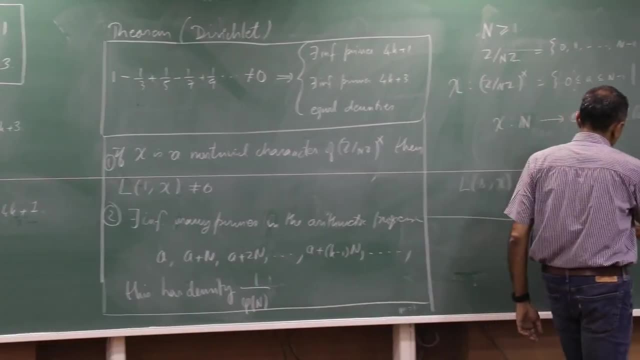 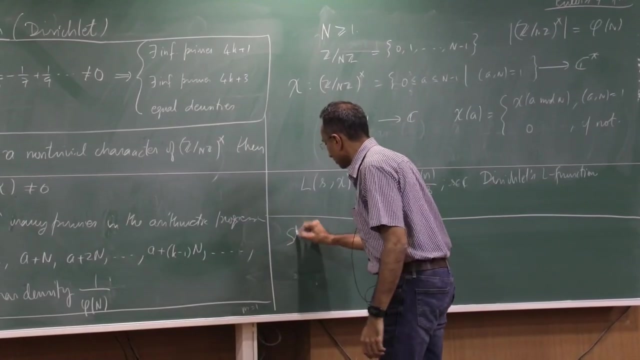 is capturing some kind of deep arithmetic of amongst numbers and amongst primes and so on. There's an entire area of mathematics now devoted to understanding these kind of things. So this value of one of an L function is a special value and the subject is special values of L functions. 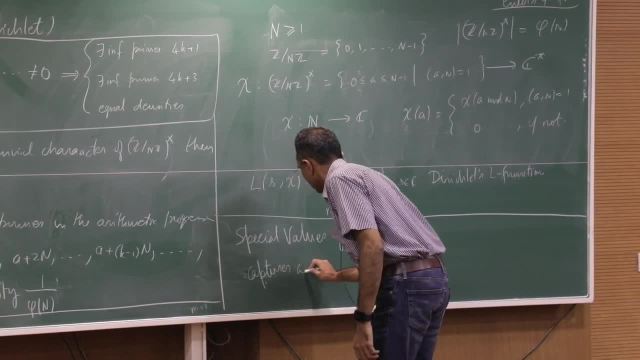 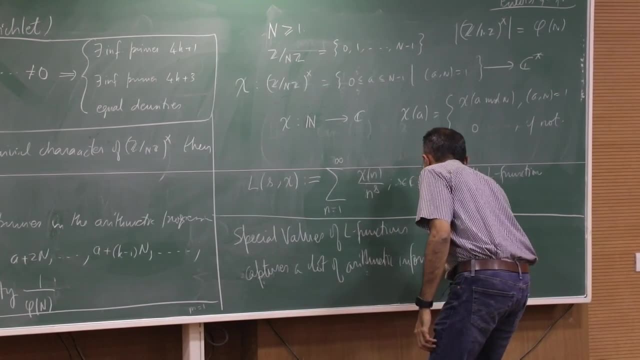 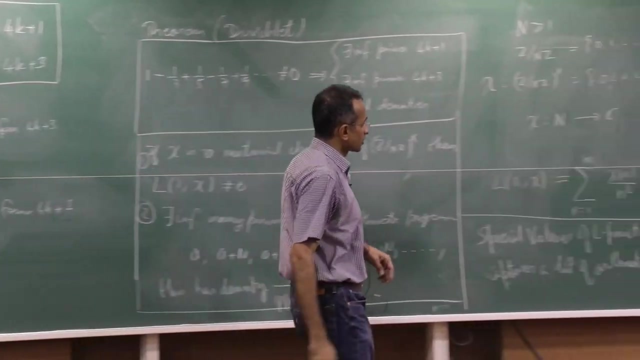 Captures a lot of arithmetic, So my own research is in this area. There are all kinds of L functions. Instead of looking at Dirichlet characters, you can. an arbitrary L function is some series of that type for some sequence: a, n. 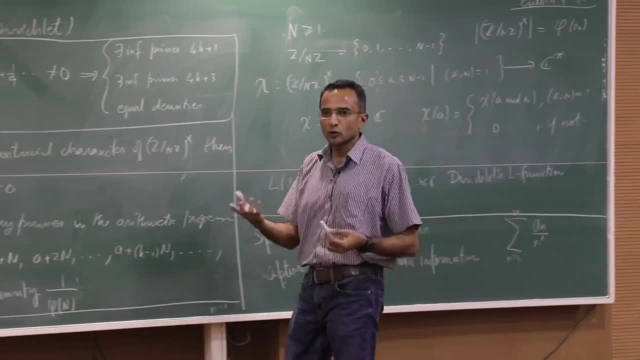 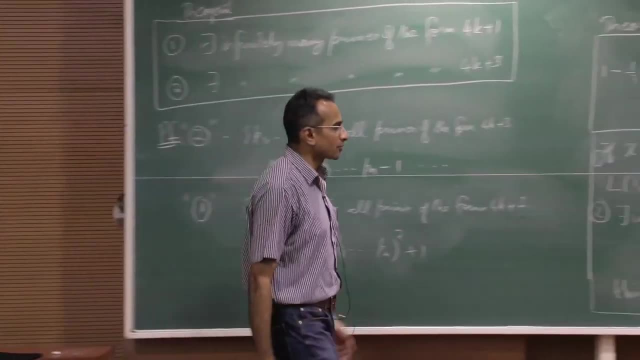 And this sequence, a, n might be coming out of some other. maybe there's some geometric problem, Maybe there's a Diophantin equation and I'm looking at solutions of this Diophantin equation. You know mod, prime powers, or I can put together those things and that L function. 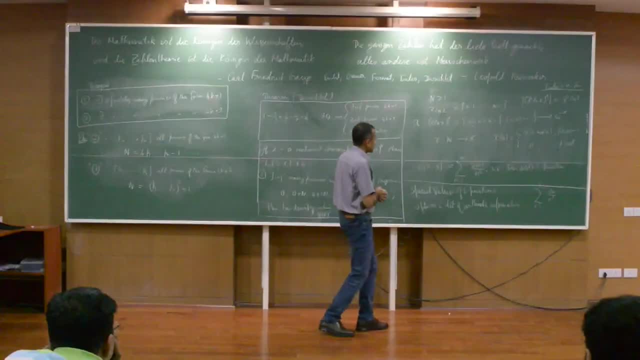 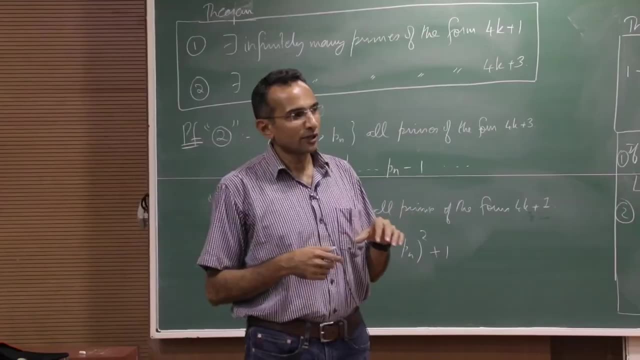 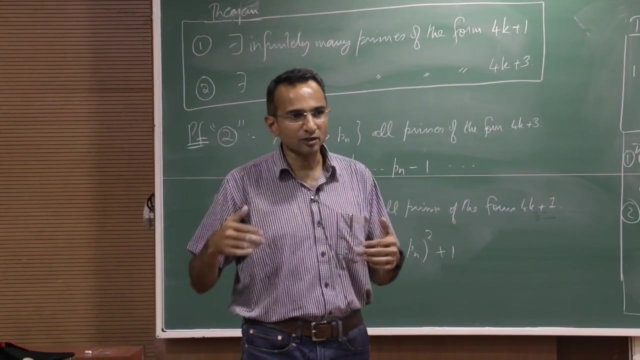 is called the Hasse-Weil Zeta function. There are the Langlands program. The Langlands program is many people consider is like some kind of big unifying theme in modern mathematics, Because it just conjecturally produces a lot of bridges between seemingly disparate areas of mathematics. 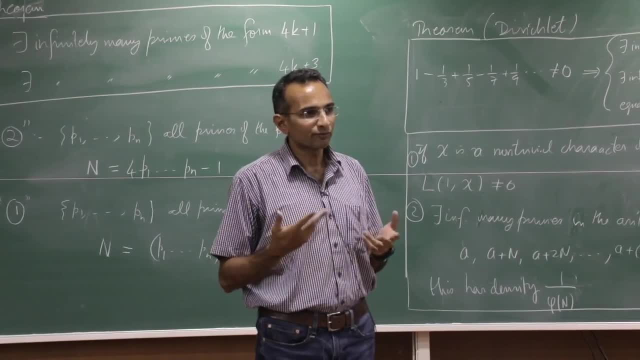 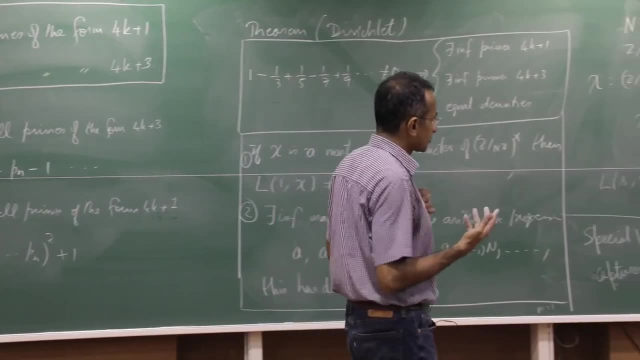 and the bridges, and you might have heard of Andrew Wiles' great work or one of the few theorems which made it into the first page of New York Times When he proved Fermat's Last Theorem, which was an instance of the Langlands program. 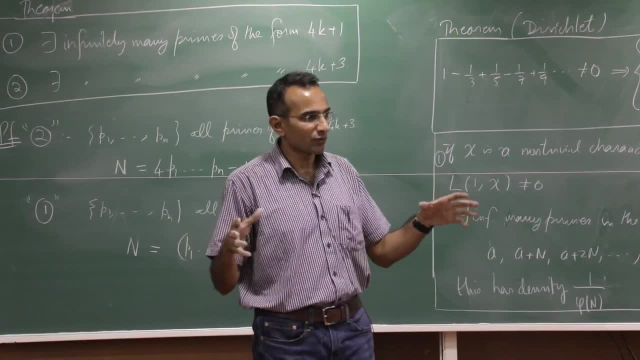 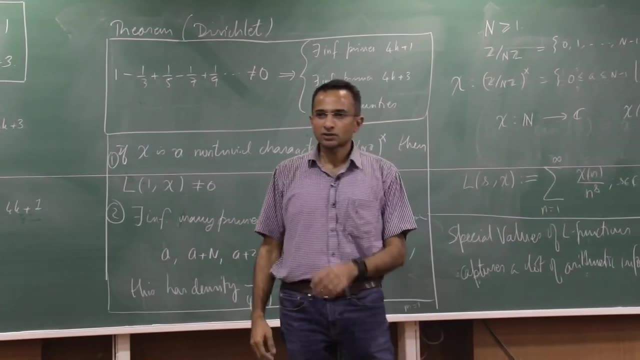 that there is some bridge between the world of ellipticals and world of modular forms, whatever these words mean. And all these bridges in the Langlands program are mitigated by some idea of these kind of functions, This world of mathematics. you can construct some functions of this type. 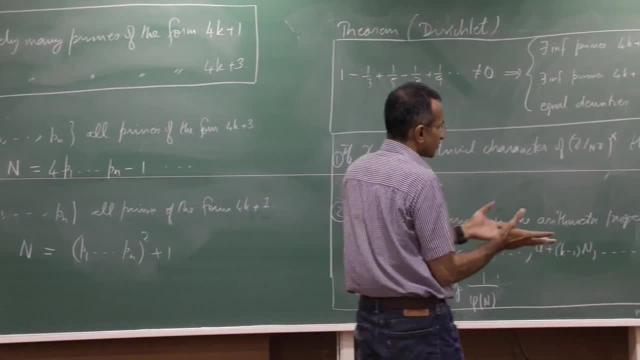 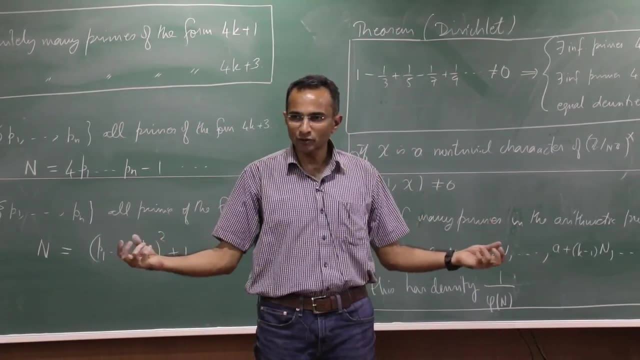 Some other world, completely different looking world. you can construct L functions of this type and this bridge is mitigated by an object here and an object here. These two L functions are the same. Therefore there is some relation between these objects, even though directly you cannot produce a relation. 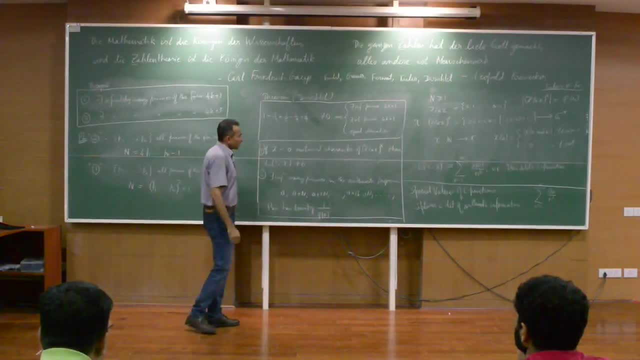 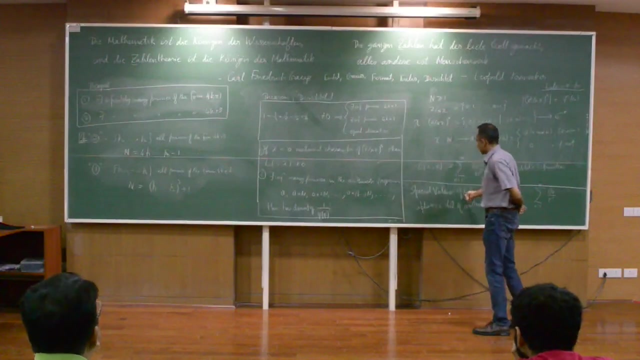 So Andrew Wiles' theorem is of that type. So these kind of the study of these L functions form a big part of modern mathematics of that type- number theory going into Langlands program- And the principle is values of these functions at some very special points. 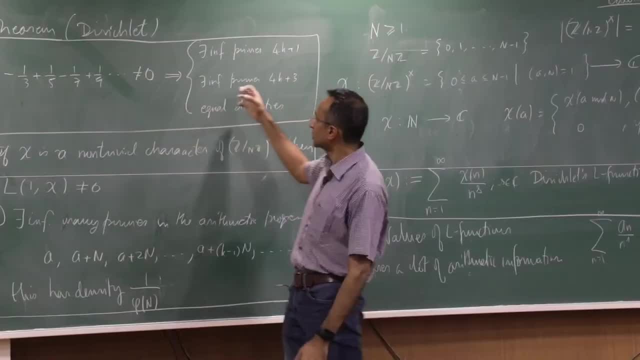 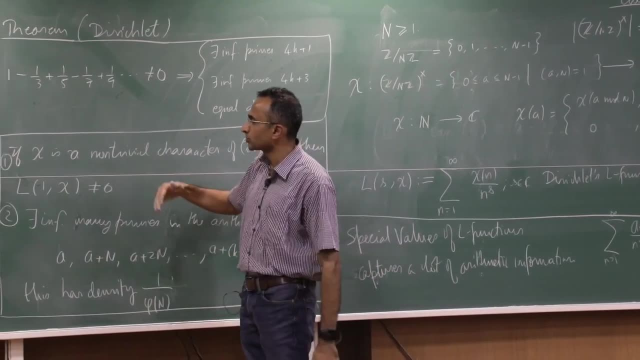 it might look like some innocuous. like this, Madhva Leibniz series actually captures some very deep arithmetic. But juicing out this information is the hard work. There actually are different kinds of problems. One is simply to have some reasonable statements like this: 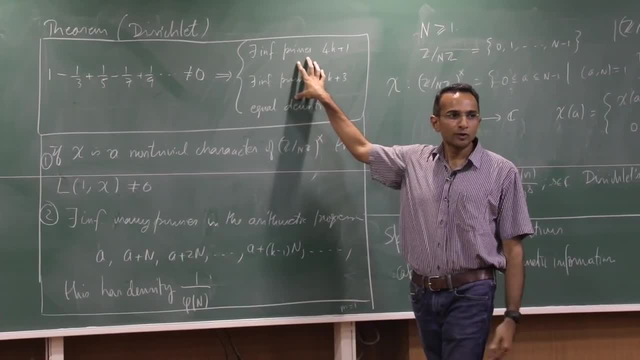 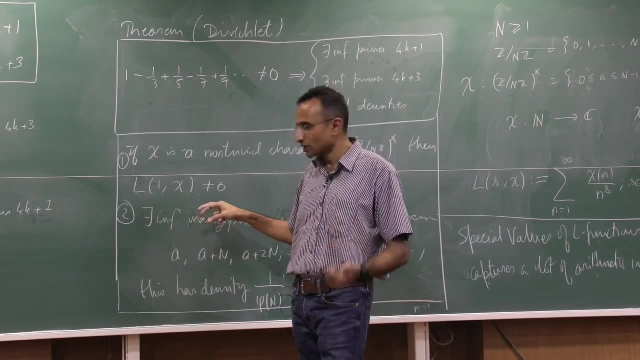 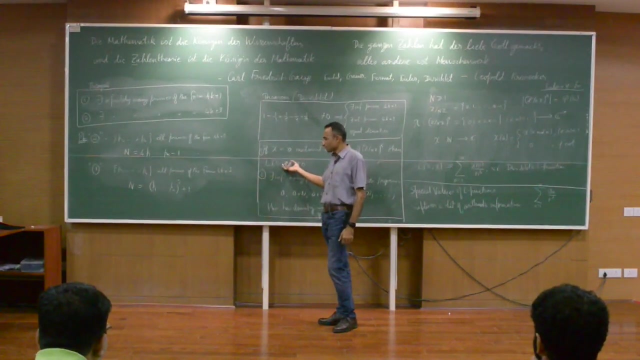 and then to juice out arithmetic. The big names to mention are well, Pierre Deligne, who is also one of the few Fields Medalists ever laureates. He has this way of thinking about these kind of special values of L functions and gives you some kind of framework of thought. 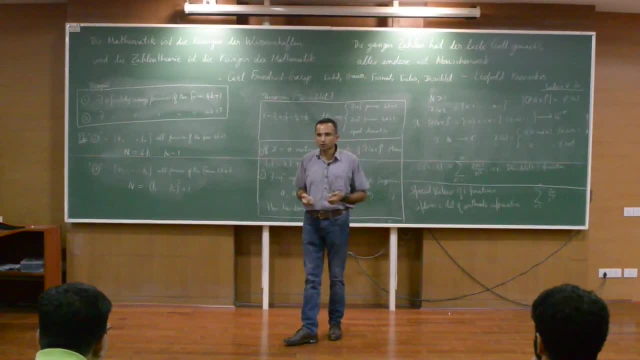 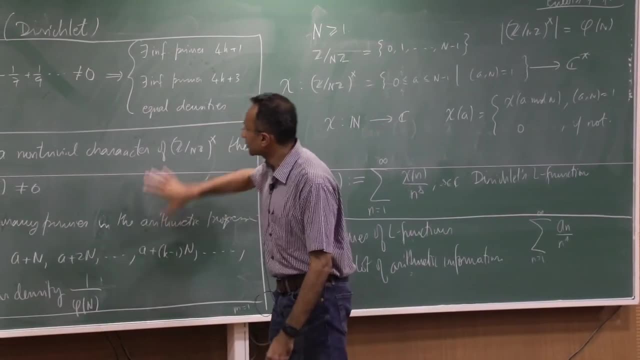 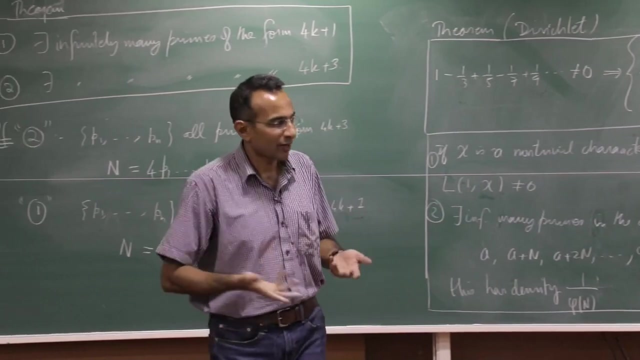 What should you expect? Okay, you can look up Deligne's conjecture on what are called motivical functions, Deligne's conjecture on motivical functions. And then what sort of arithmetic is embedded? That's a different story. That's, I don't know, in this talk. maybe it's kind of. 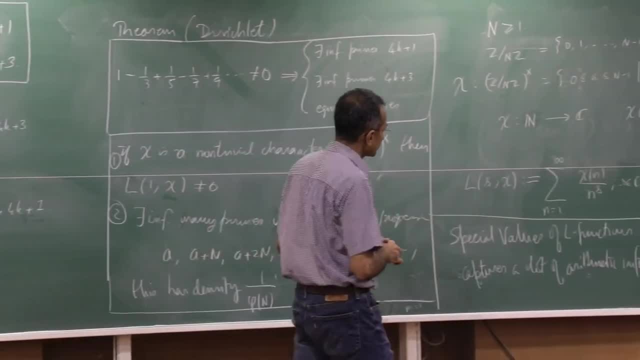 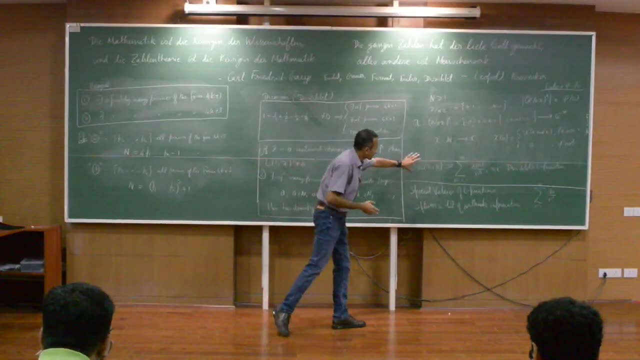 I'll be just throwing words and names. So again, the take home message, I guess, is the function that Dirichlet constructed is an early instance of an entire family of L functions which is prevalent in modern number theory, And people try to understand the values. 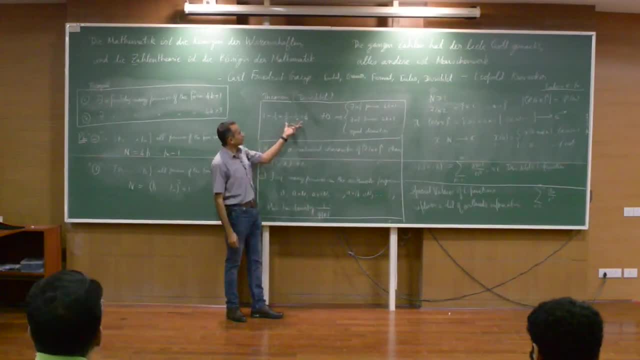 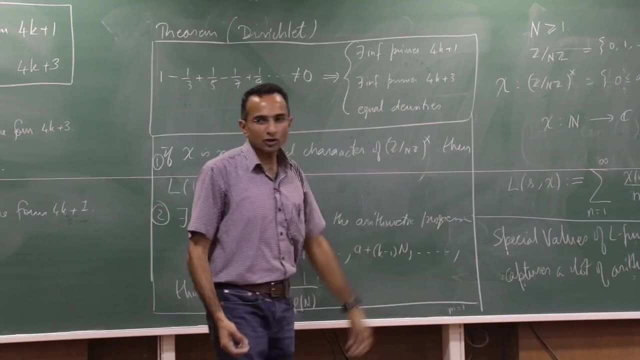 of these L functions at various points. In this case it boils down to, in the classical scenario, it boils down to some series like this Madhava-Leibniz series, And then one wants to juice out arithmetic information in that special value. 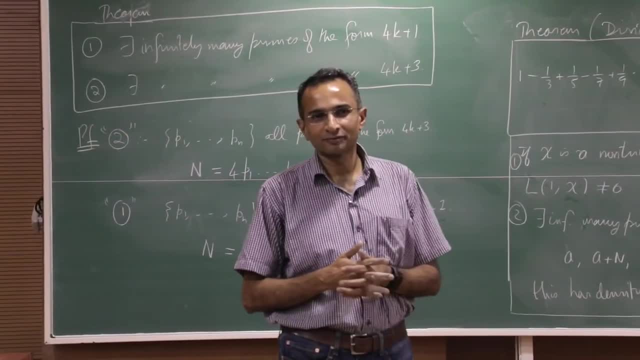 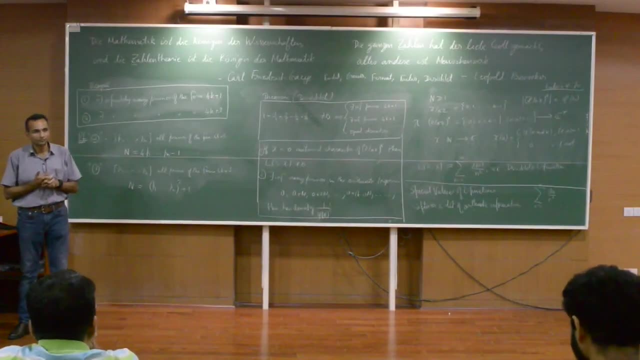 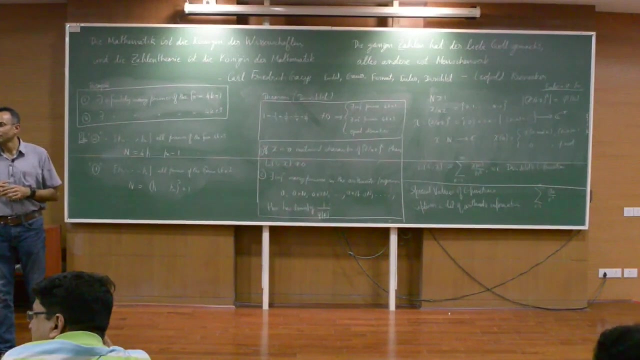 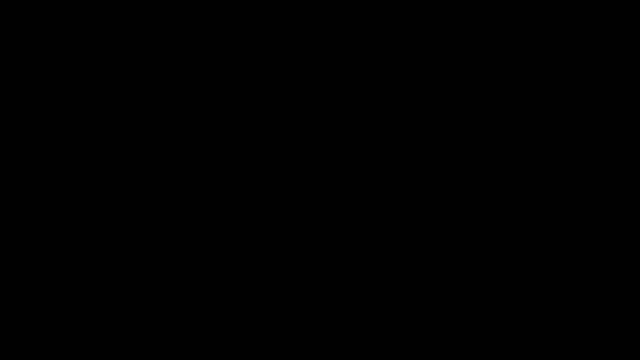 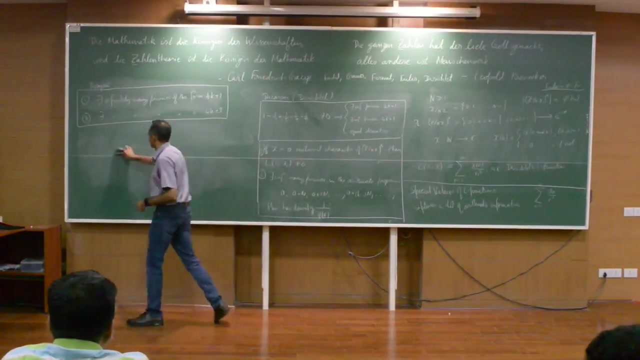 So with that statement, I think I'll just stop Ask me questions. Yeah, so maybe I it is. So maybe let me just work out what happens for n equals four and then you will see this. Take n equals four. So if I look at what are the possible residue classes, 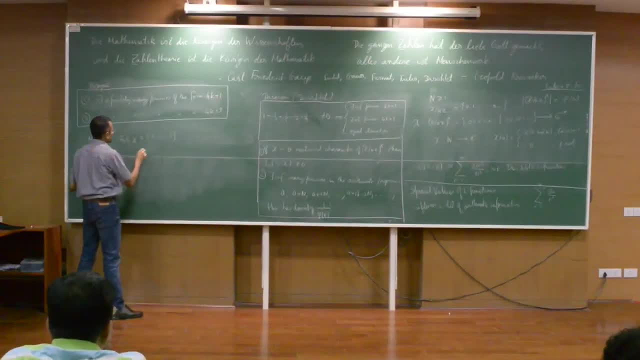 when I divide by four, they're captured by zero: one, two, three. So what are those which are relatively prime? Well, you delete these two. These are the relatively prime to four, And I want a homomorphism from this to complex numbers. 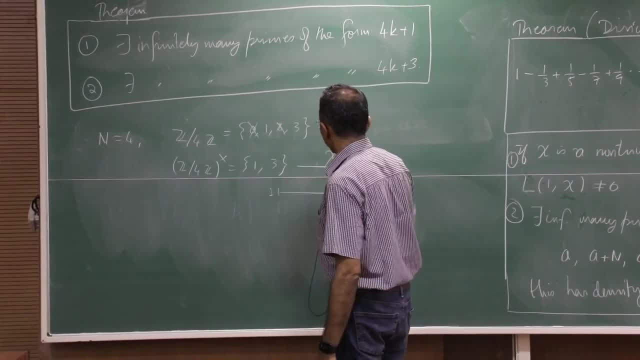 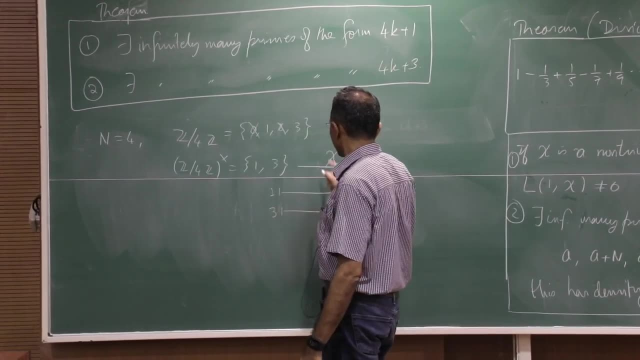 non-zero complex numbers, The only nontrivial homomorphism- these are words I don't know if you know such words- has to send one to two, It has to send one to one and will necessarily to be non-trivial. 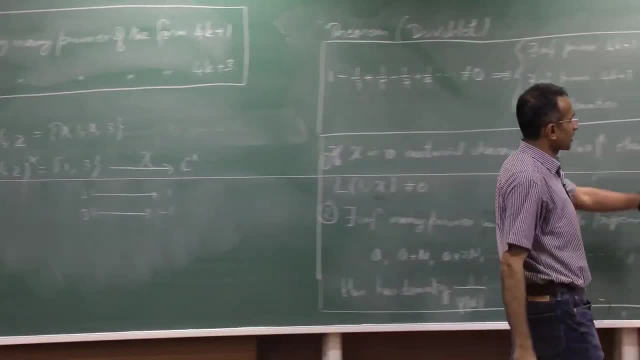 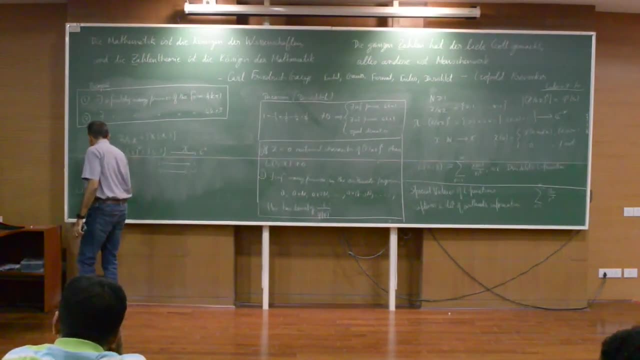 it has to send three to minus one. And then, if I apply this recipe and construct this function, so what does this function look like? ls chi, Well, chi, one by one to the s, that's just one. The next term is chi two by two to the s, but two is not there. 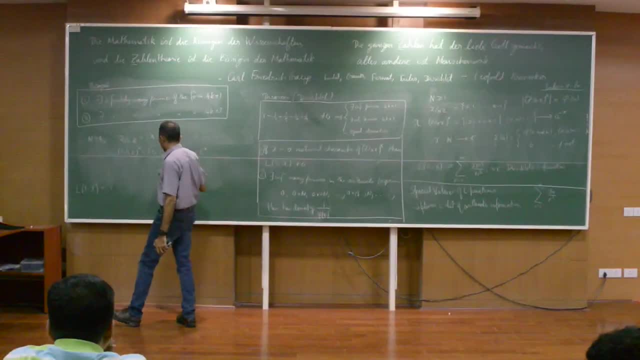 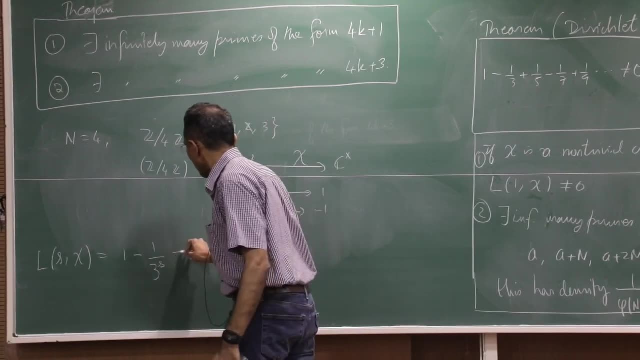 I just that's zero. Chi of three by three to the s three is mapped to minus one, So this becomes minus one One by three to the s. Chi four again is zero. Chi five- five is like one model of four. 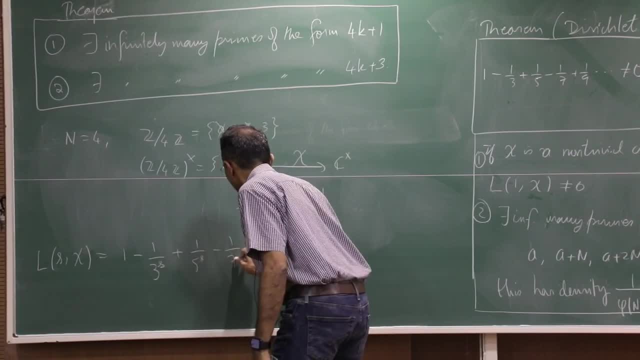 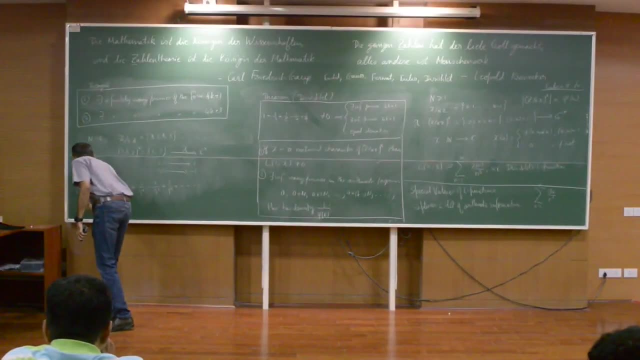 So that's one by five to the s, and you see the pattern, Minus one by seven to the s, plus one by nine to the s, and so on. So for this particular chi, l one, chi is pi by four. 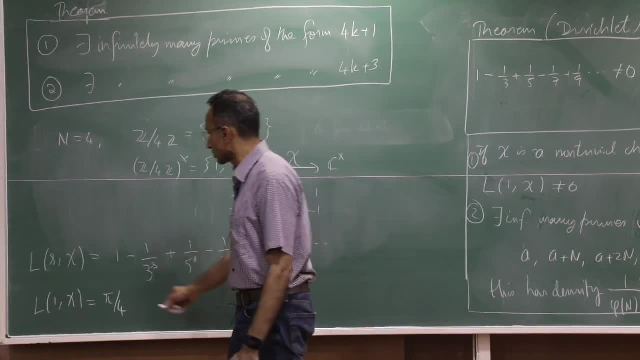 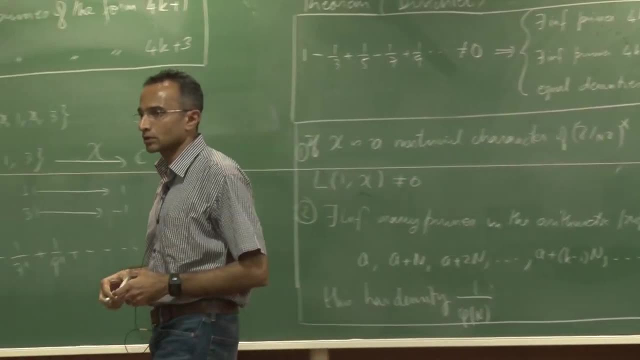 If I put s equals one, the series becomes a Madhava Leibniz series. So this is a special value, so that this guy is a special value of a certain Dirichlet L4. That function, Of course. the real meat is here. 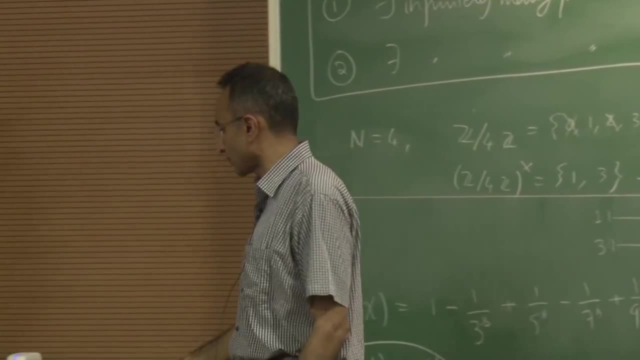 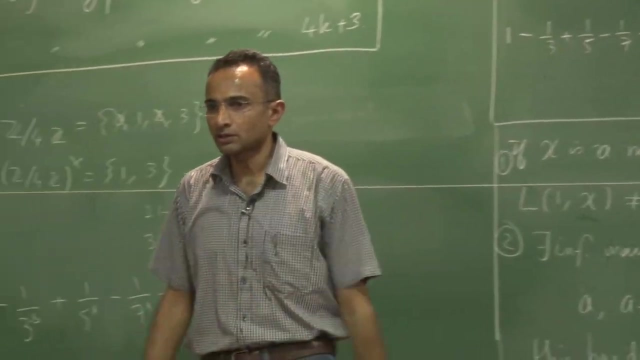 This is magical. What is this series got to do with the structure of primes or the form four k? so that's where I mean it's impossible to do that in one lecture. This is like a one semester course to understand this. Yeah. 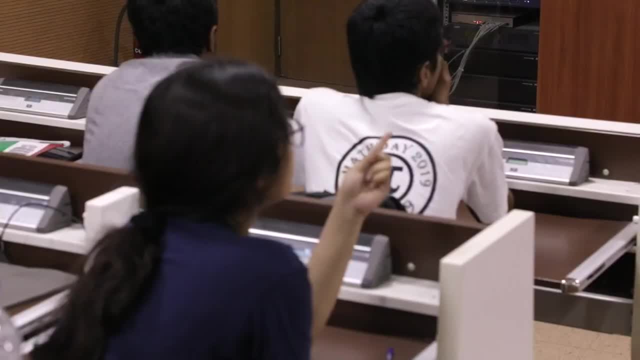 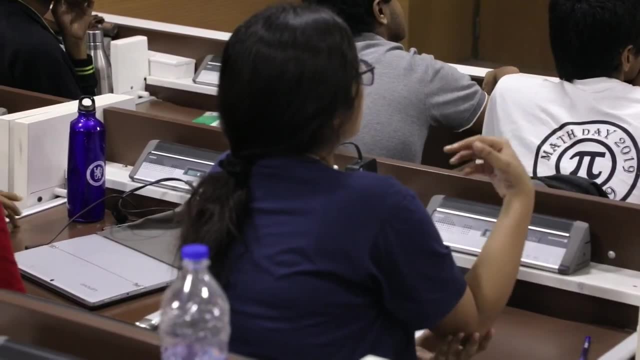 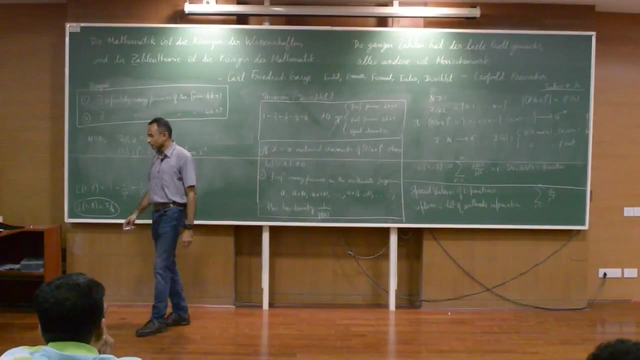 Yes, Yes, Yeah, actually. so in the proof of Dirichlet's theorem you will need all the non-trivial case. For all of them, the value at one should be non-zero. So it's some of the package. 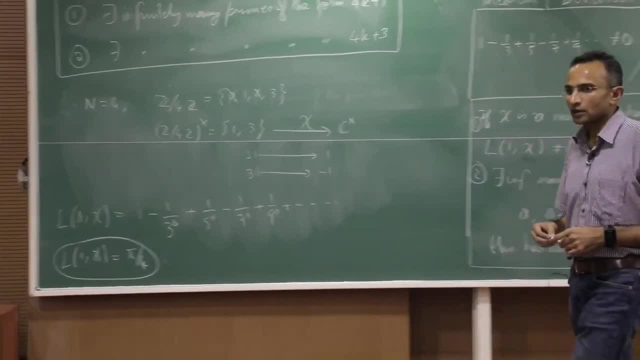 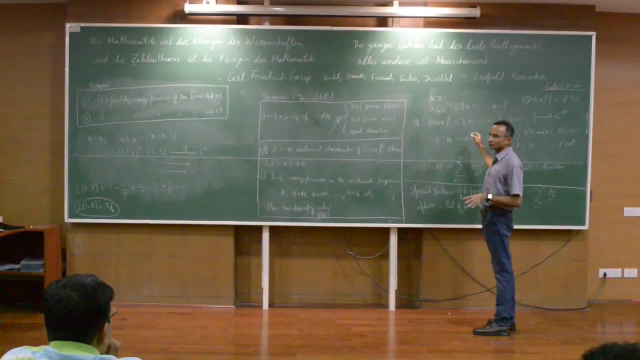 of that entire information is necessary, not just for one of them. So if I take- I don't know So you're in which year? Third year, You've done some group theory. This is a finite abelian group. I'm looking at all homomorphisms of. 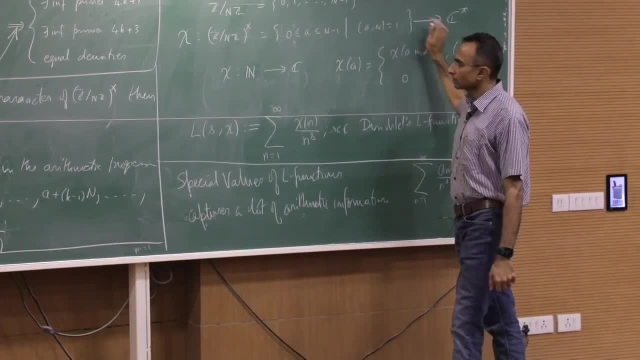 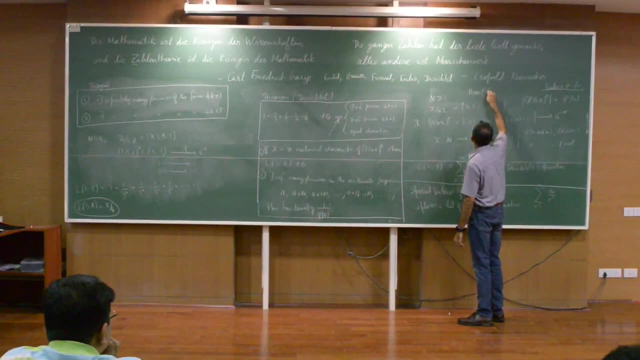 this finite abelian group with C cross exercise. This is the set of homomorphisms. So take any finite abelian group. This is isomorphic to A. It's a bad isomorphism but nevertheless there's an isomorphism. 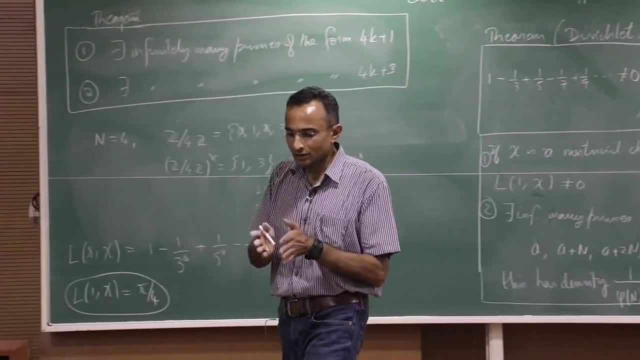 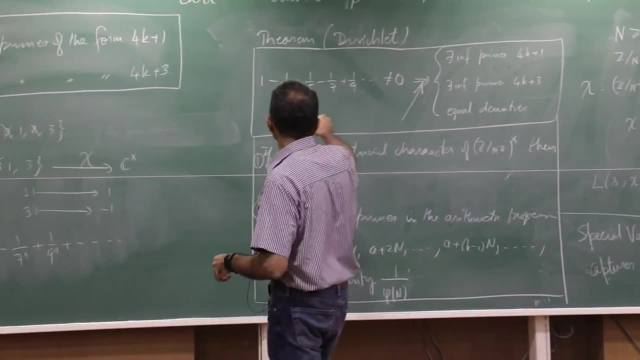 So there are as many non-trivial characters as the cardinality of A minus one. The identity is okay, So there can be many such and you want to prove. this is to be known for all of them. This is to be known for all of them. 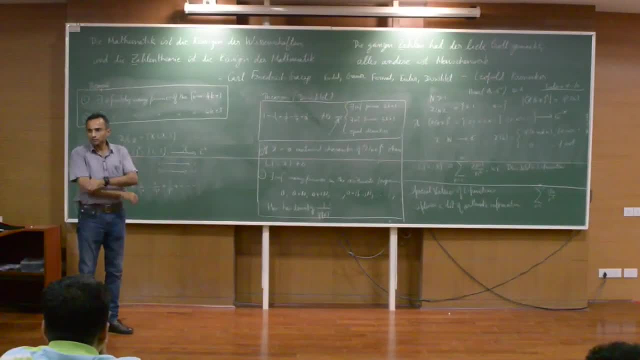 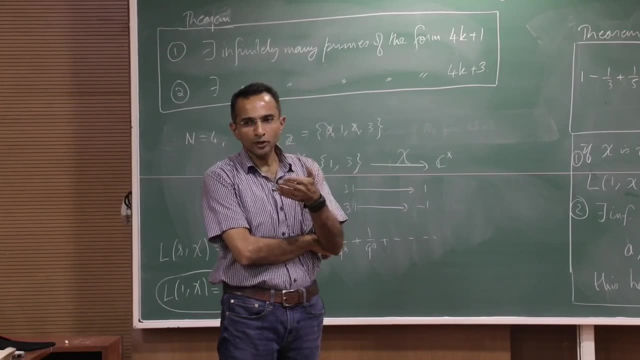 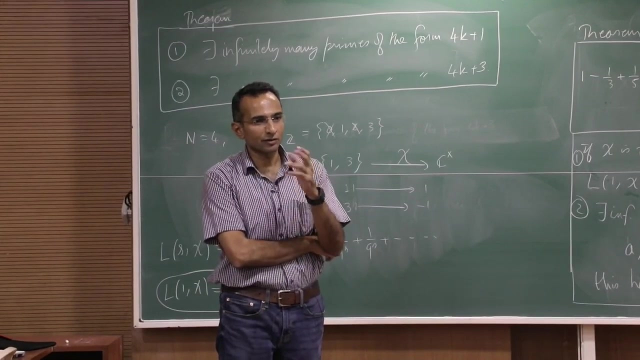 Look up Sayre's course in arithmetic, or Ireland and Rosen. whichever Sayre is very slick. Sayre's writings in mathematics is considered the ultimate in the art of Precy writing. Now I know this whole business of Precy writing is lost upon the current generation. 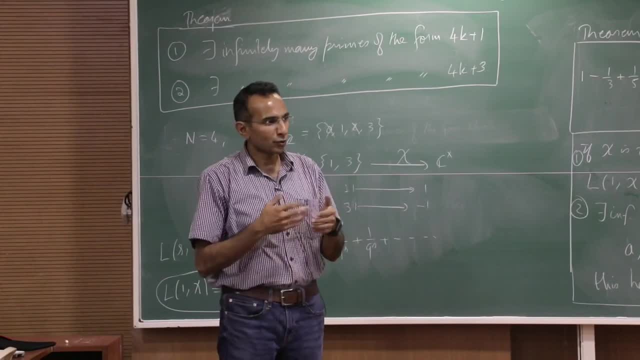 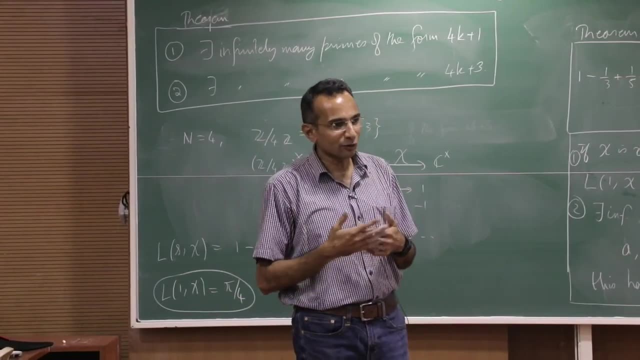 It was already getting lost upon my when I was a student, and now some of your. do you even know what is Precy writing? Yeah, look, that's the. and in the art of writing, mathematics, you know you have to exercise this. 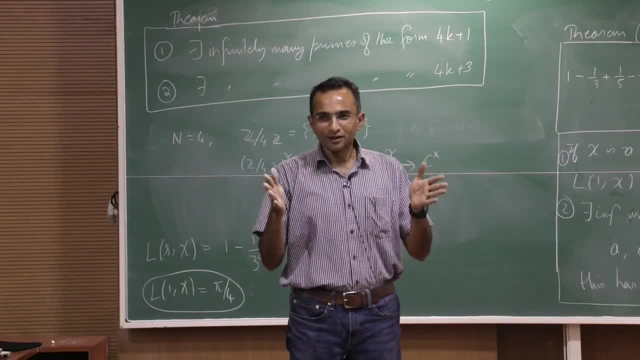 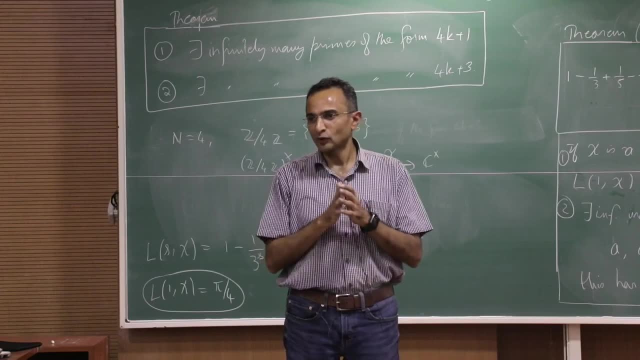 So what is Precy writing? You have some passage. You want to keep all the essence of that passage, all the content, but kind of cut out all the noise. okay, Cut out all the unnecessary adjectives, and you know, Anyway. so you have to. 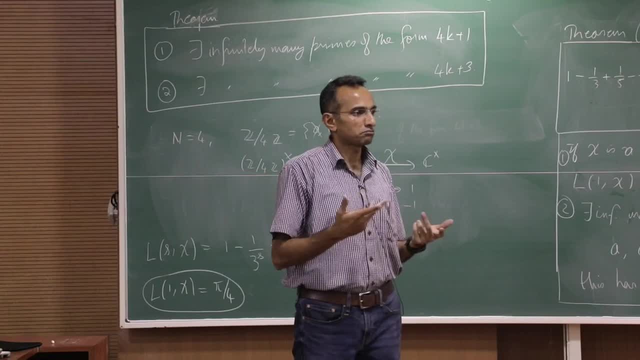 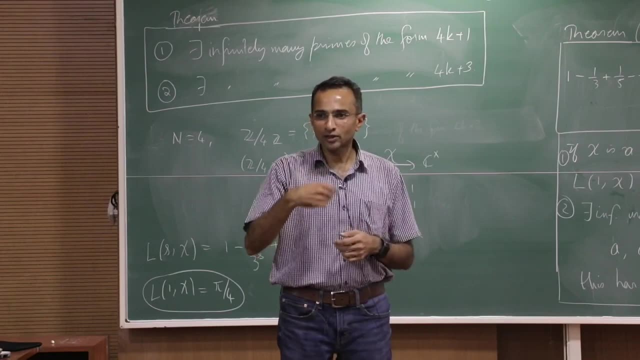 you might have a hundred word passage which you need to cut down to 25 words. Okay, And when you write? finally, the hope is, you know you all go on to become great scientists and mathematicians and you'll be writing. 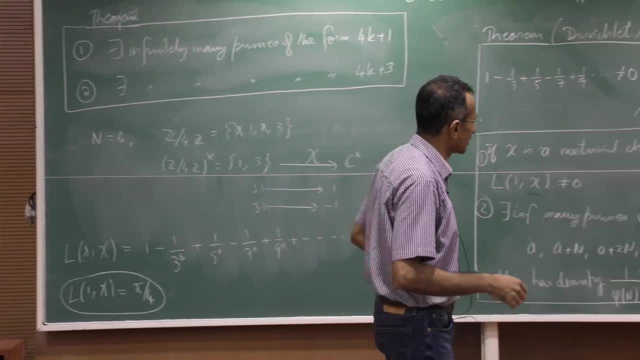 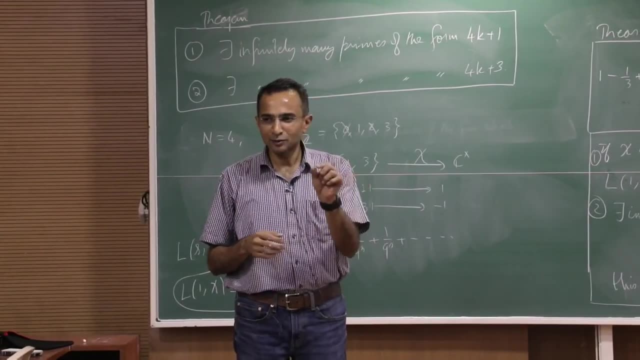 And this is you will need to do this. Sayre, his book course in arithmetic is just- you know, I don't know. 70 pages, 80 pages, Some it's really thin, but there is a lot of mathematics embedded there. 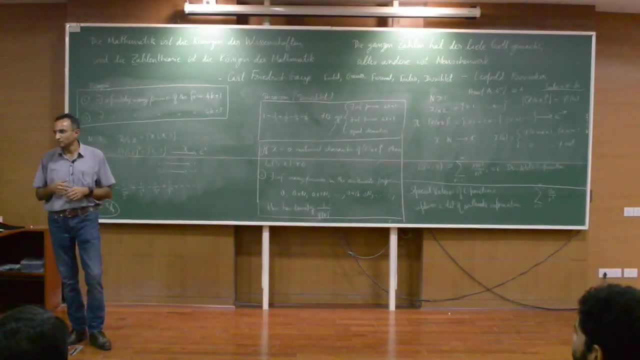 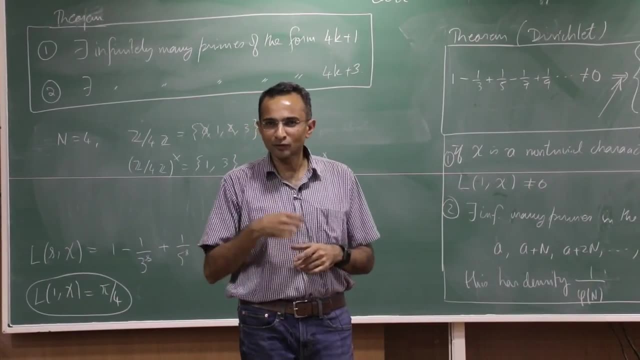 He is considered really one of the great masters in the art of writing mathematics. Those of you who are interested, you can email me. I'll just send you something in the way of writing mathematics. There was a number. here is David Goss at Ohio State. 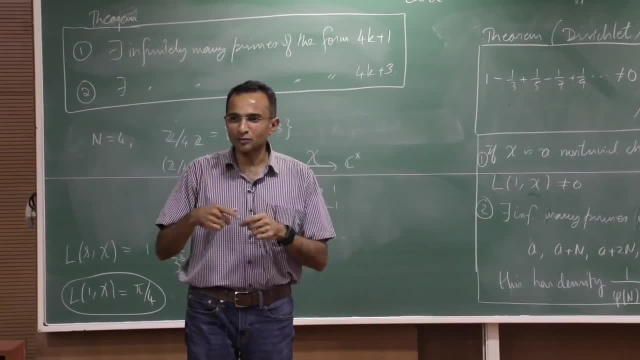 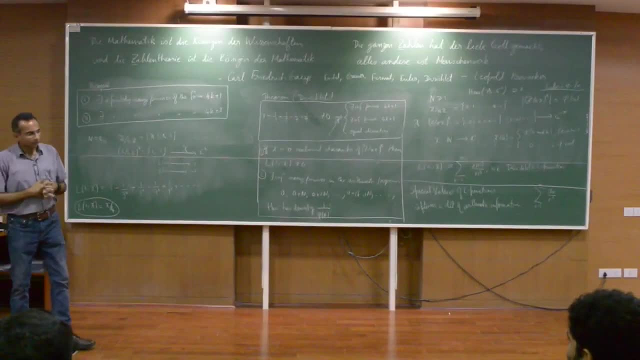 He recently passed away So he wrote a four page article on how to write mathematics, various things he's learned from Sayre And you can learn many things from that. That was an extended thing to say. that I learned in Rosen's book is like 200, 300 pages. 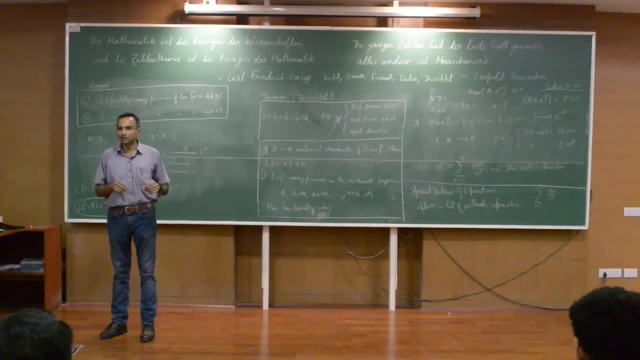 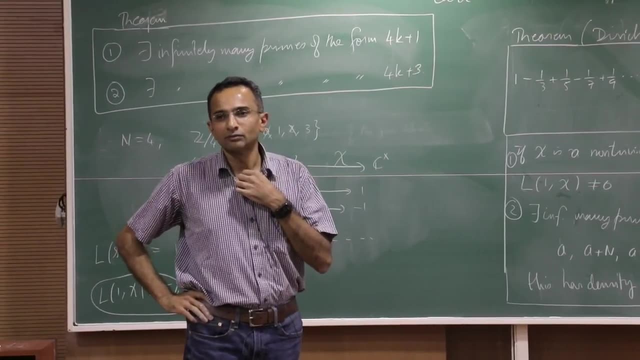 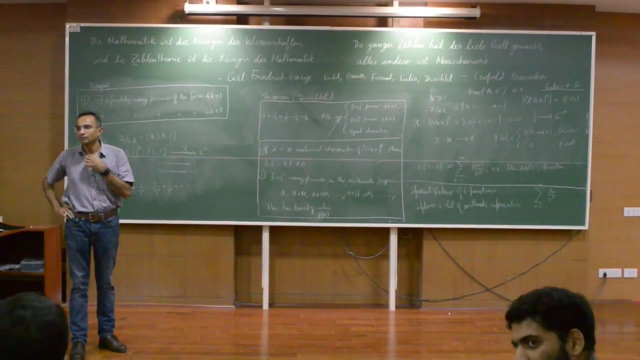 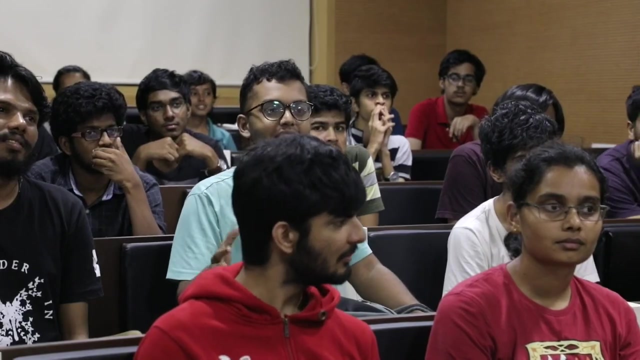 And this theorem comes, I don't know, in the 18th chapter or something like this, but it can be done very slickly also. Yeah, That's obvious. Yeah, why, Why is it obvious? They all have to be odd numbers. 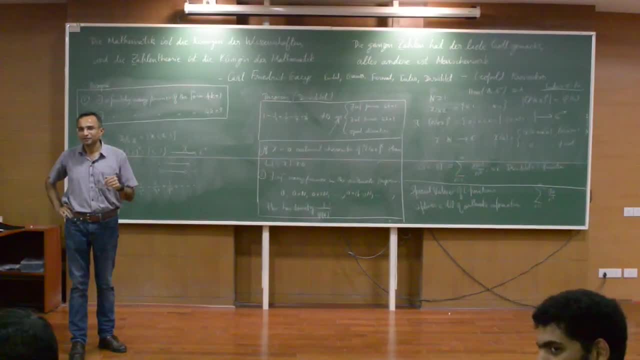 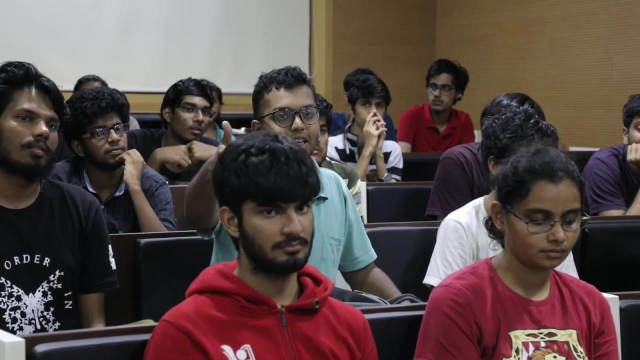 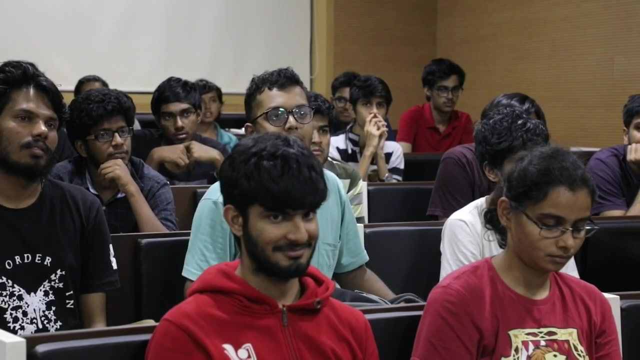 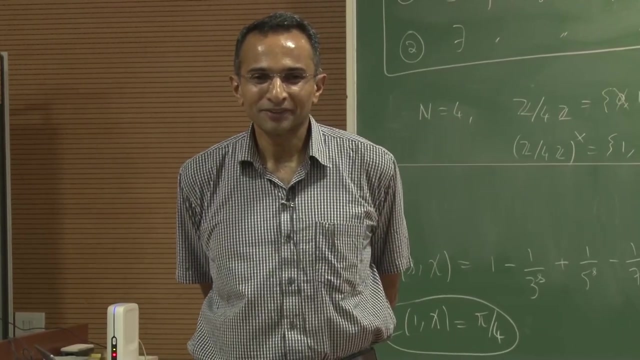 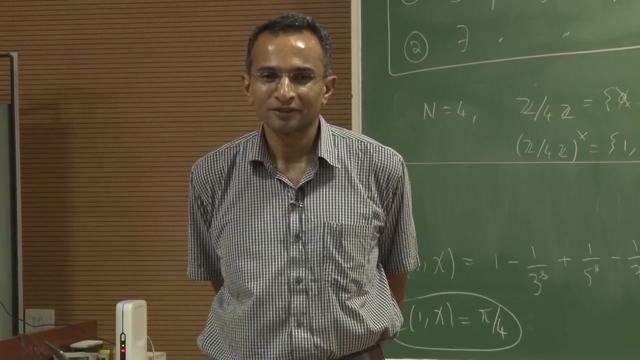 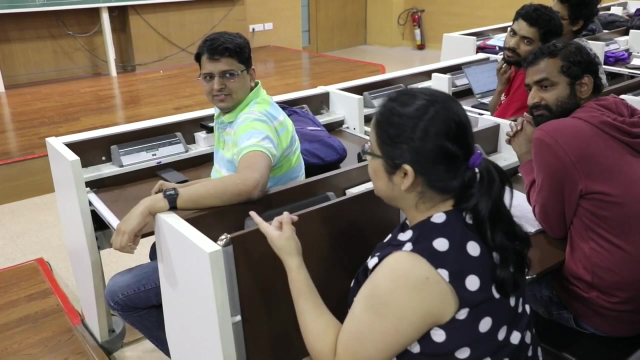 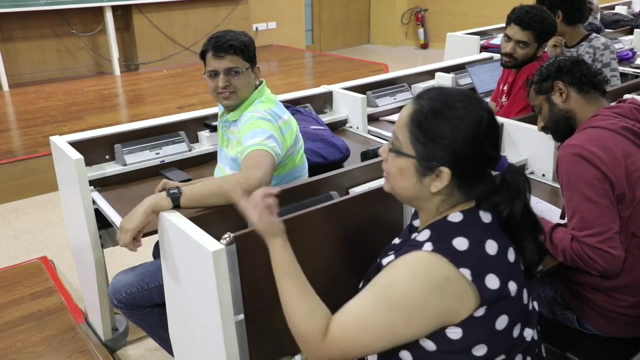 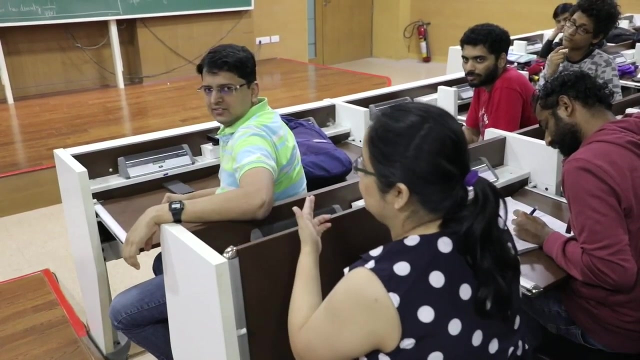 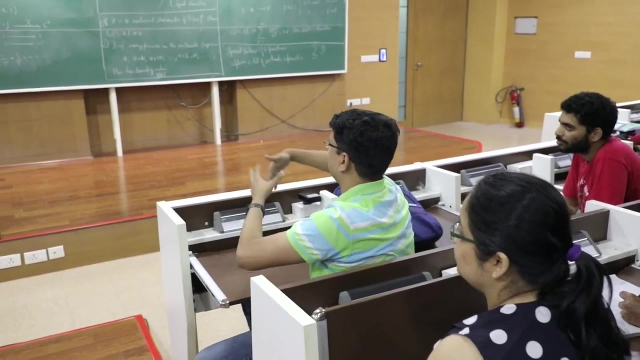 So it cannot end with zero, two, four, six, eight. I will leave my colleagues. Yeah, What does the theorem say? I see, Okay. Yeah, I see, Yeah, I mean, this is the beauty of number theory. 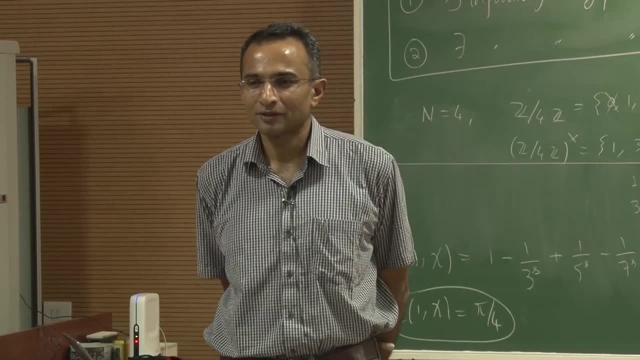 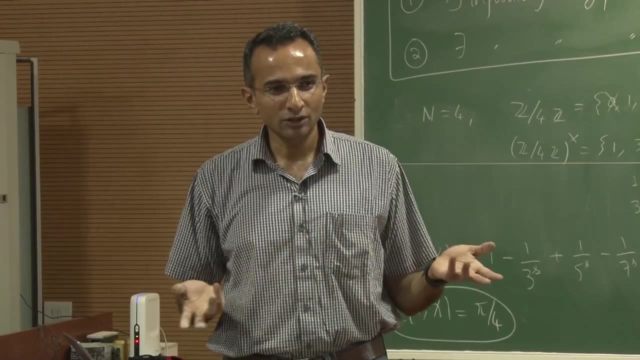 I suppose you can, one, can you know? just the statement makes sense, First of all. so let me just, for the sake of everyone. any prime is other than two. they're all odd, So the last digit has to be one, three, five, seven, nine. 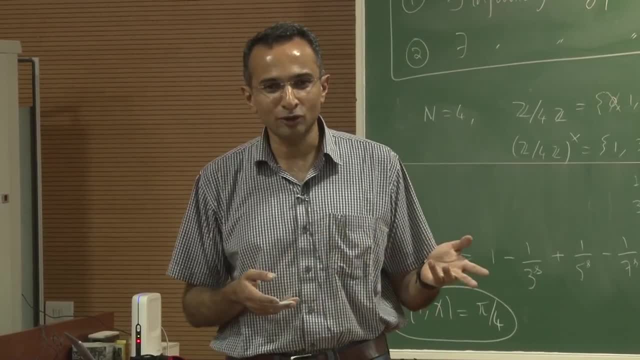 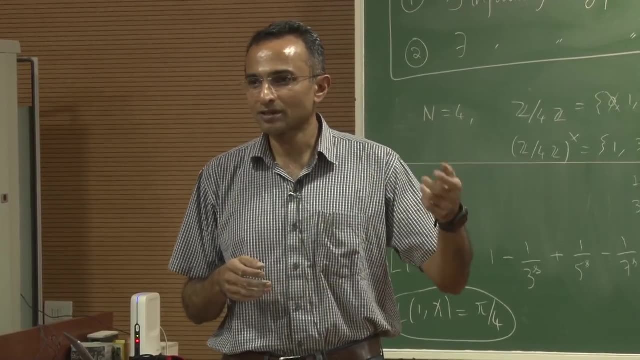 It cannot be five, because then five is going to divide that number. so it's one, three, seven or nine, And then you can start asking probabilistic questions. Set of all primes ending with one. set of all primes ending with three, seven and nine. 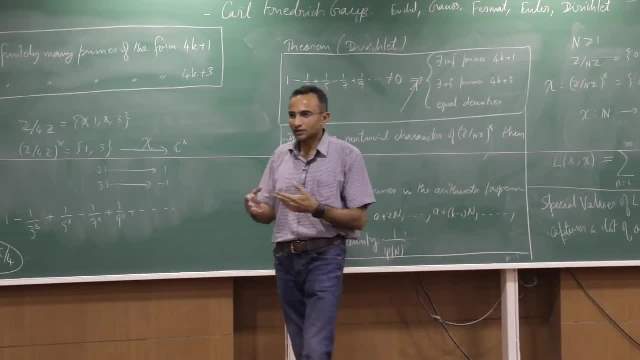 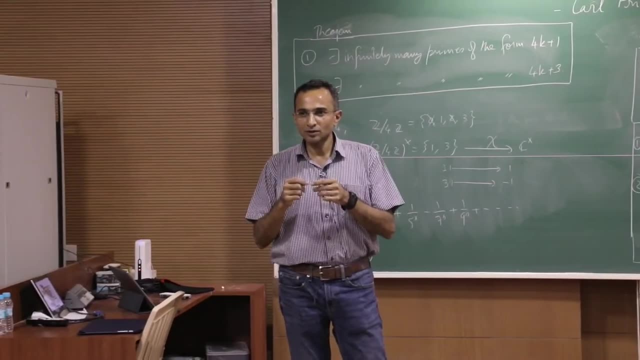 Dirichlet's theorem, applied to capital N being 10, will tell you that these are equidistributed. Now the question here seems to be if some prime is ending with the last digit three, what can you say about the next prime? 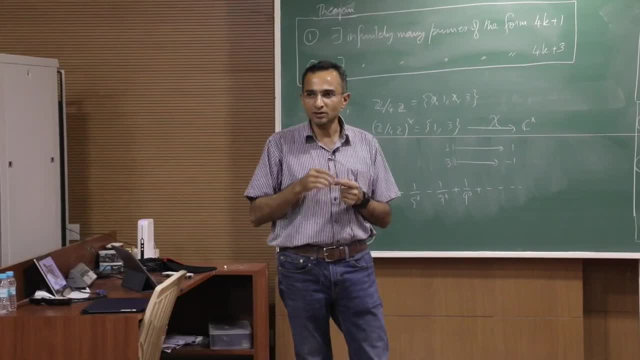 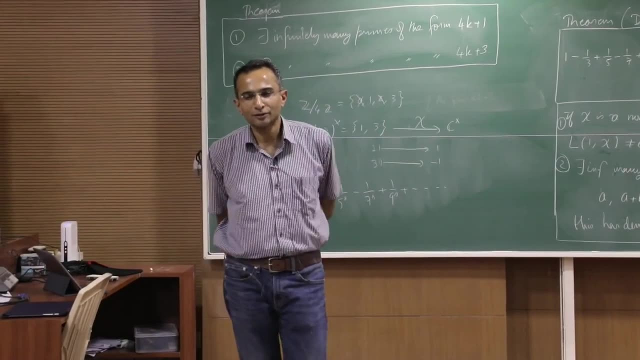 the last digit of the next prime And apparently there is some recent theorem which says with high probability, the last digit of the next prime is something I really don't know. this kind of I mean I'm not up on the literature on this- 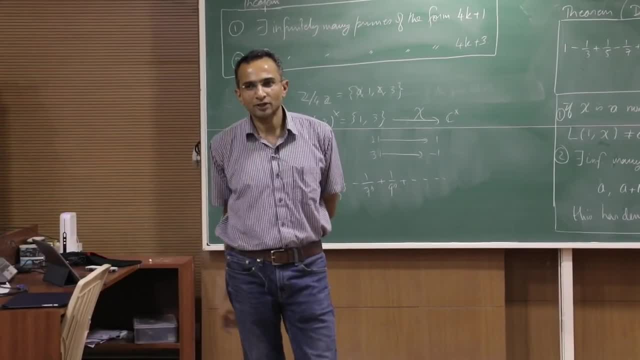 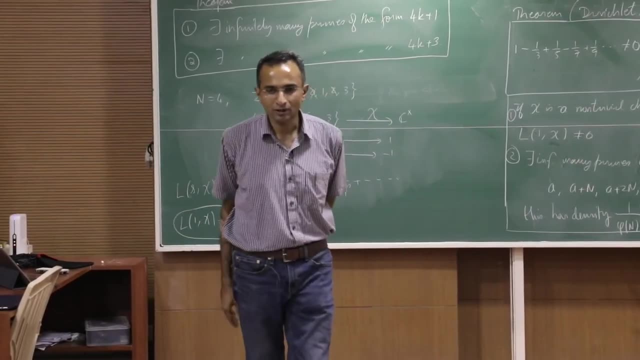 but it's very recent. yeah, I mean the name she mentioned, Andrew Granville and Saundar Rajan. this is Kannan Saundar Rajan. he's at Stanford. As you can guess, he came out of India. 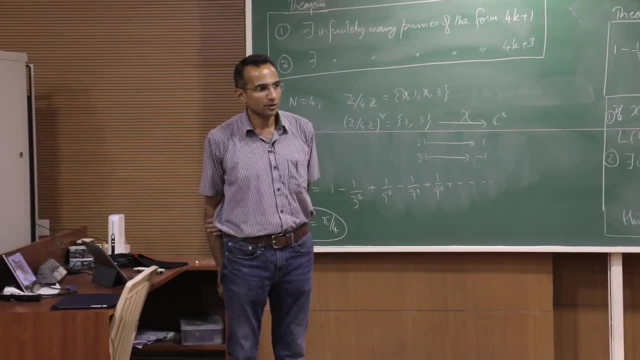 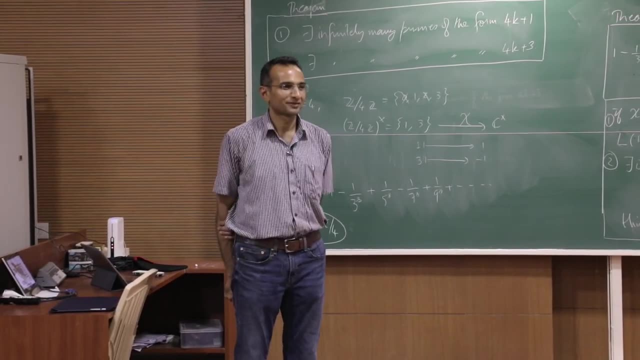 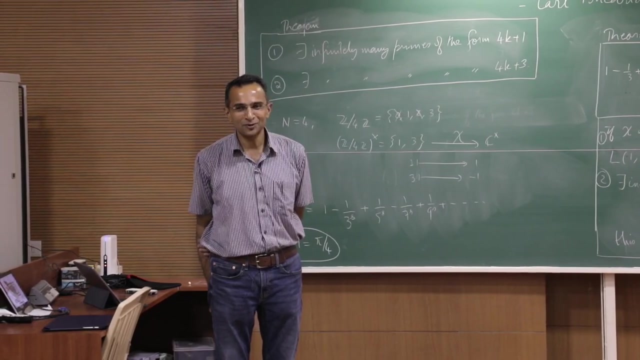 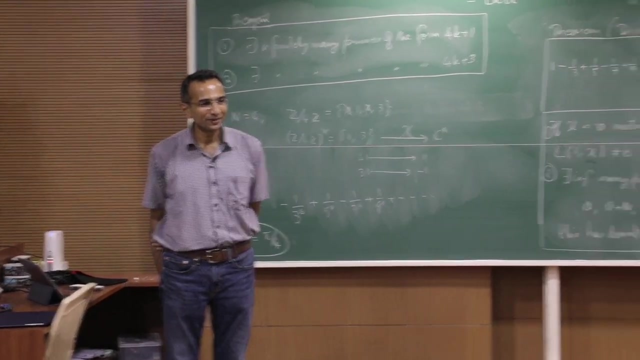 Fantastic analytic number theorist of our times. These are big names in number theory. Any other questions You will ask later You can ask. it's okay, He wants to show off? show off. Yeah, Now you have to. Yes. 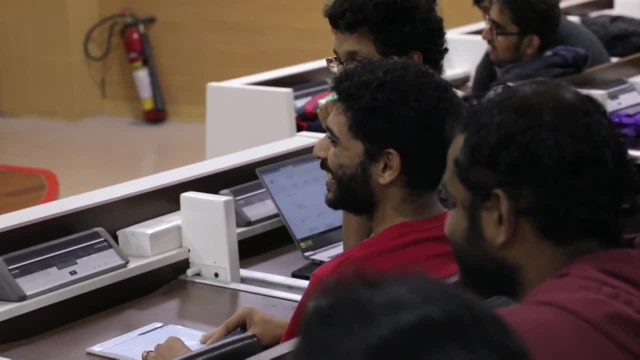 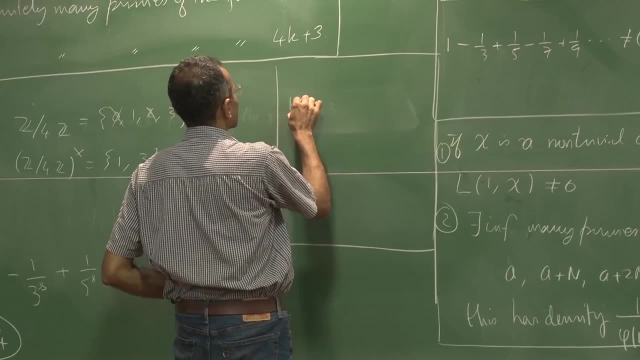 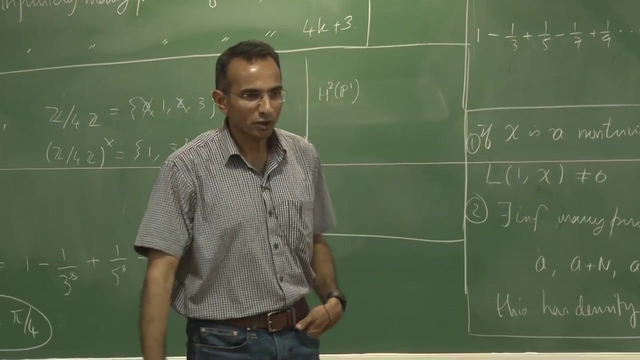 Of course The The simplest example is to look at H two of P one, And the point is, I don't tell you P one or what, And some of that is the motive. So you can think of this as you know. 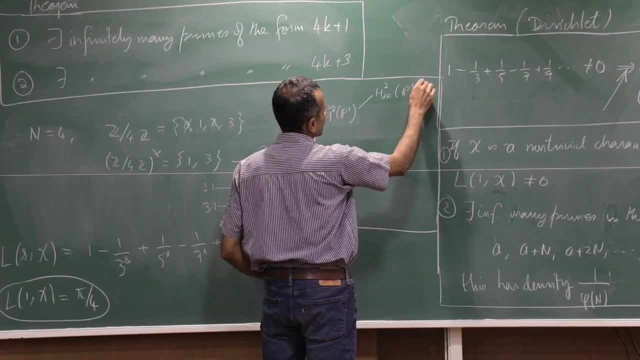 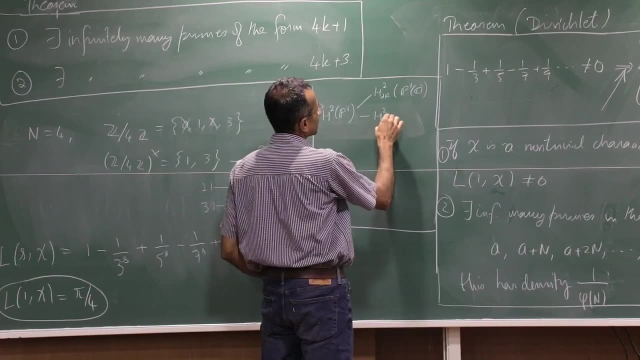 Durham. cohomology of P one over complex numbers. For most of the audience this might be just words, but you might as well hear it, Or I can look at you know, singular Betti. cohomology of P one of C.